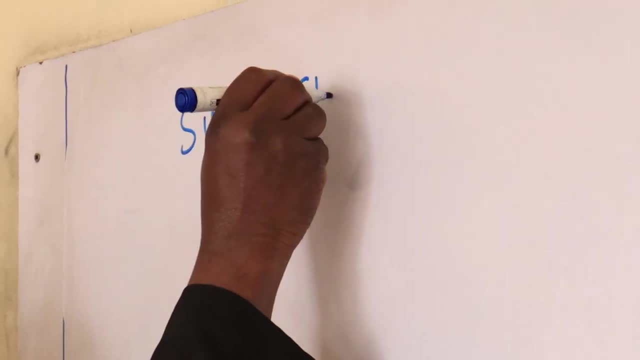 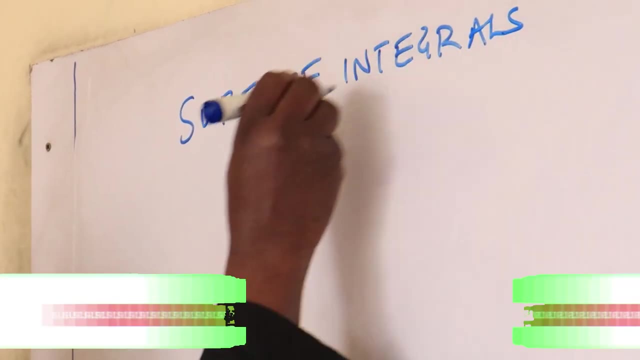 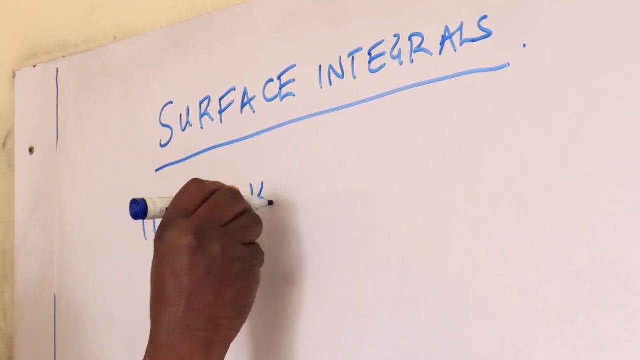 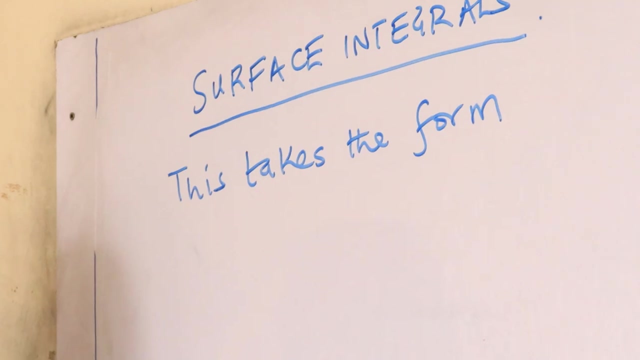 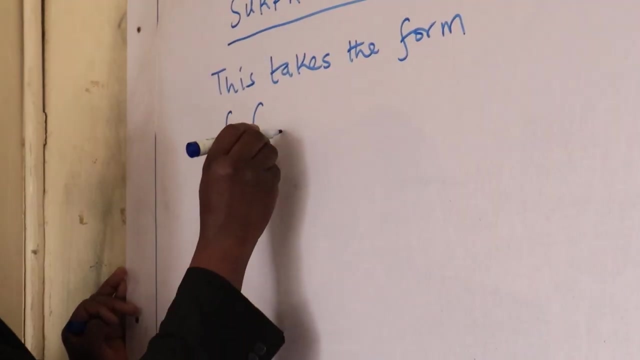 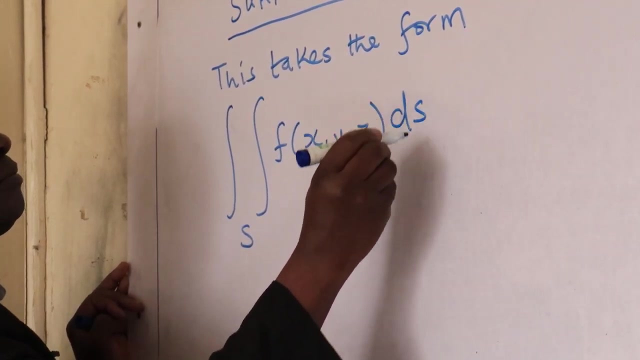 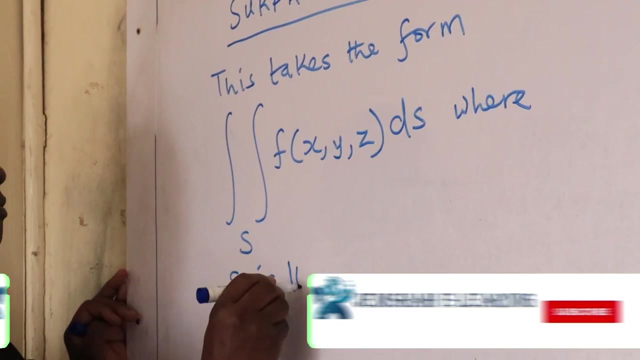 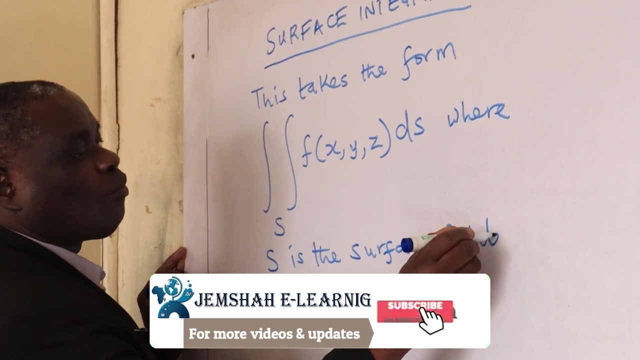 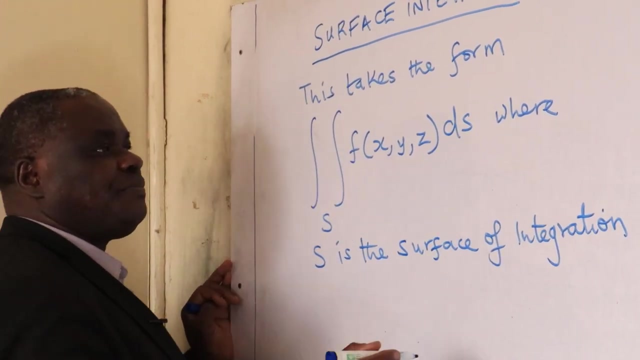 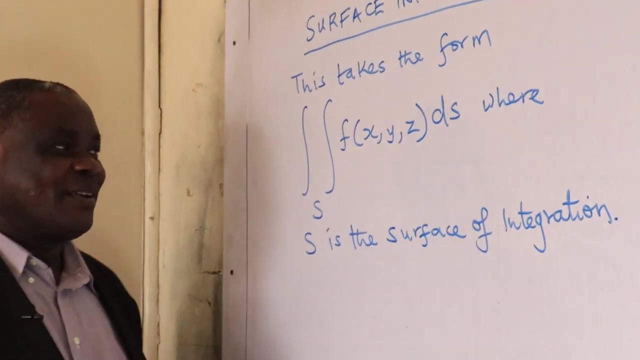 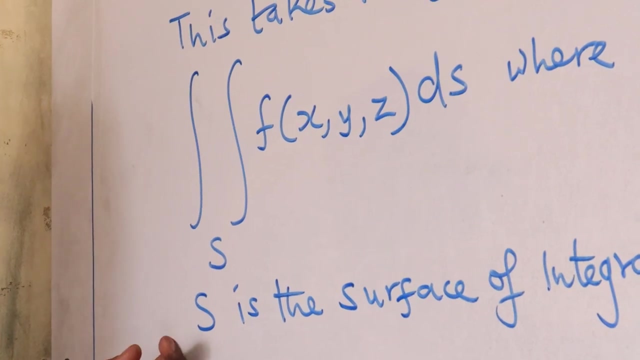 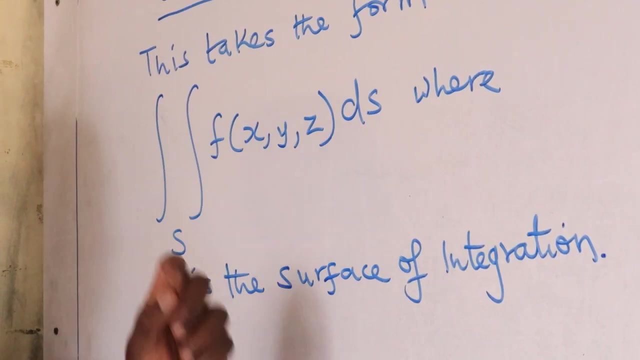 surface integrals. This takes the form, So this takes this format. it is a double integral and we are now integrating over a certain surface. So we say S is the surface of integration. This dS is a small portion of that particular surface. 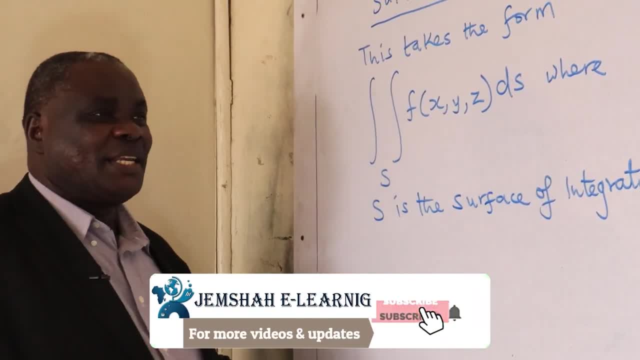 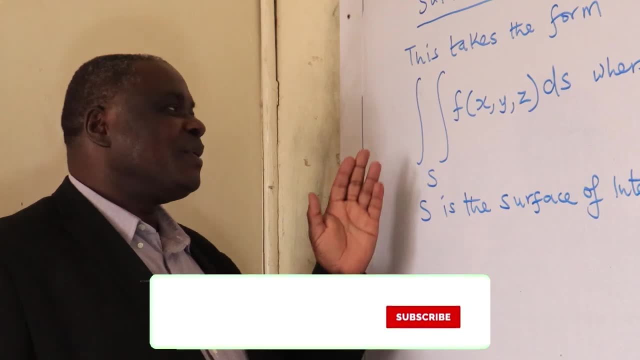 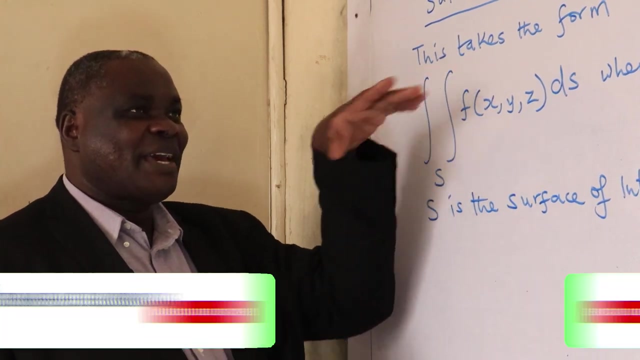 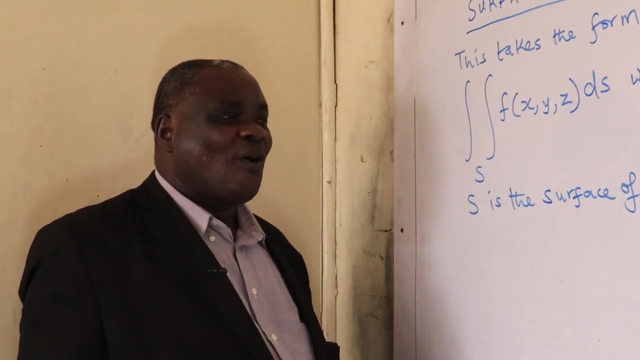 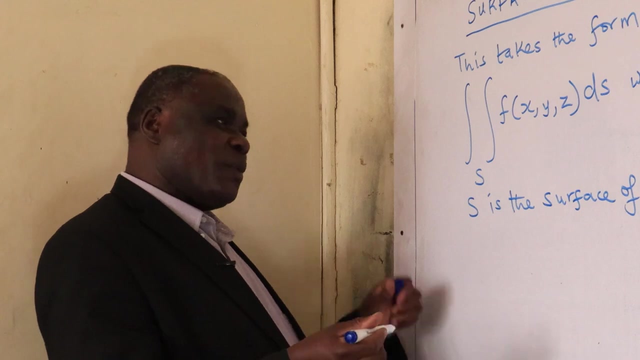 So, since we have dS here, depending on the surface that is concerned, we can be able to integrate this and we can always. if it is a plane which is above xy plane, we can always now project that surface. So, projecting that surface onto xy plane, we say now this dS will change and this particular 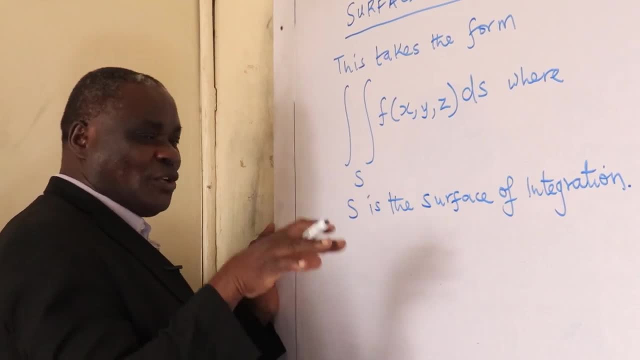 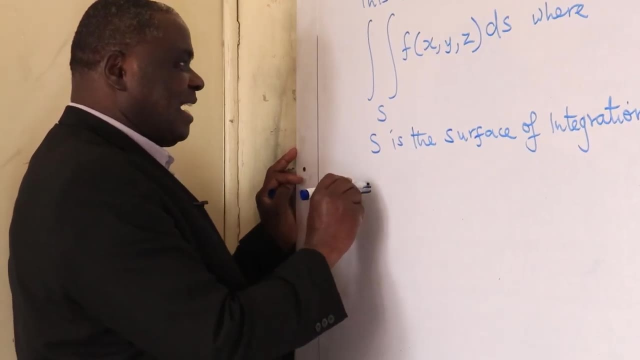 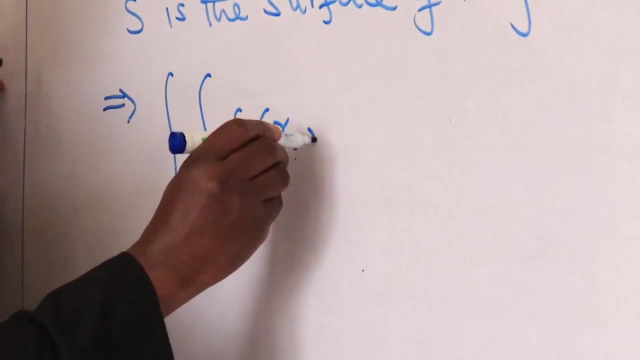 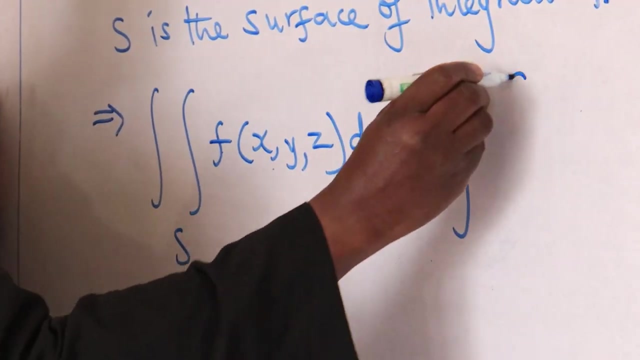 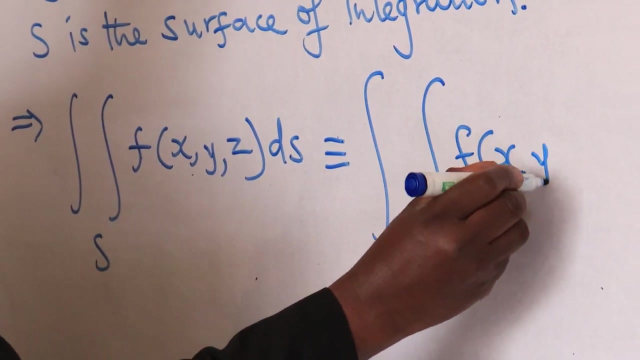 surface of integration. we will have it as a region R because that is the projected region on the xy plane. So this implies the integral S function over xyz, z, ds will be equivalent to a double integral region R. Here we have function of x, y, but 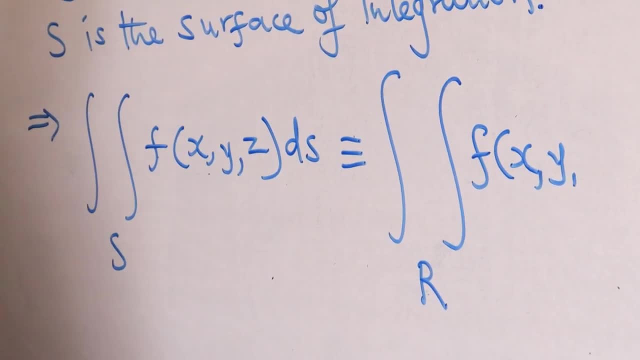 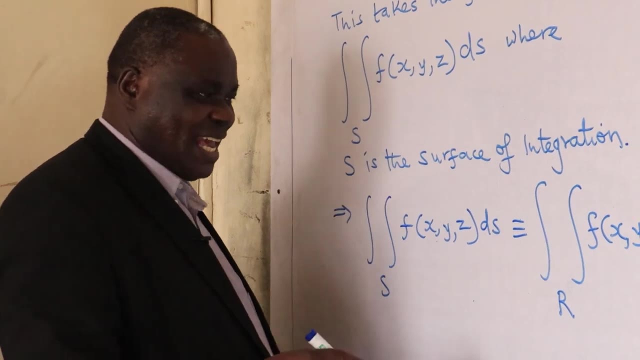 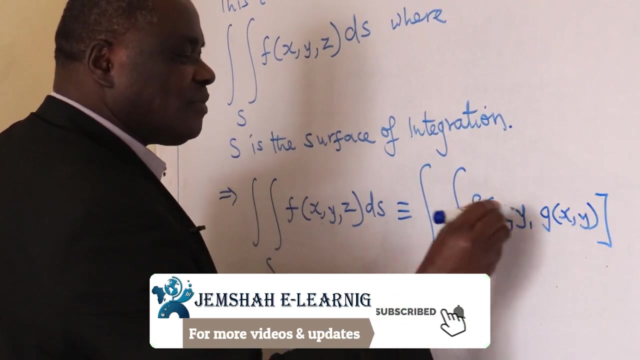 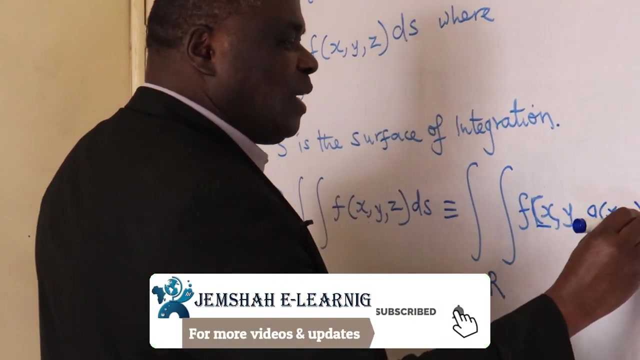 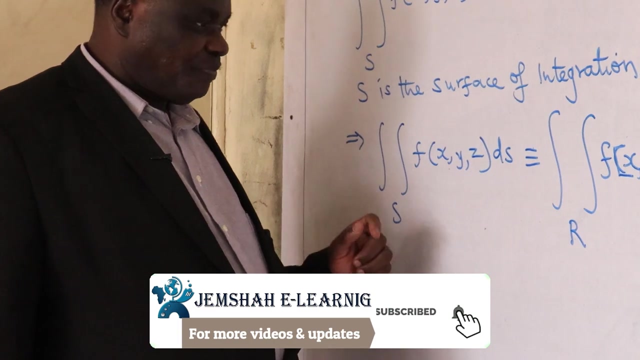 this z we are going to replace it with, because z on that surface can be described in terms of x and y. So we can say g of x and y there. Now our ds now changes into a square root of changes into a square root of. so we've been saying this double integral. when a surface 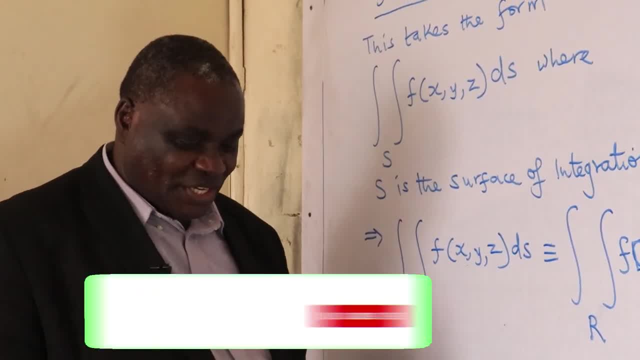 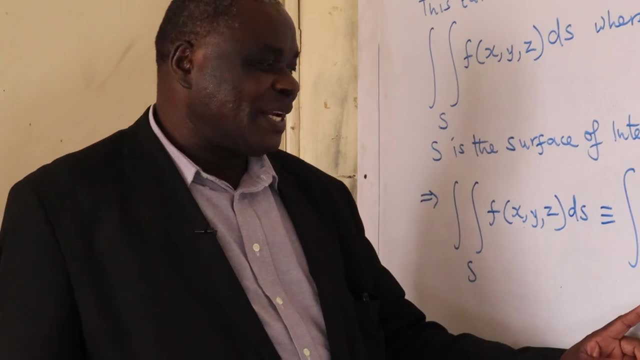 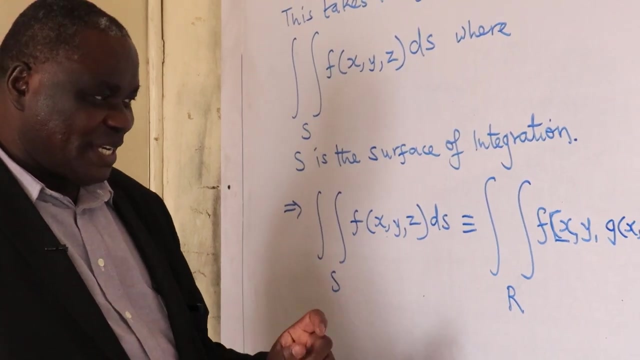 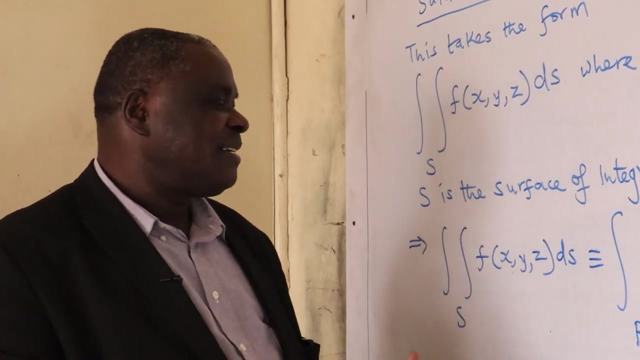 is on top of x- y plane. It can be projected onto our x- y plane so that we use the regional projection as our region for integration, for the double integral. Now, this z, we are going to replace it with the function of x and y Over that surface, over that surface that we have z, it will. 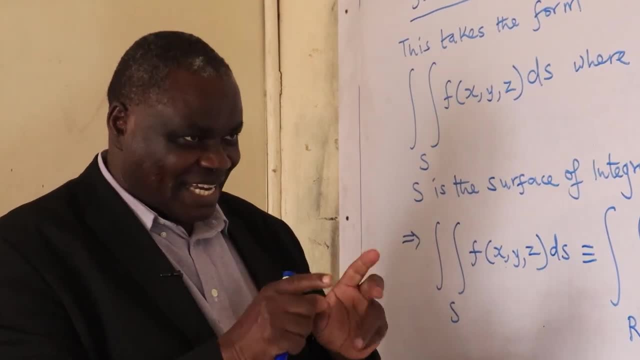 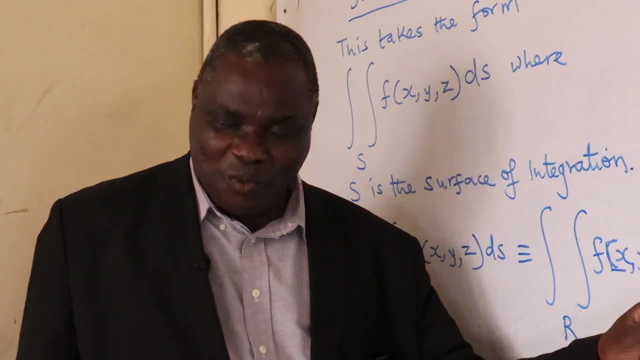 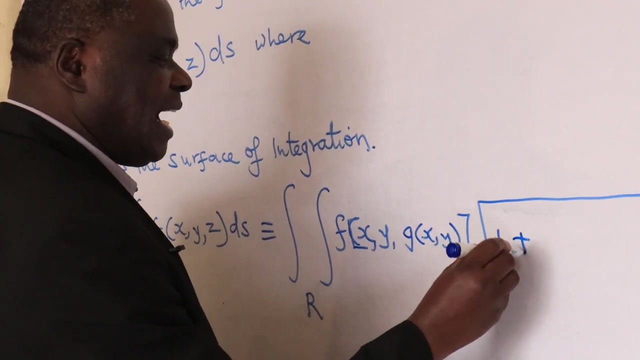 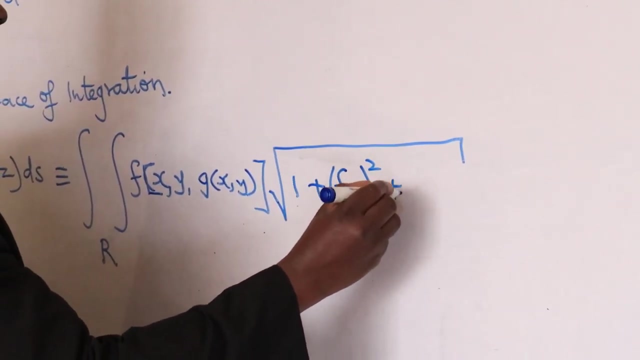 be an equation containing z in it, And we have z in it, so we make z the subject. z will now be a function of x and y. Now the ds will be equivalent to square root of 1 plus 1 plus fx, squared plus f. subscript y. 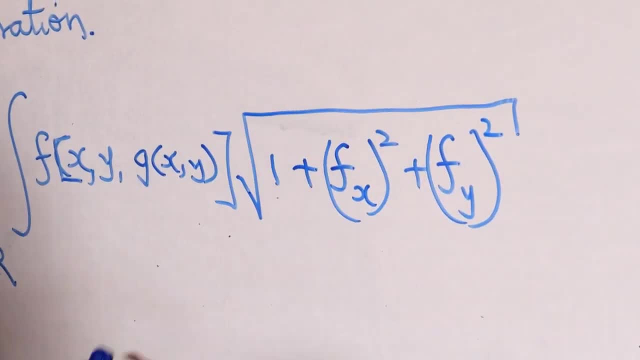 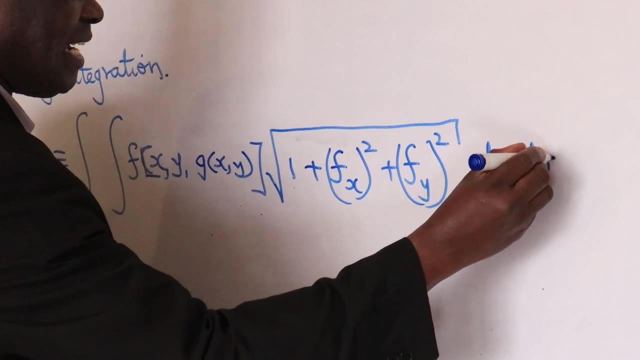 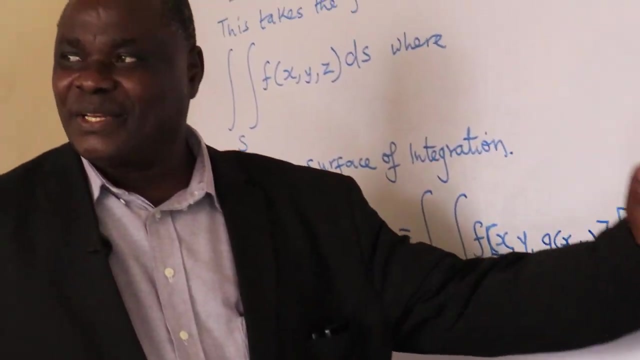 squared, Then we go for square root And then now, because region is on our x, y plane, we integrate it with respect to y And then a x, Or we can use dx dy, Whichever. now we can use dx dy or dy dx. 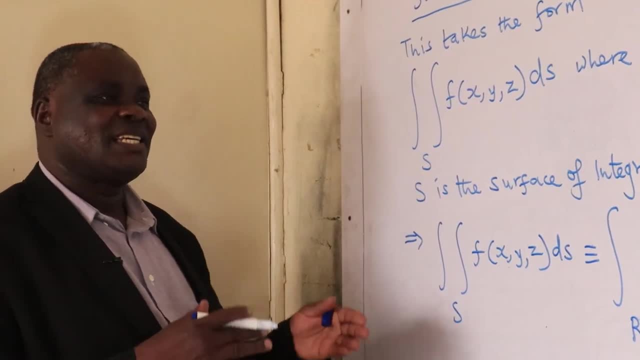 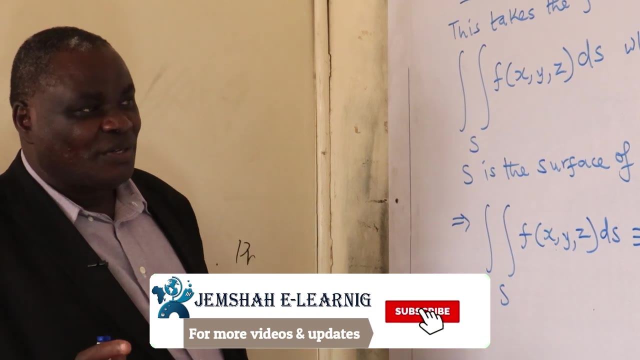 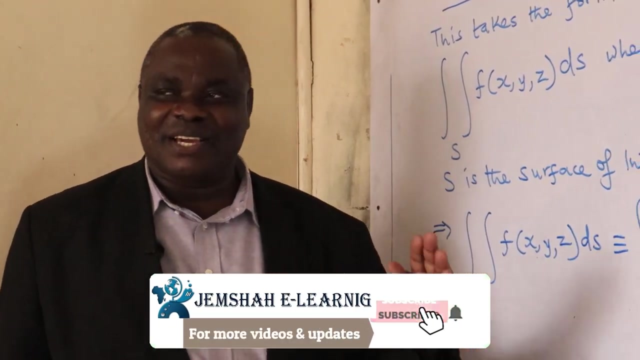 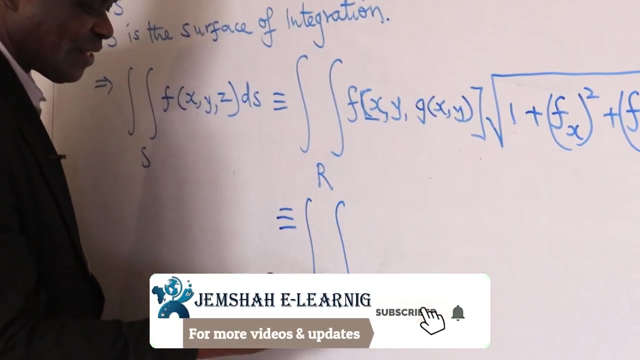 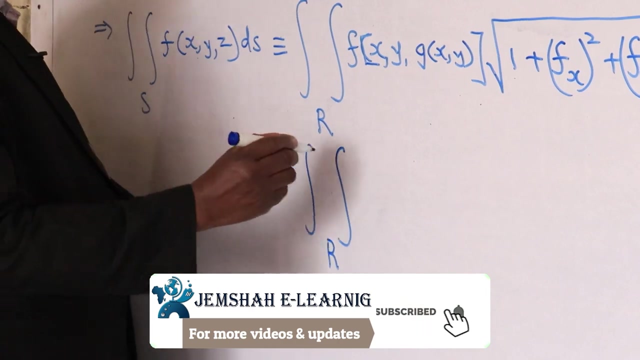 So that's how we are going to evaluate our double, our surface integrals. But also there is something, There is another way of running writing ds in vectorial form. we can also say: this is equivalent to: we are projecting the plane on xy, we are projecting our surface on xy plane. so this will just be a function. 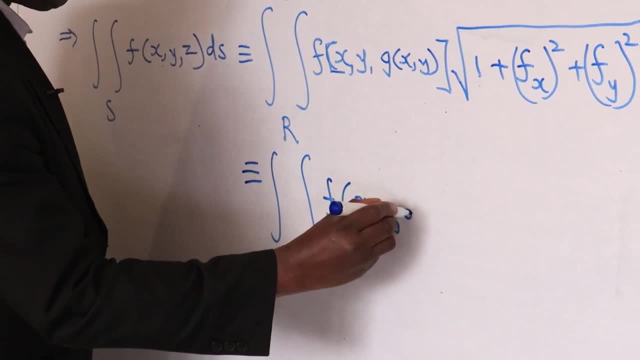 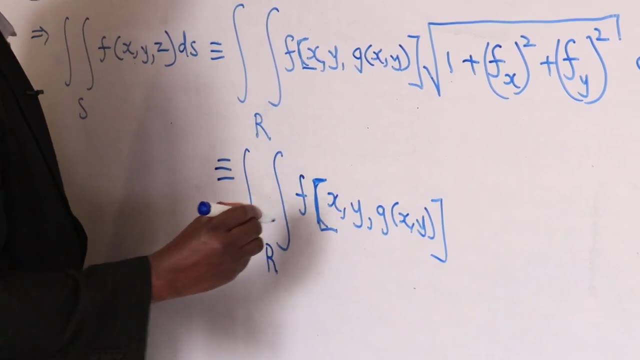 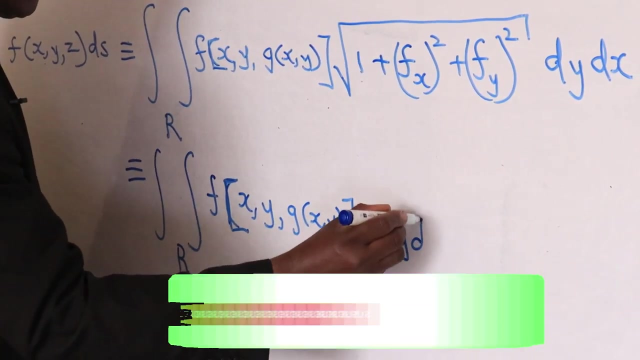 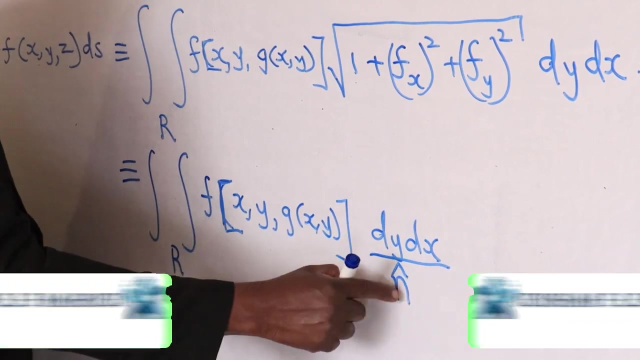 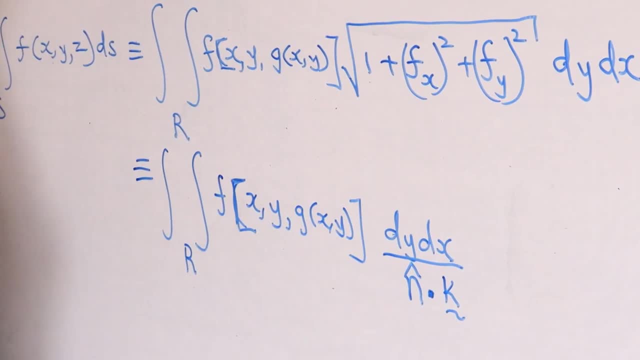 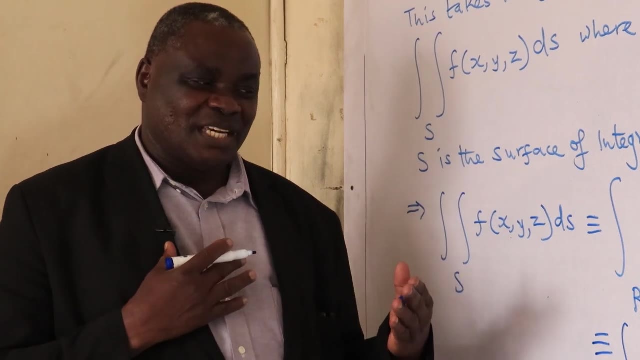 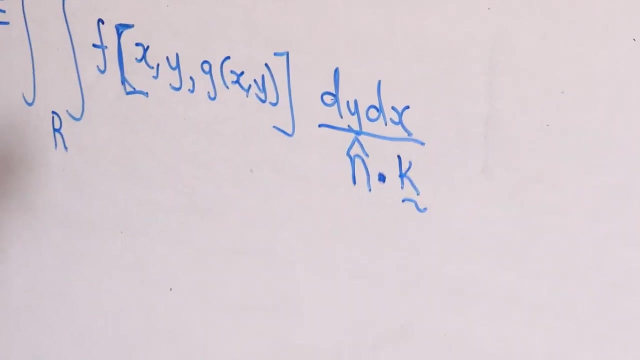 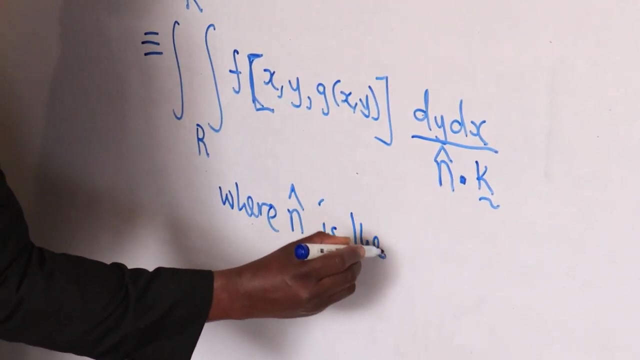 dotting k, vector k, because we are projected on xy plane. It depends on the plane that projection is required. If it is on xy plane, then it will be n dot k where n, where n is there? Unit normal vector. unit normal vector. 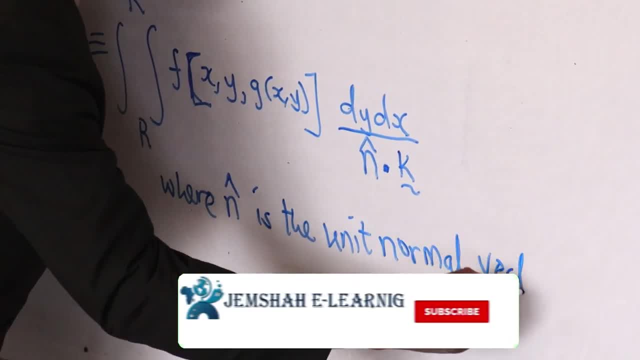 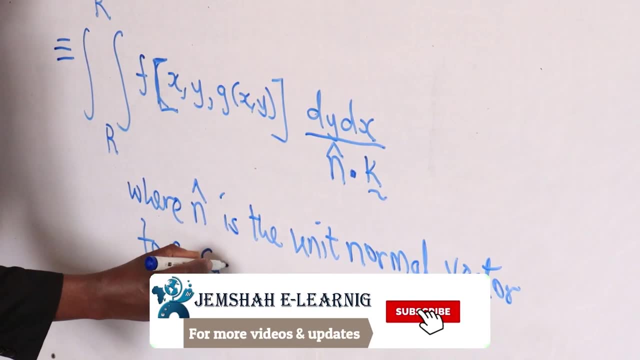 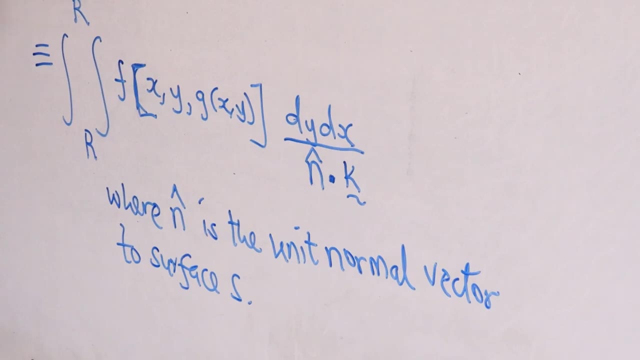 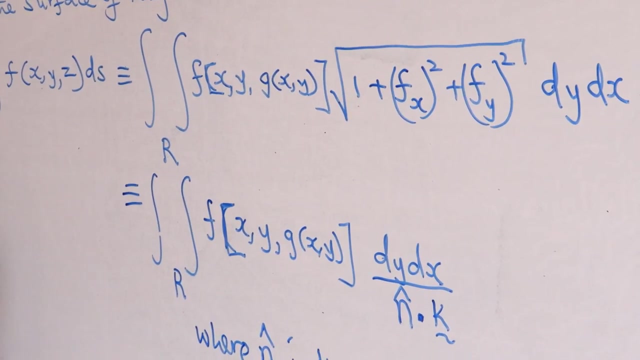 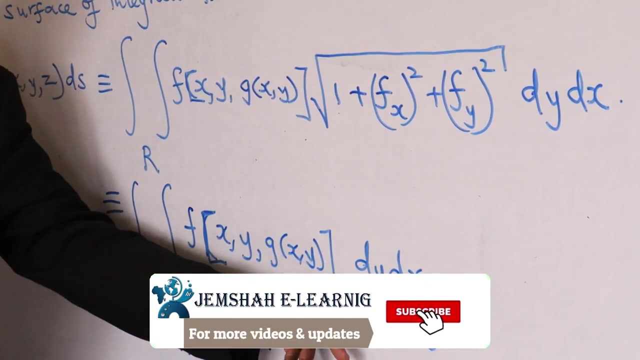 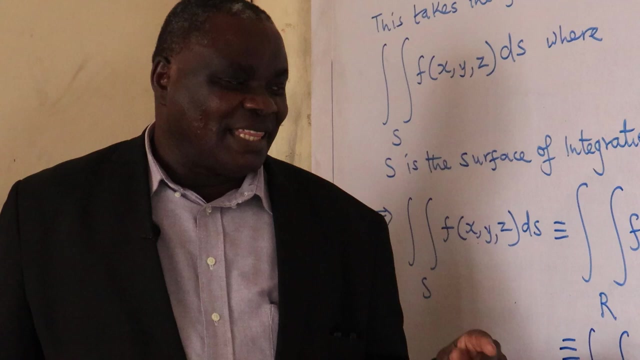 This unit normal vector to surface to surface s. So this is another way of we can use this or that, whichever comes first, Whichever looks simpler. we can be able to use this, too, for our operation If the region is projected on yz plane. if the region is projected on yz plane, then 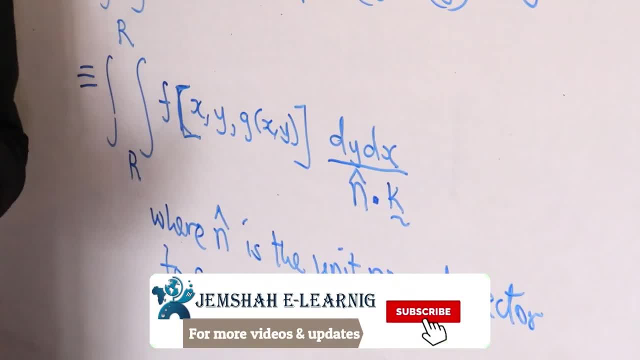 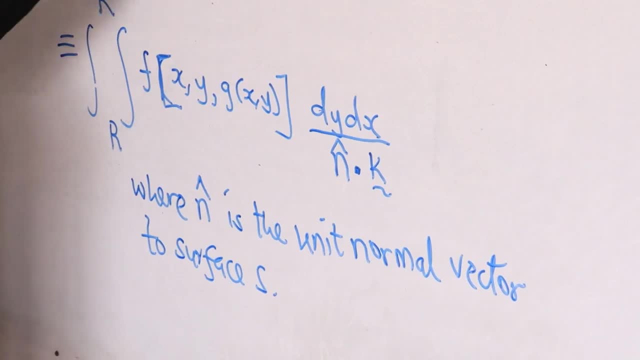 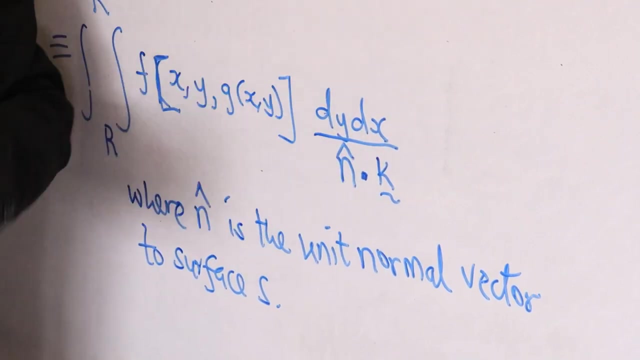 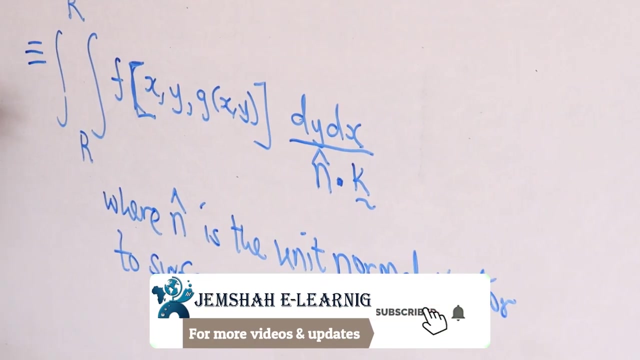 we will be having here n dot i. If the region, if the surface is projected on xz plane, then we are. we are going to have here n dot j, n dot j. But most, most of the surfaces, we normally project them on xy plane because working. 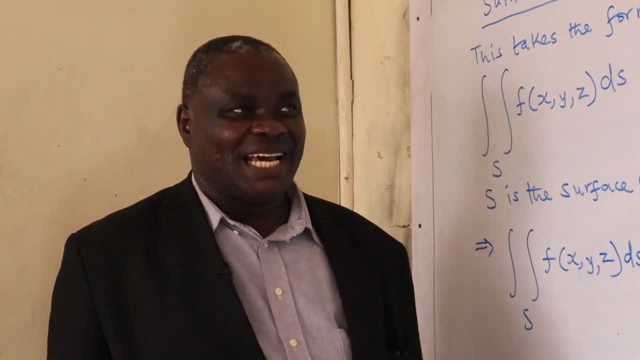 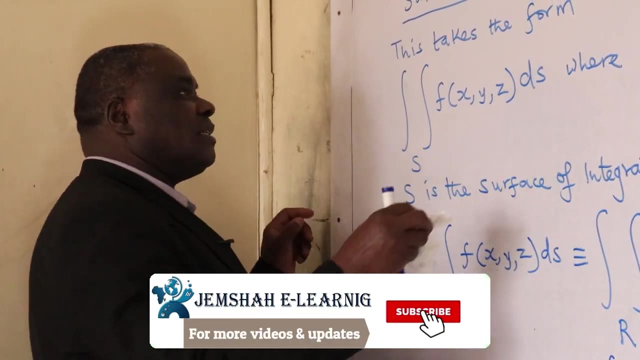 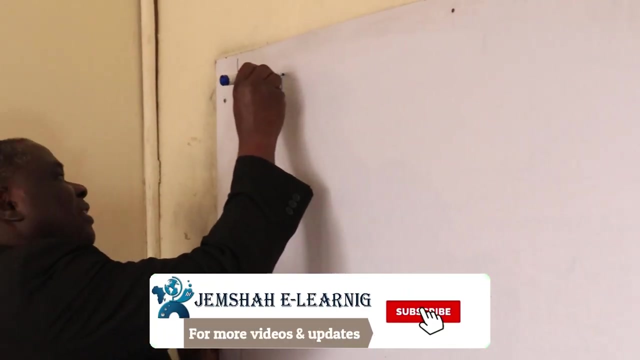 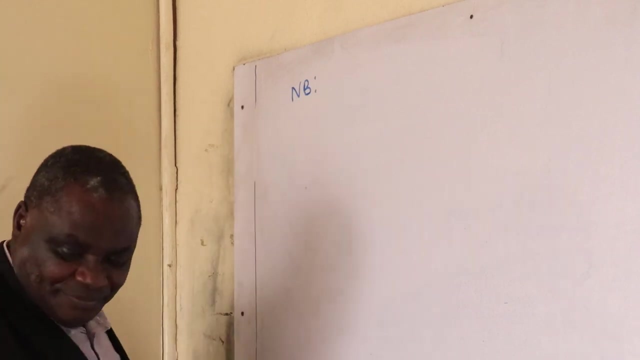 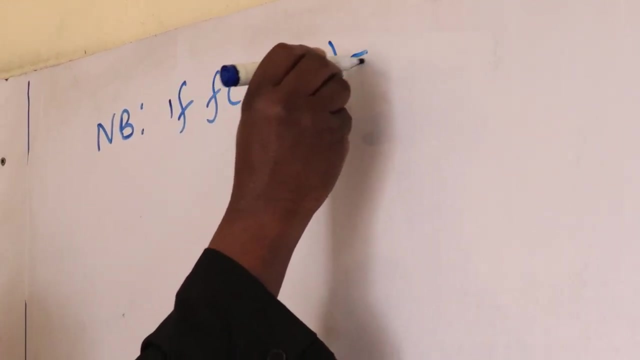 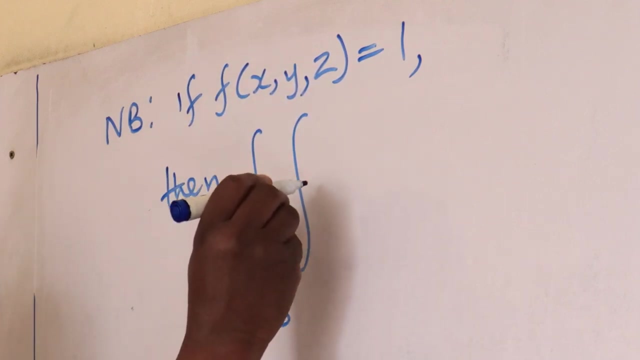 with the dy, dx, because people are used to that, it becomes a bit simpler. So now let's have example one. Now, before we have our example one, we can note something carefully. Let me see: If a function of x, y, z is equal to one, then the double integral, s, d, s will be equal. 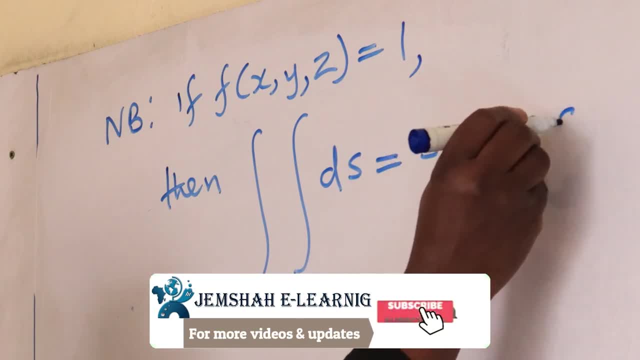 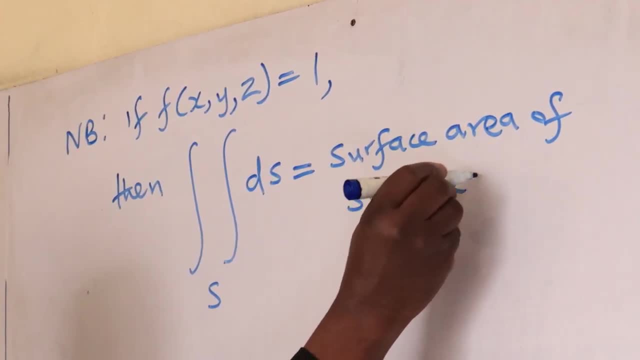 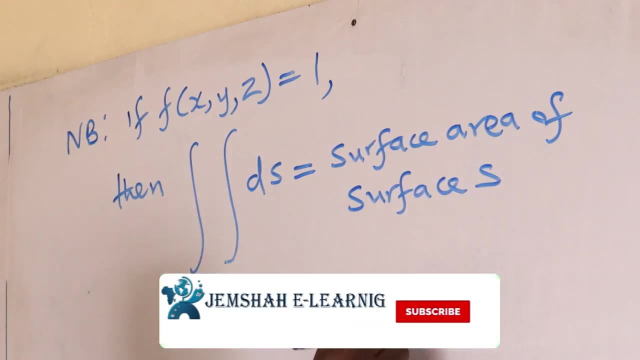 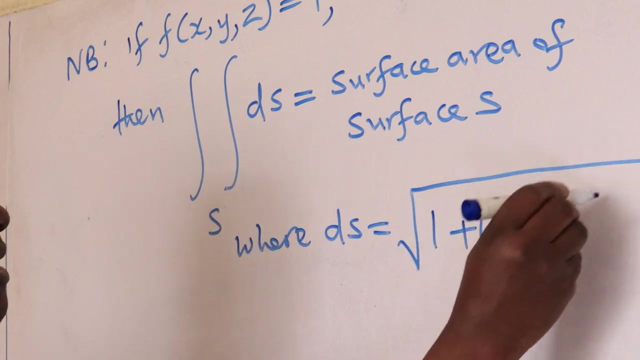 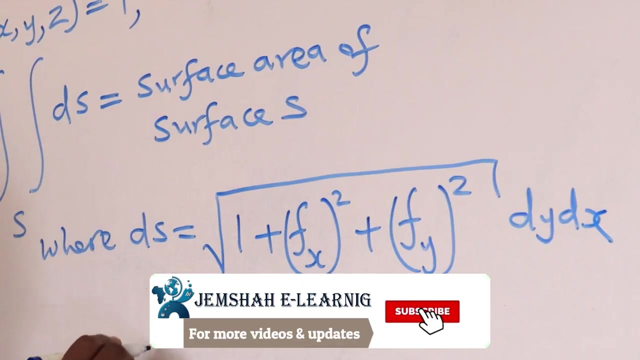 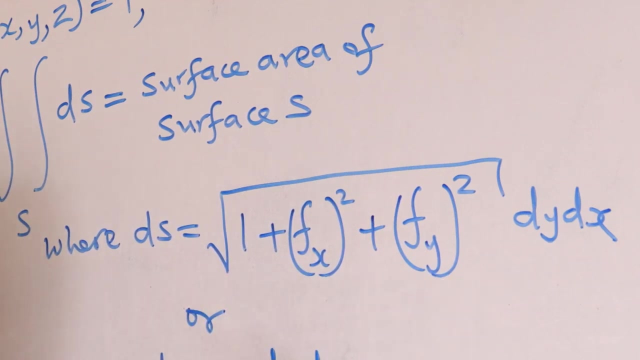 to surface area Will be equal to surface area of surface s Of surface area where ds can be made, as we said, square root of 1 plus f subscript x squared plus f subscript y squared, then dy dx Or ds will be equal to dy dx all over n dot k. 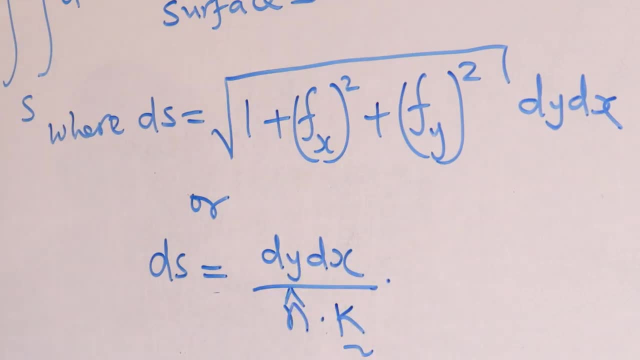 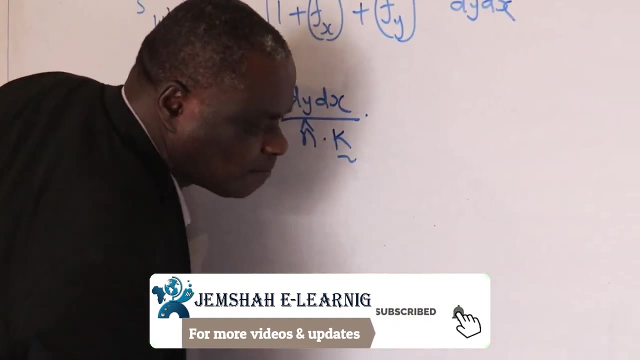 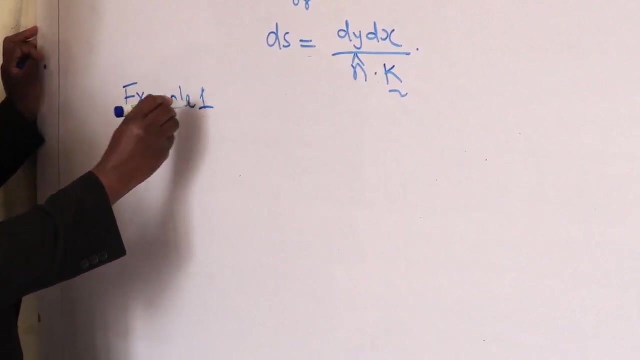 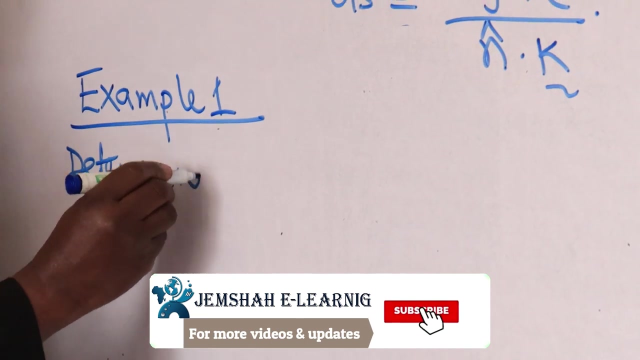 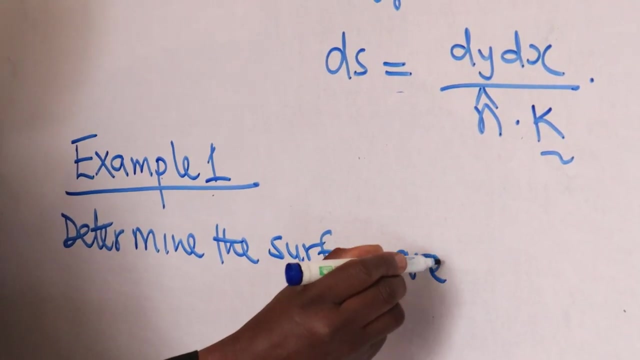 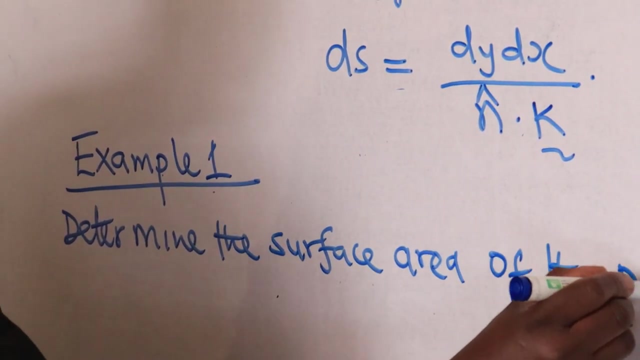 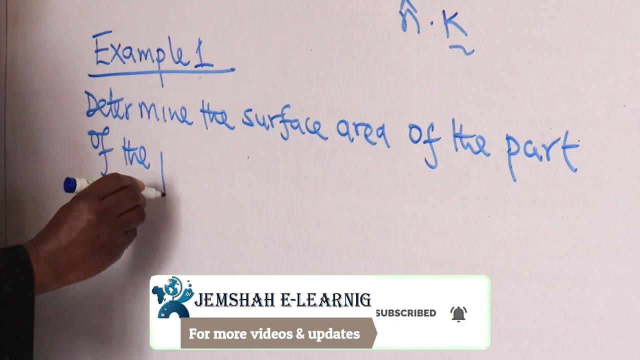 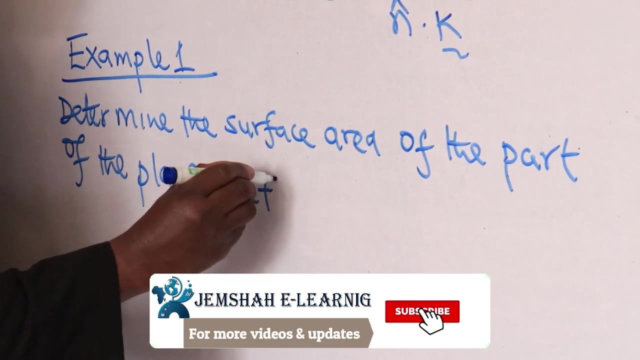 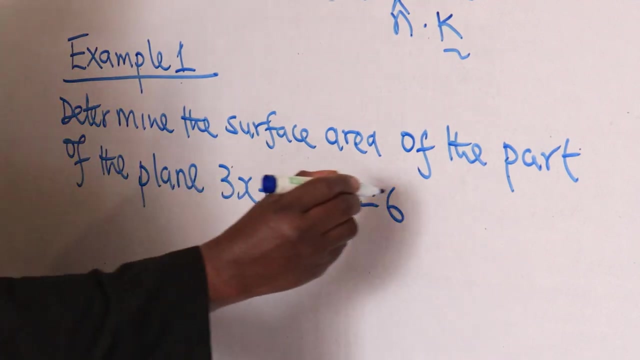 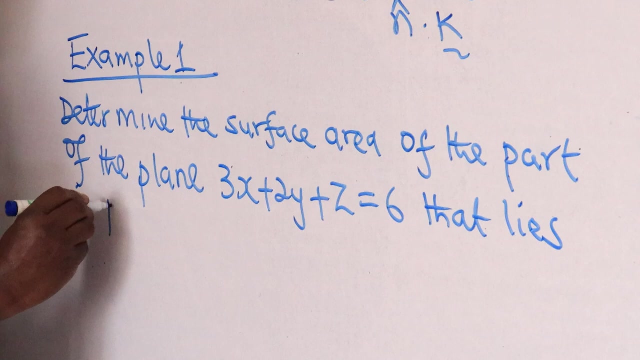 All over n dot k. So example 1. Determine the surface area. Determine the surface area Of the part, The part of the plane, Of the part of the plane, 3x plus 2y plus z is equal to 6, that lies, that lies in the first octant. 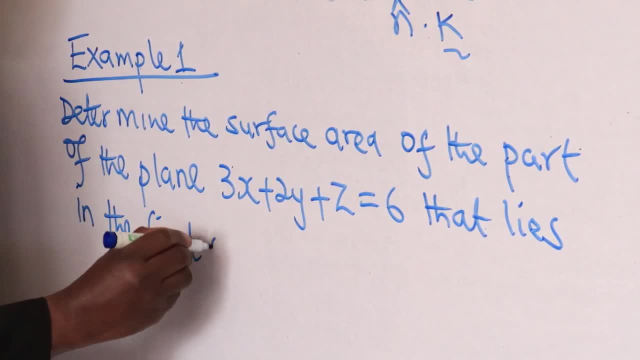 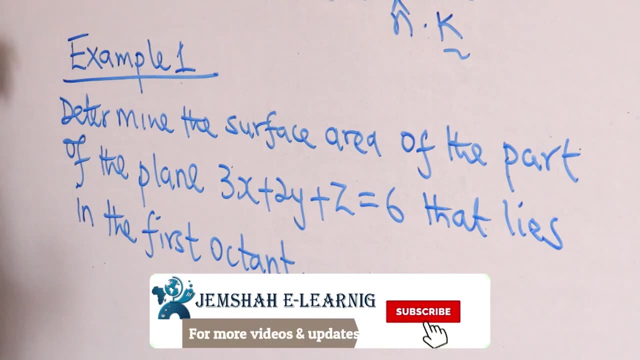 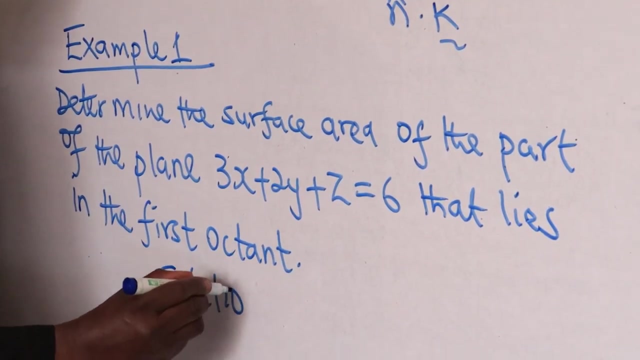 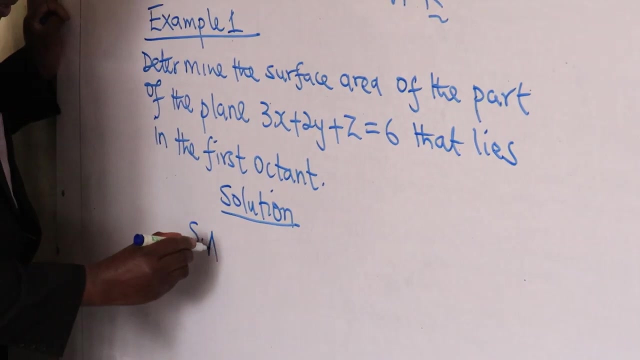 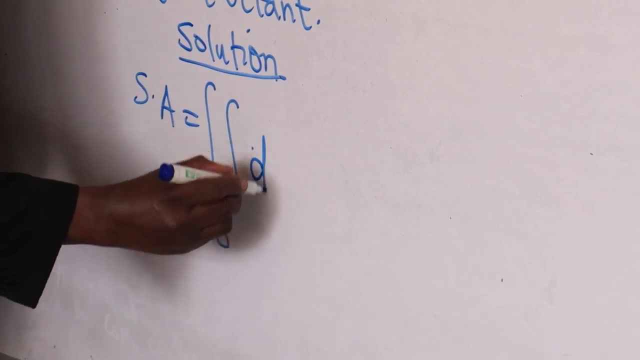 In the first octant. That lies in the first octant. Now, in our solution here, Our surface area. surface area is going to be given by double integral s, and now we have ds, Because now the function of x, y and z is equal to what? 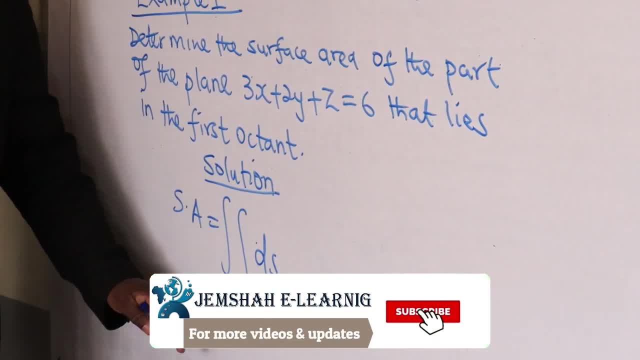 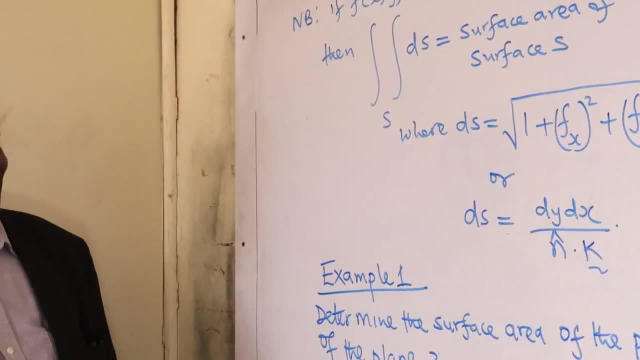 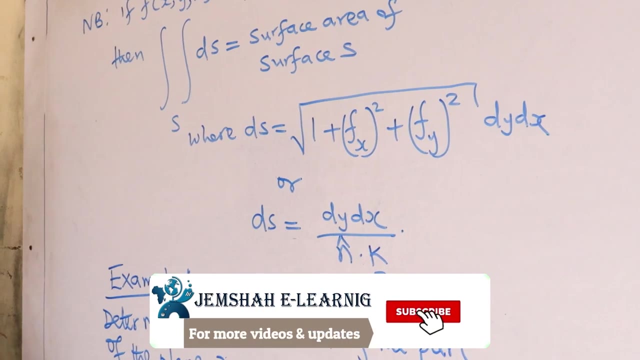 1. So double integral ds, then you have s there. Now we want to convert ds using that particular method. So we would like to get fx and fy. So in this particular connection, from the equation of the surface, 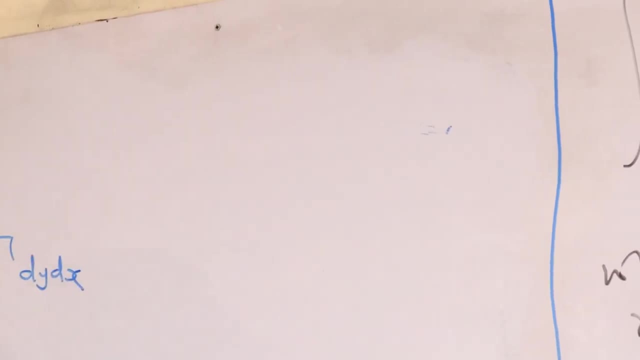 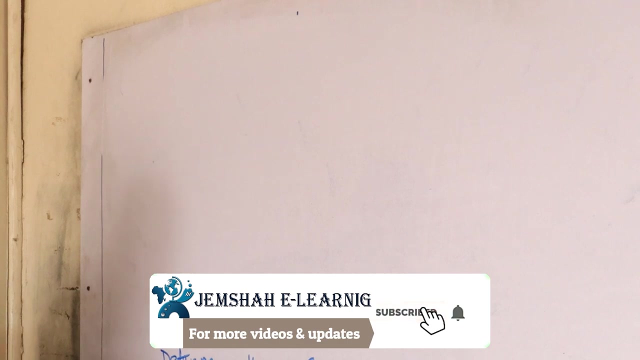 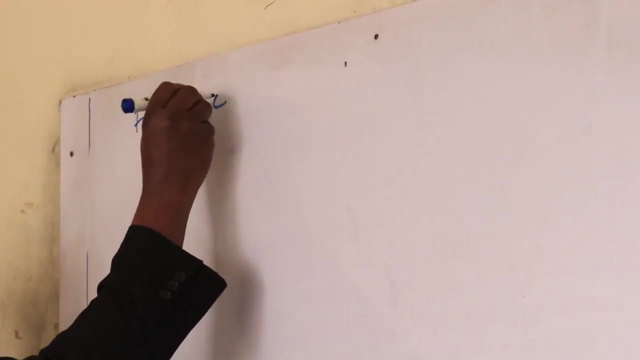 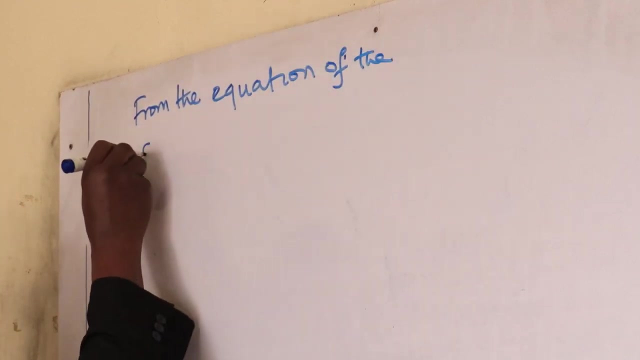 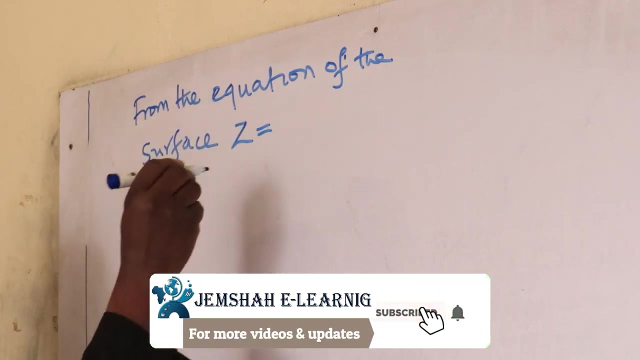 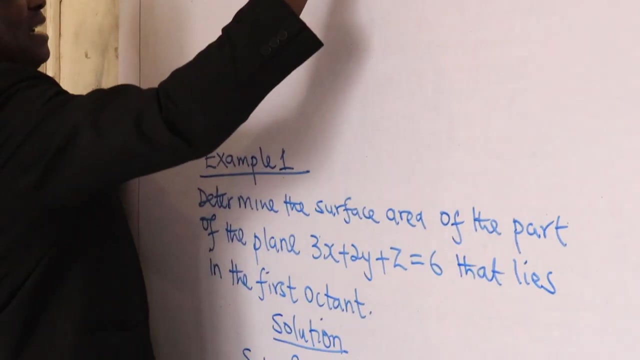 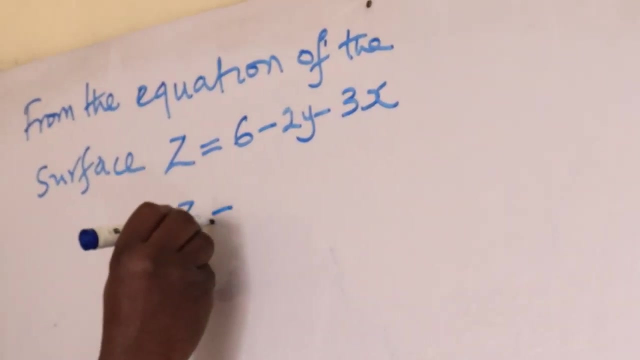 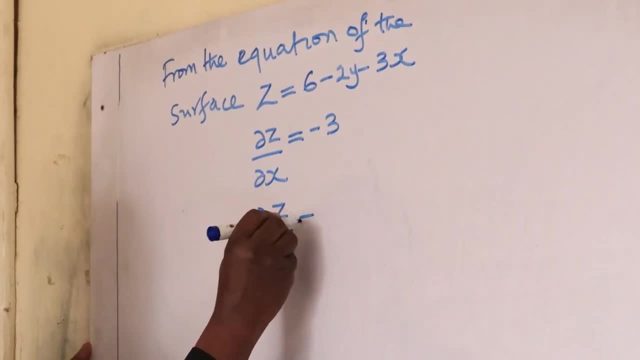 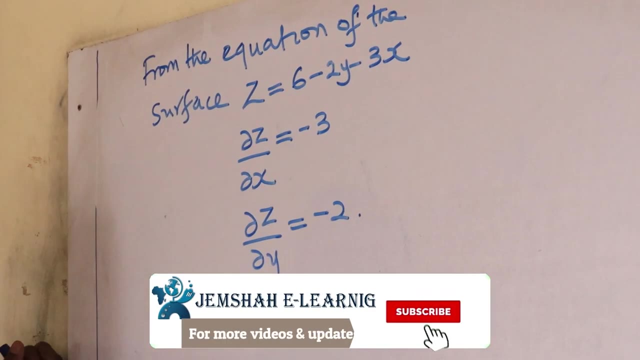 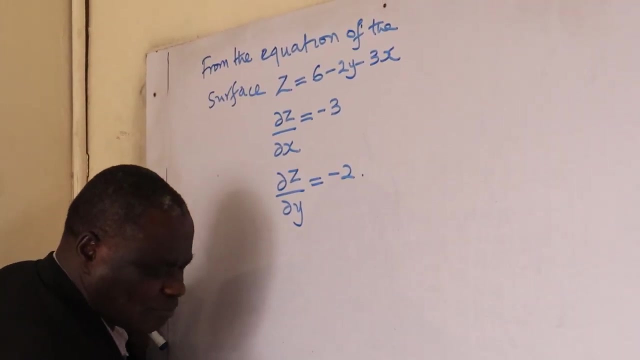 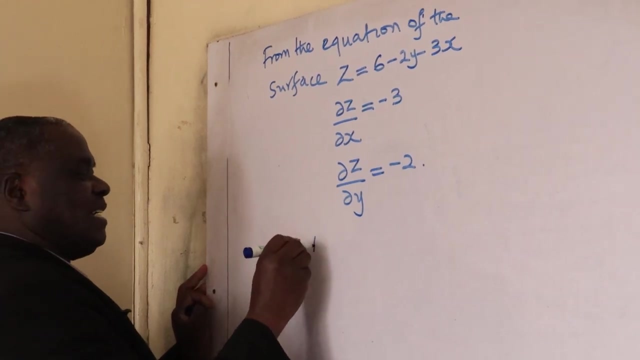 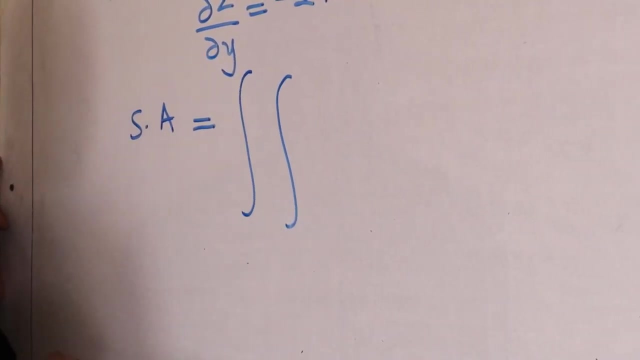 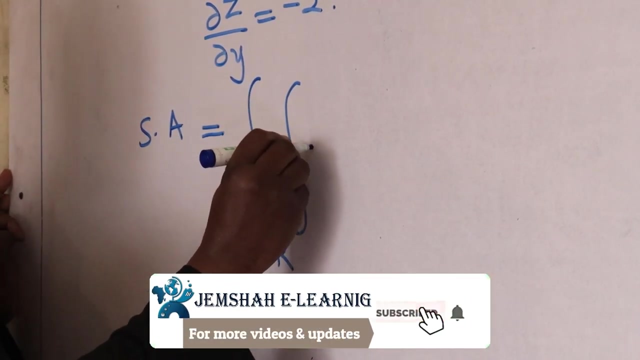 dz dy will be equal to what Minus 2.. Now, from that particular arrangement we now say So, our surface area will then be equal to a double integral. Now we are going for region R. Then our ds now will be equal to square root of. 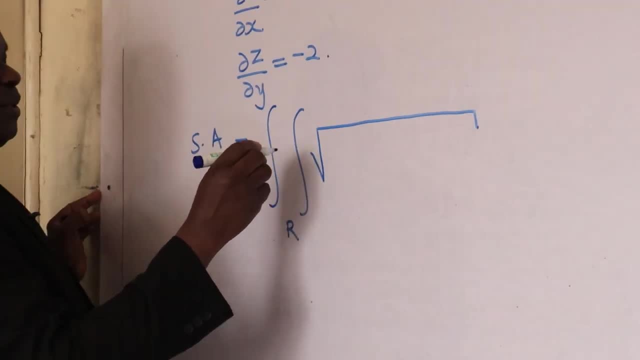 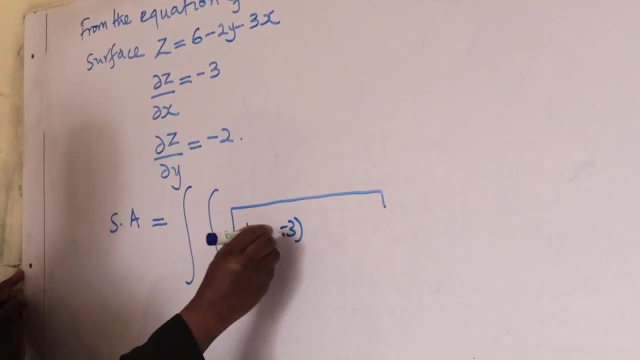 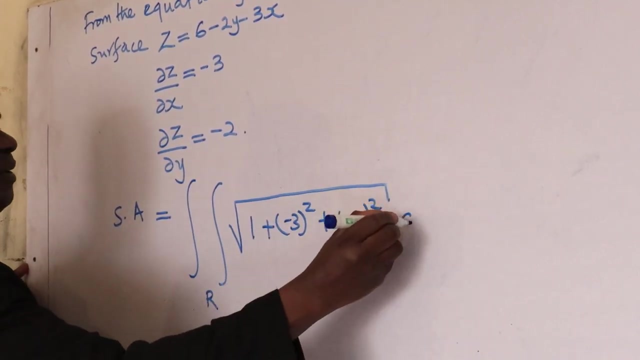 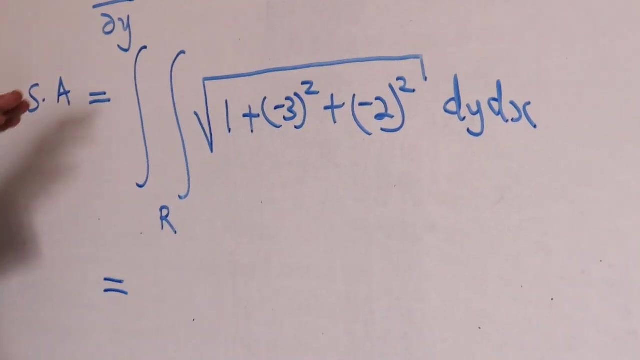 Let's just input those. We are inputting 1 plus dz, dx minus 3 squared, dz. y minus 2 squared. Then here we will have dy dx, Which will now be equal to When you project that surface on xy plane. 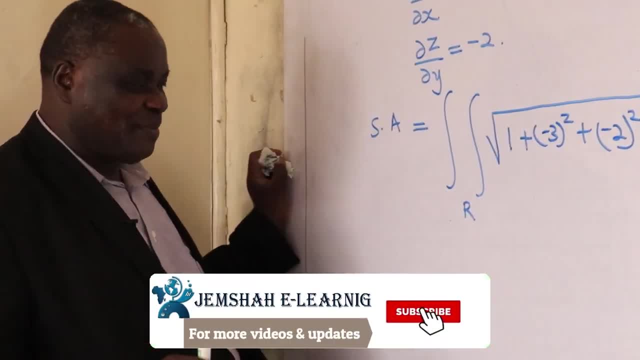 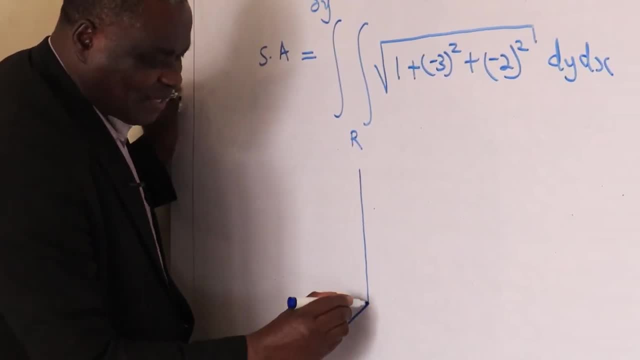 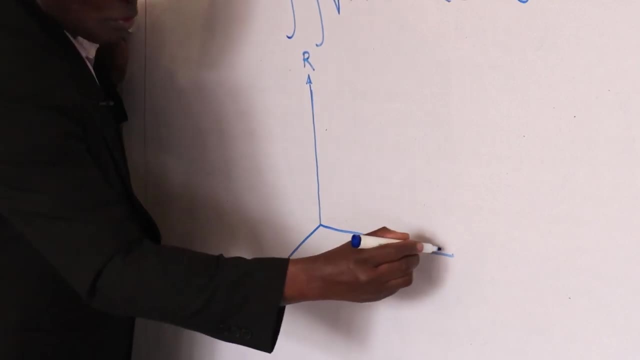 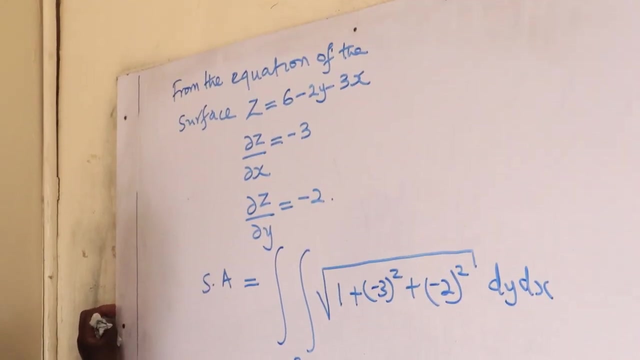 When we project it on xy plane, It will now be something like this- Maybe you can see it from a diagram. So our surface was: 3x plus 2y plus z is equal to 6.. When x and y are all 0.. 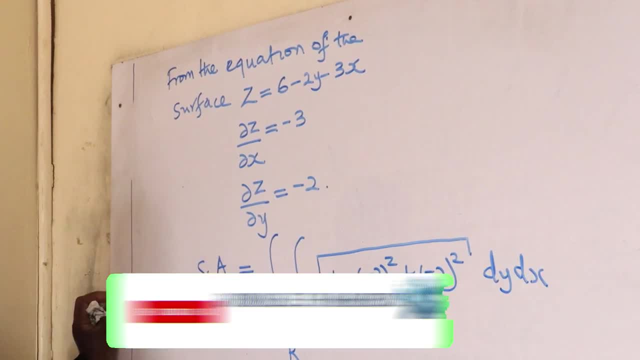 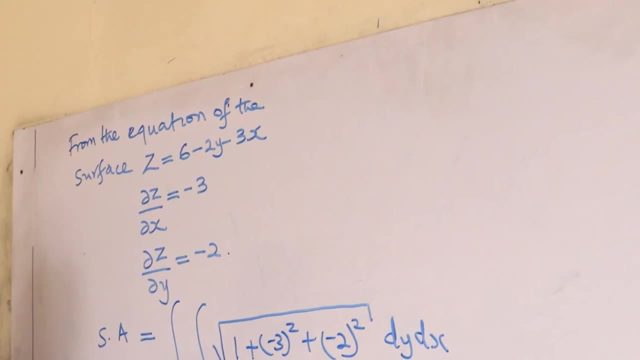 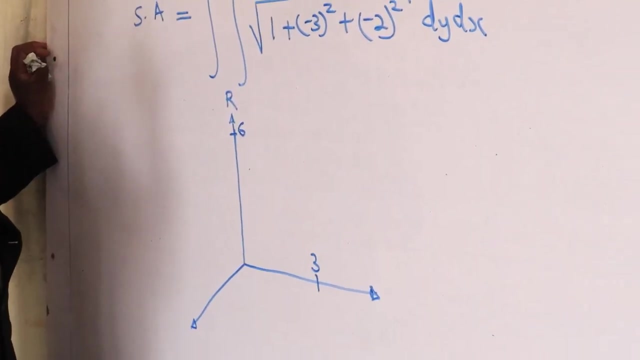 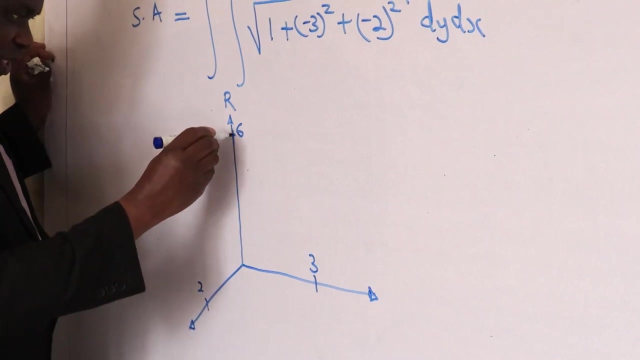 z will be equal to 6.. When, When z And x are 0. y will be equal to 3.. When Both z And y are 0., x will be equal to 2.. So the plane we are talking about. 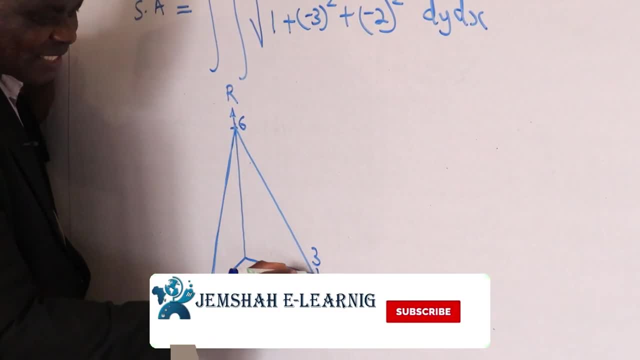 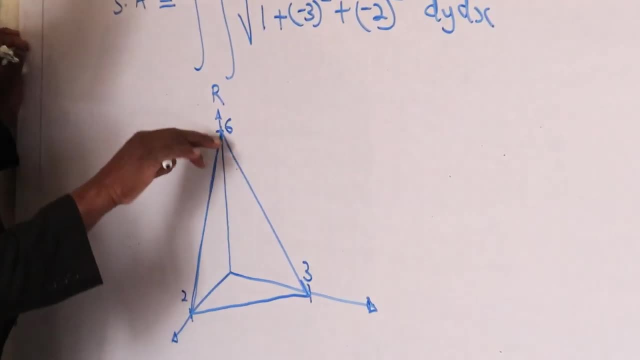 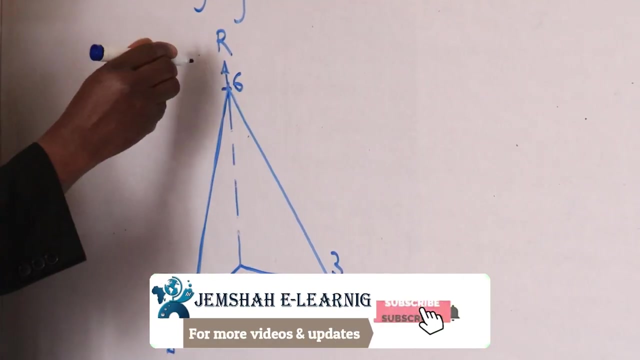 Is this plane that appears on this, On our first octant, And if it is appearing here, This is now When we project it, When we project it On xy plane, Because this is z, That is y, This is x. 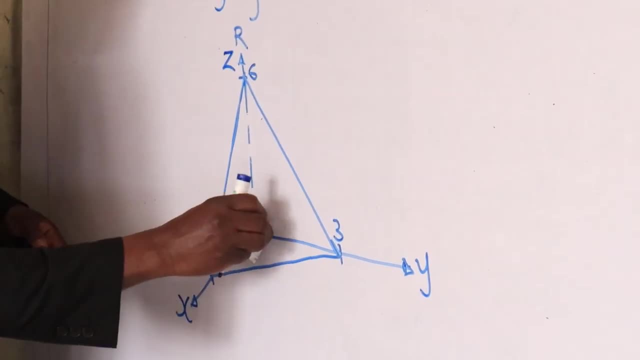 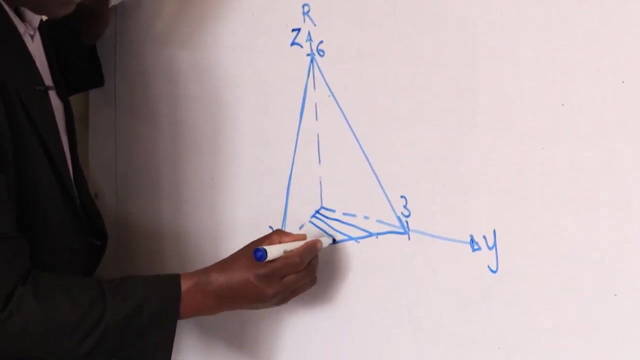 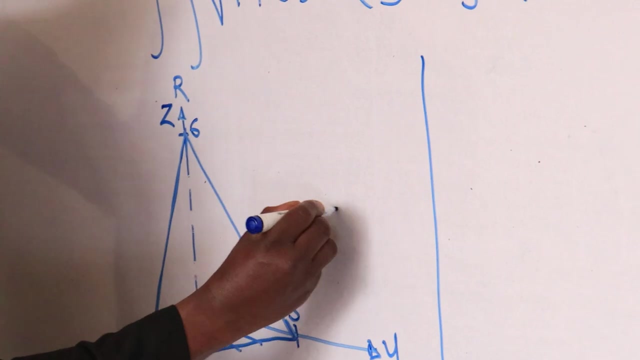 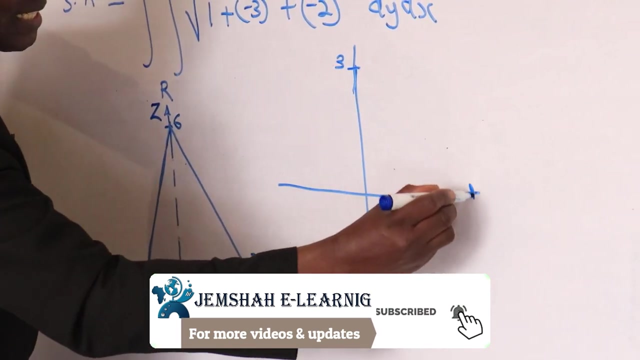 When we project it, The plane, This is the Our region. what Region r? So For us to see it nicely, We can draw it on an xy plane Plane. So here y It is at 3.. The x intercept is at 2.. 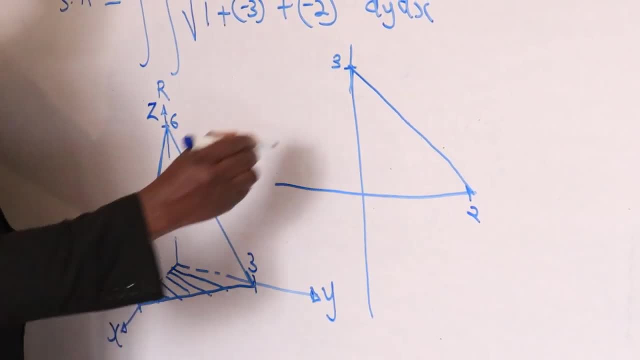 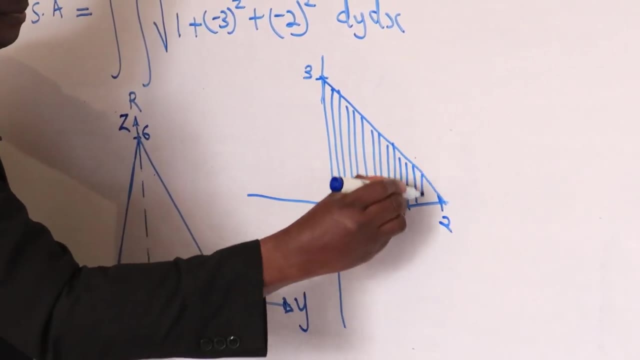 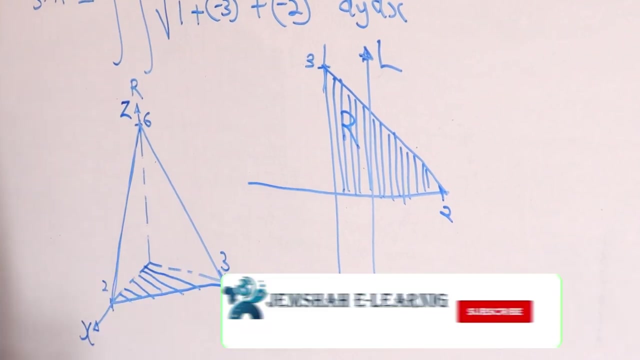 So we have something like that. So this is the region of integration. now That becomes our region of integration And we can draw our line l here. So this is our region r r Now. From that We can get our limits. 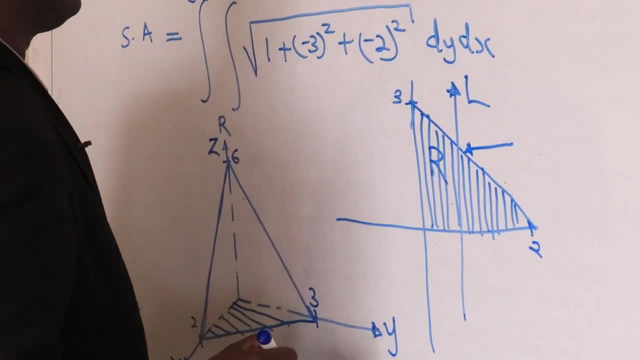 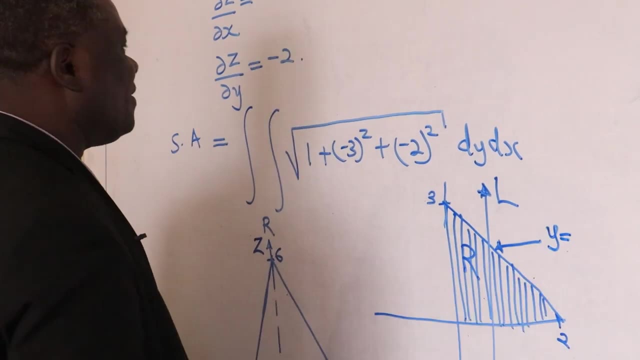 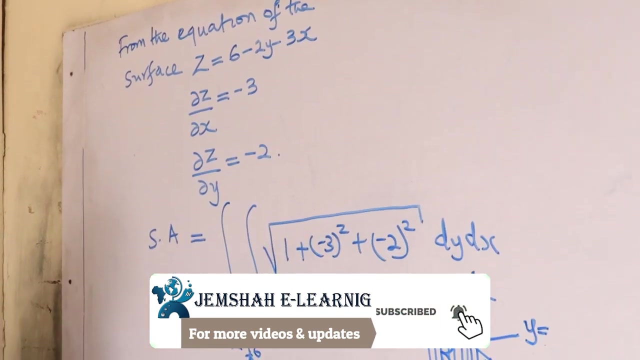 This line, we can call it now. This line, we can call it: Y Is equals to, Y is equals to When z is 0.. When z is 0. That equation will be: 3x plus 2y is equal to 6.. 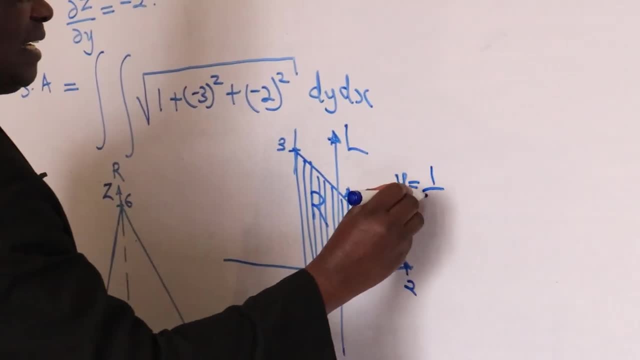 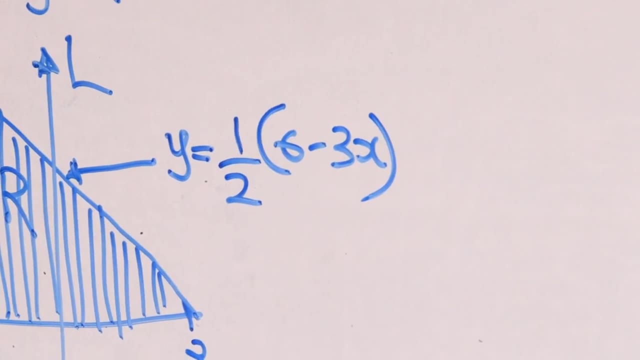 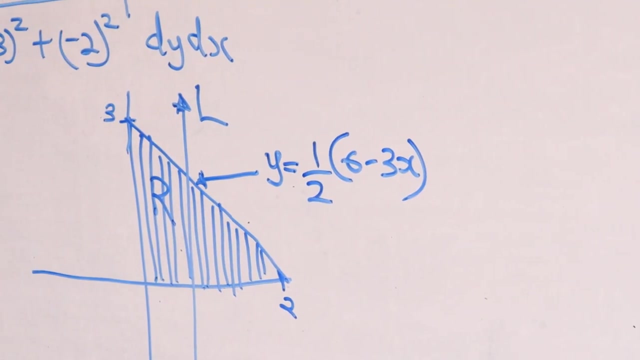 So y is equals to a half Into 6 minus 3x. Y is equals to a half Into 6 minus 3x. Now, After having those values ready, We can now be able To proceed With our 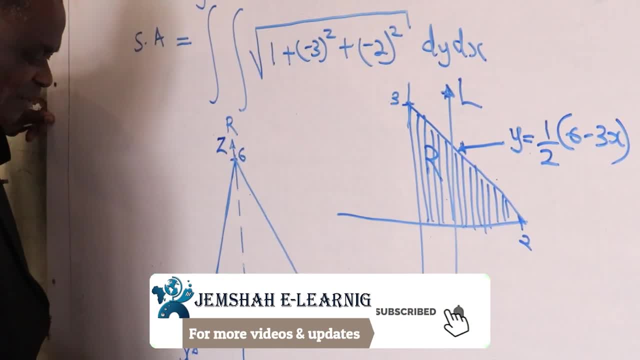 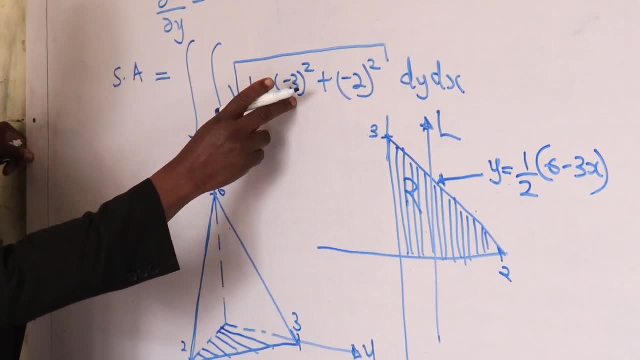 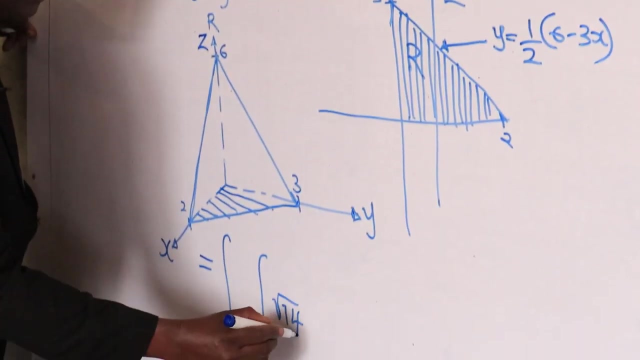 What With our surface area analysis? So we have our double integral there. This is root, what This? 1 plus 9.. 1 plus 9 plus 4.. That's root 14.. Root 14.. Then divide here. 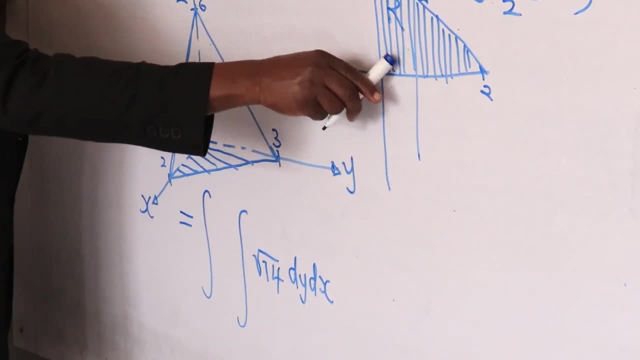 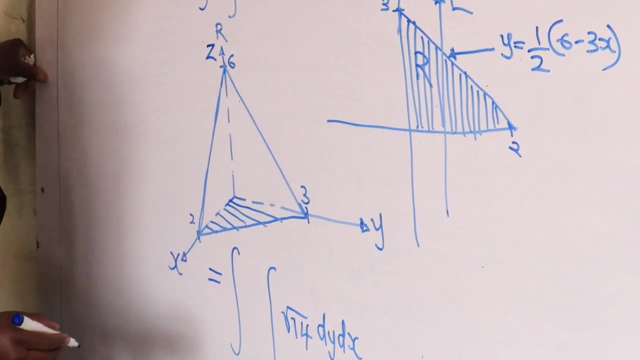 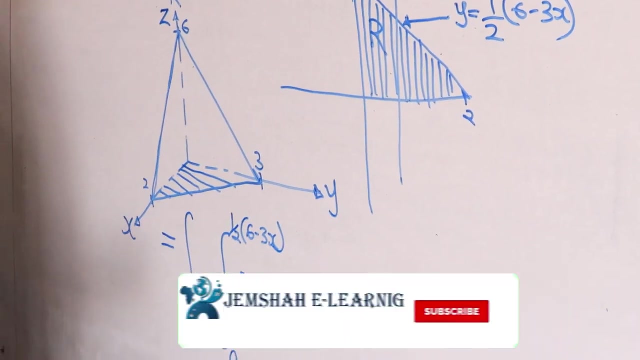 dx. Now In this, From this particular region, We can see the limits will be. Starts from y is equal to 0. To y is equals to A half into 6 minus what 3x And x is, starting from 0 to 1.. 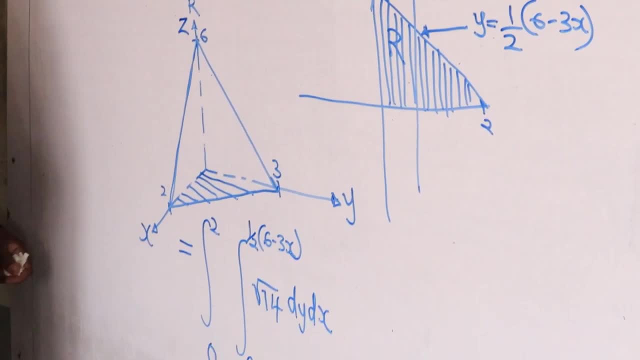 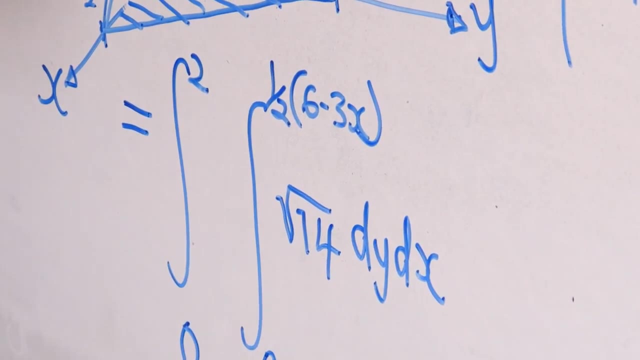 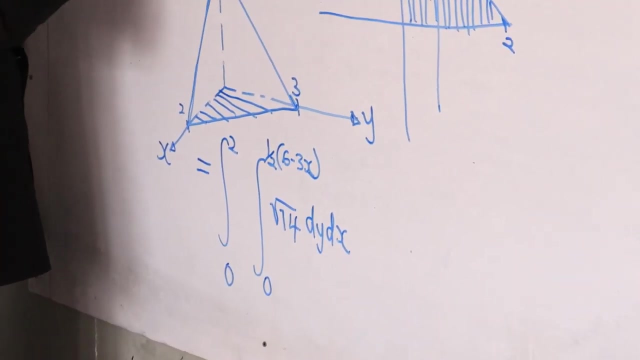 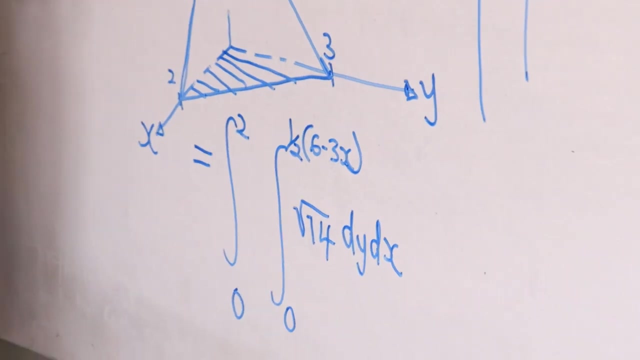 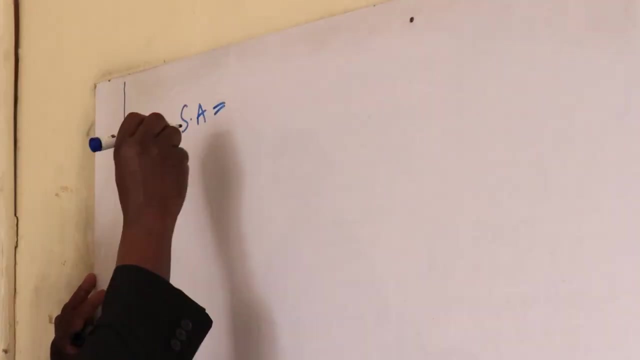 0 to 2.. So this one will now give us The surface area. Let's now evaluate it. Let's now evaluate it So evaluating. So our surface area Will be equal to 0 to 2.. 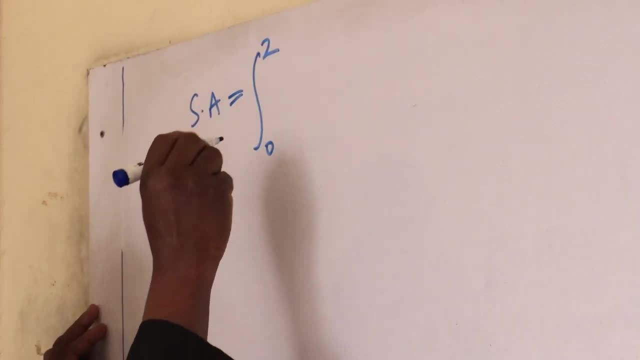 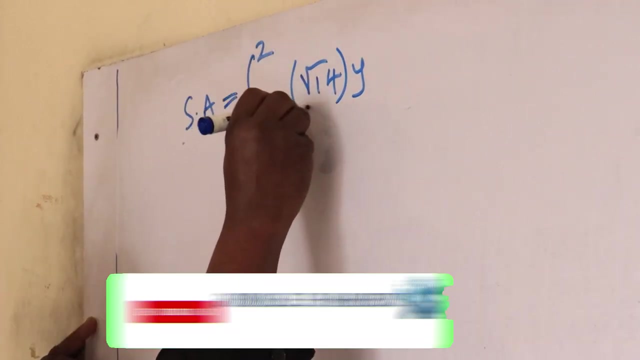 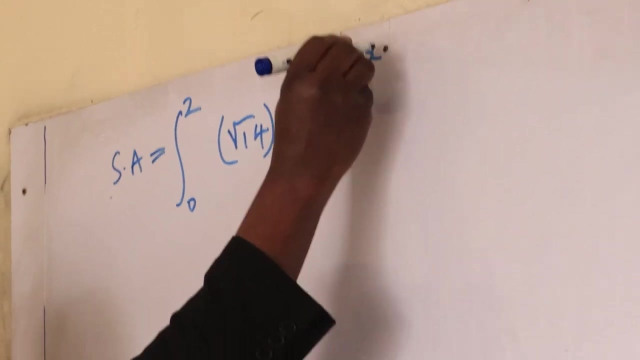 Then we have Root 14.. Will multiply y. Root 14 will multiply y. Will put limit 0 to a half Into 6 minus 3x. Then we have here, And then we have here dx remaining. 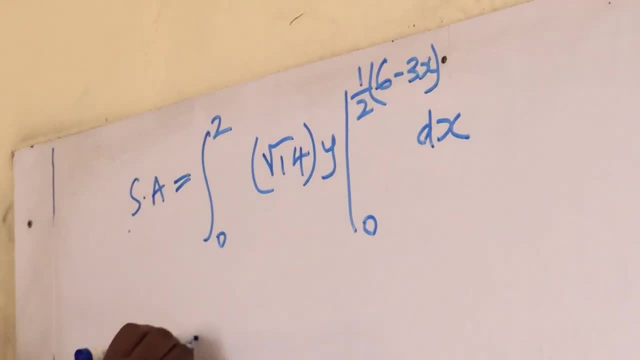 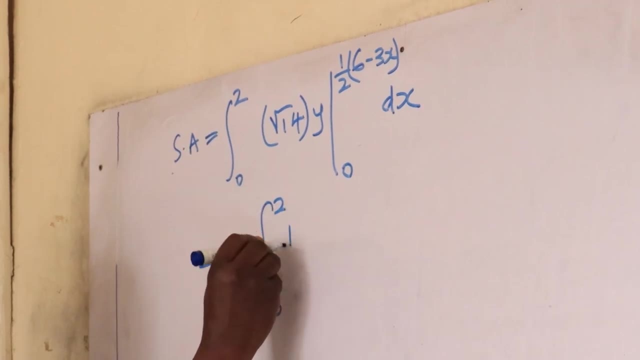 We have evaluated the first integral, So this one Root 14.. We know it's a constant, It can even go out. We have 0 to 2. Then we have a half When you insert here Where there is y. 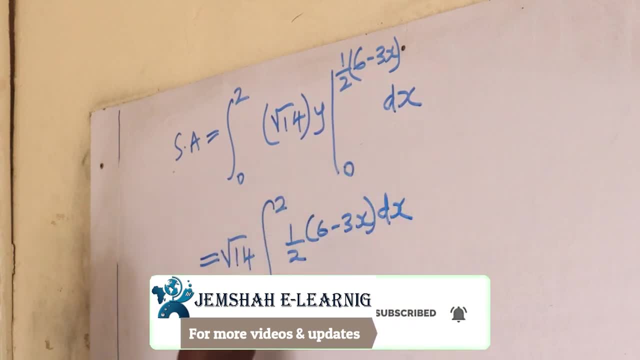 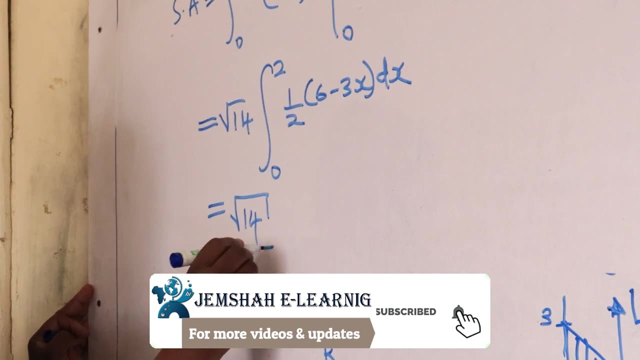 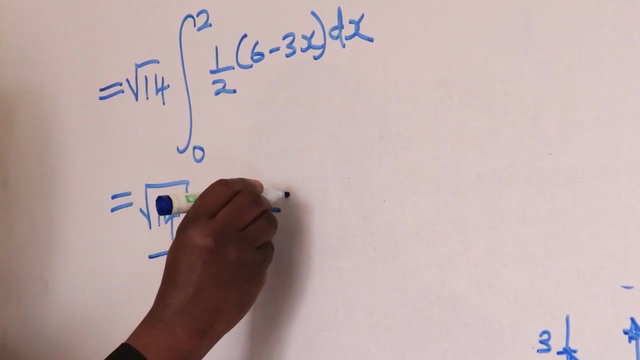 6 minus 3x, Then dx, Which is equal to root 14. Root 14. Over 2. We can have it there. When you integrate this, We get 6x Minus 3, all over 2.. 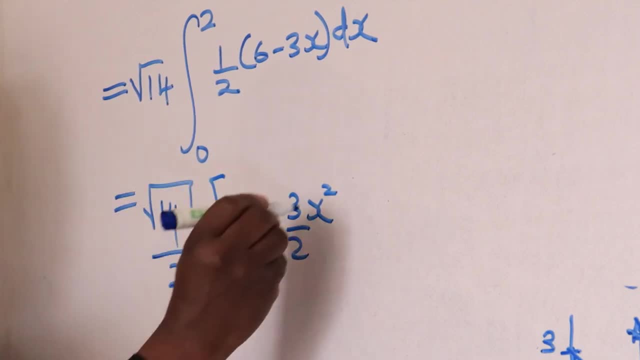 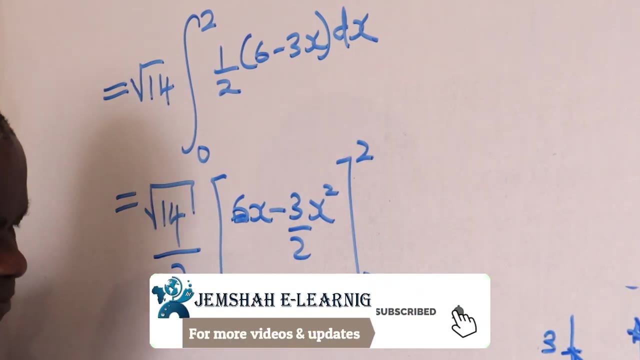 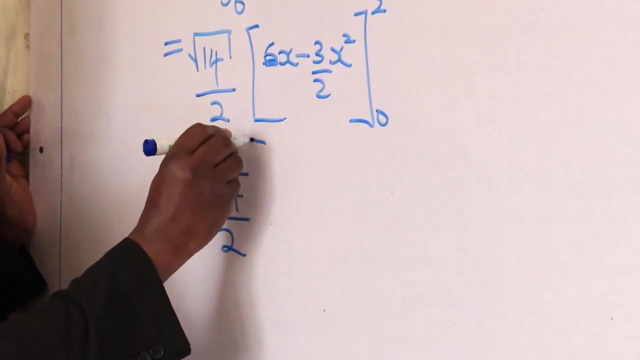 x square Square. And then we have our limits, From 0 to what? 0 to 2. So this will be equal to Root 14. All over, 2. A into We insert 2. here We get 12.. 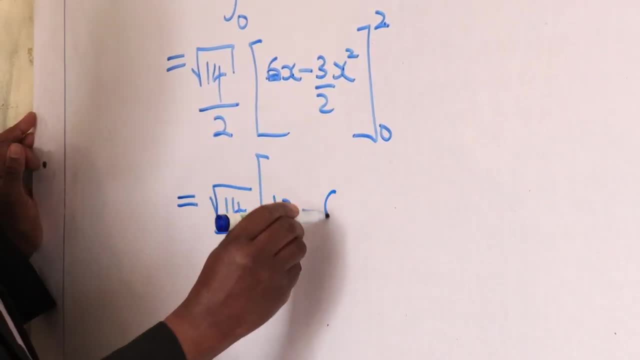 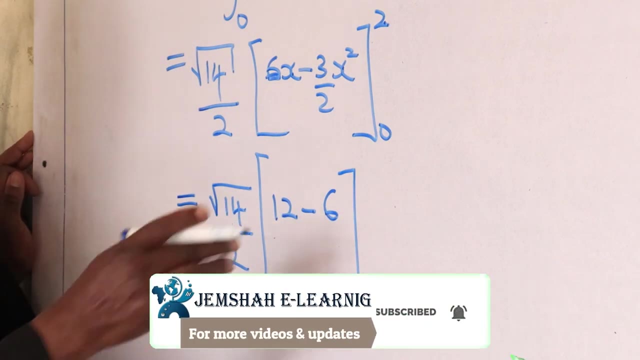 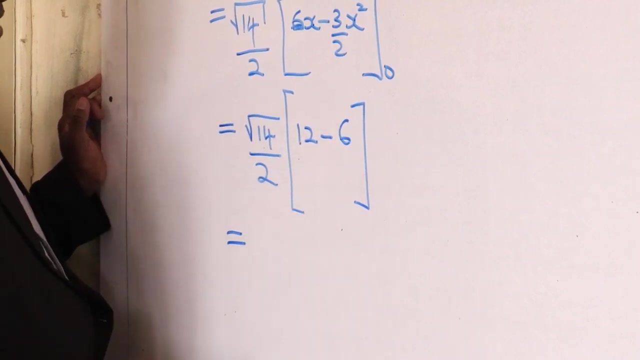 We insert 2 here, We get minus 6.. 3 over 2 times 4. We get 6.. The lower limit will bring all the 0s. So this one gives us 12 minus 6 is 6.. 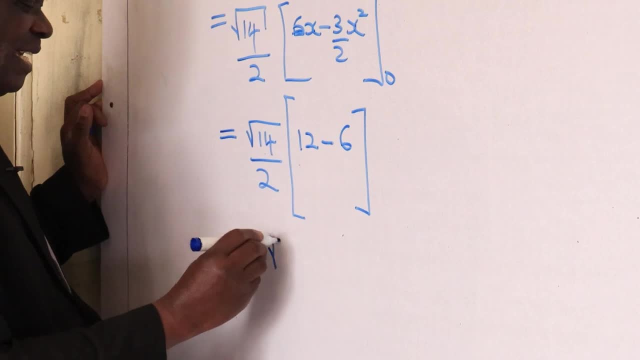 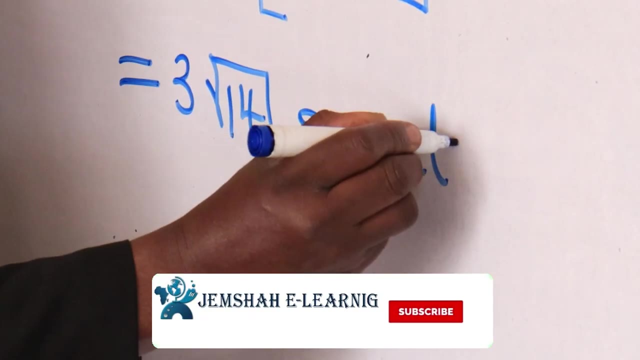 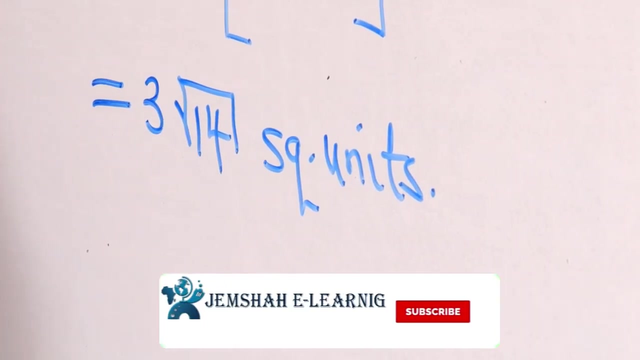 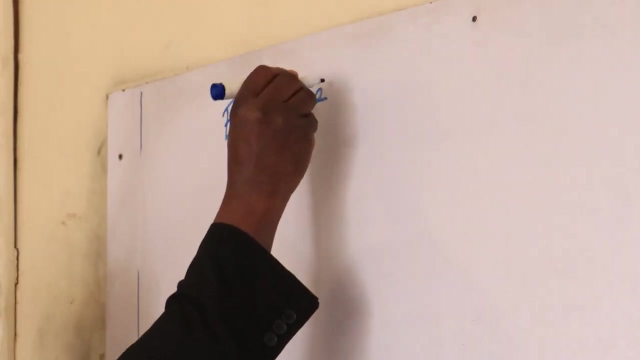 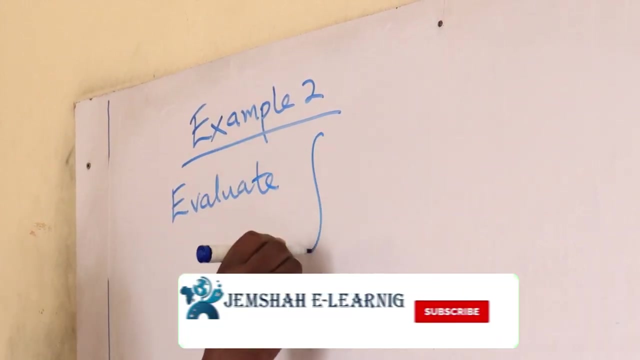 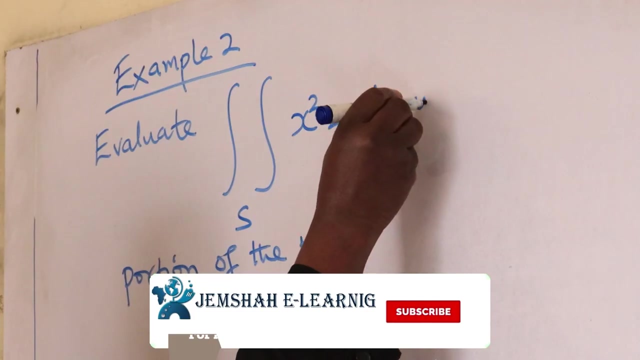 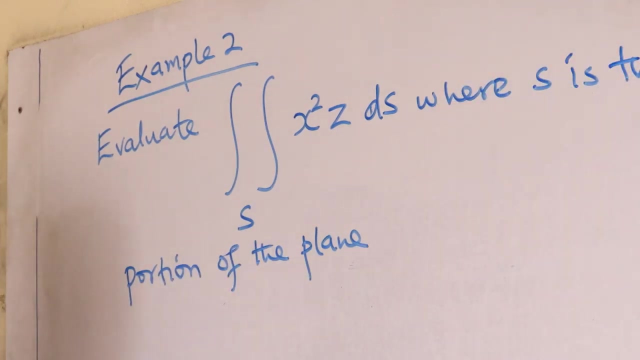 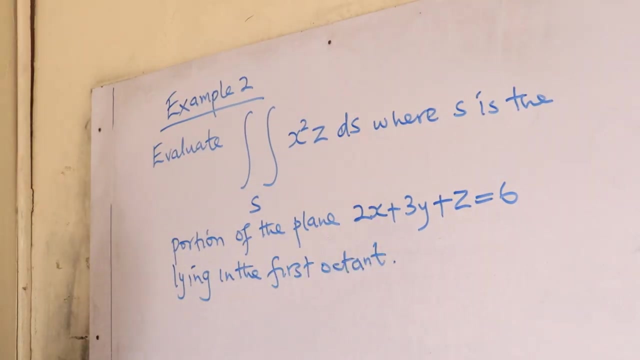 6 divided by 2 is 3.. So the answer is 3 root 14.. Now square unit Units, Because it was about A surface area. And that is the end Of that particular work. So So here we are told. 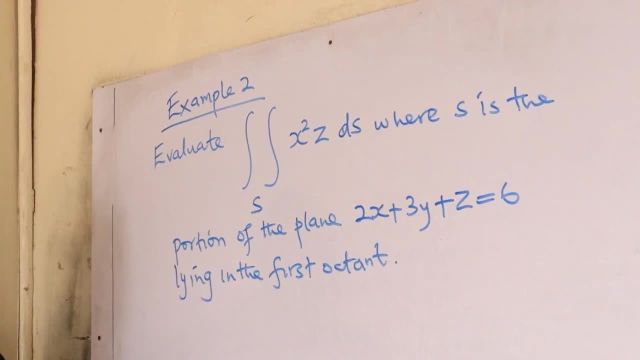 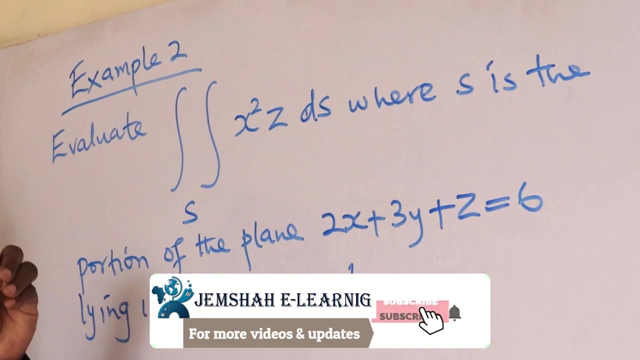 Evaluate, Evaluate, Evaluate In our example: 2. Evaluate This double Surface integral. Where s is the portion of the plane? 2x Plus 3y Plus z Is equal to 6. Lying in the first. 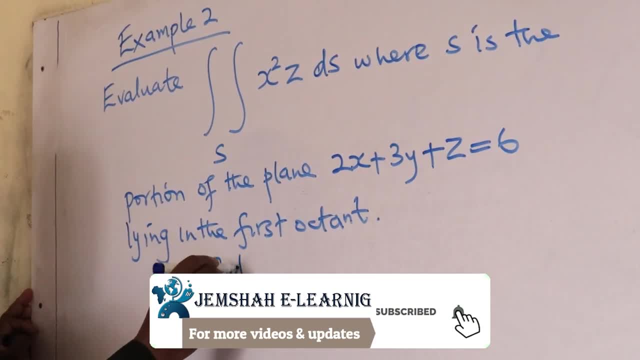 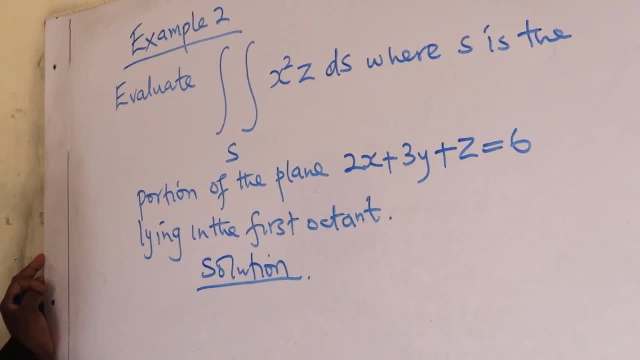 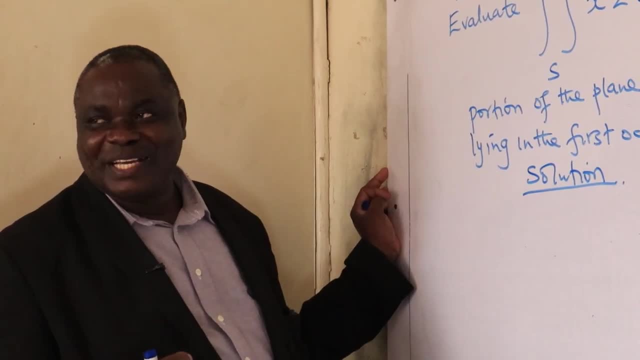 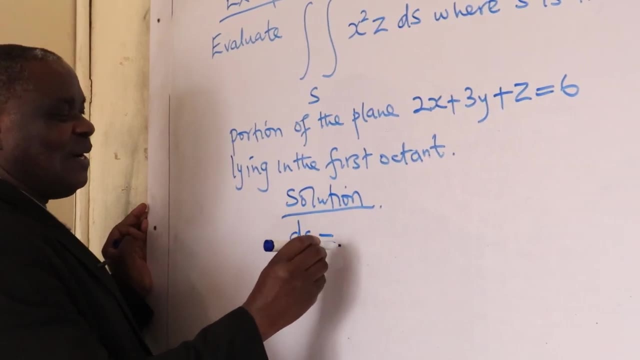 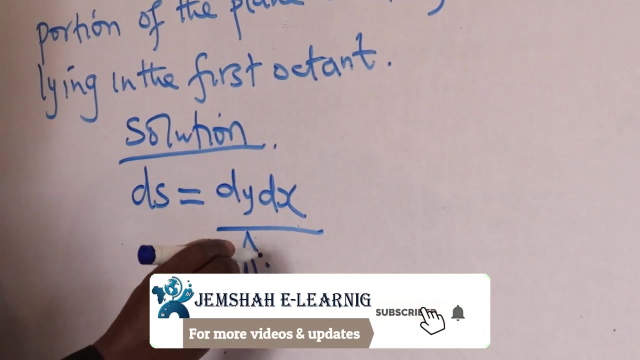 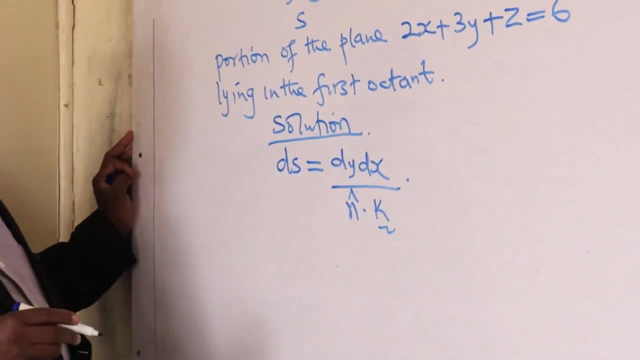 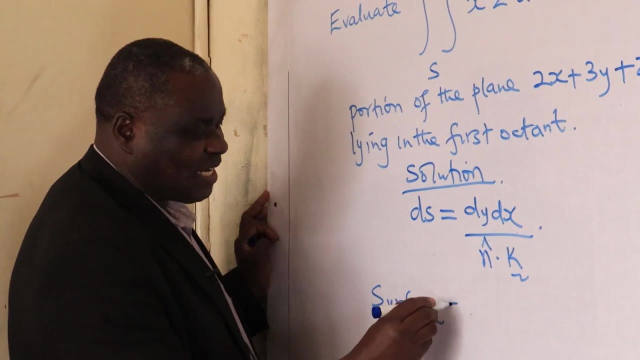 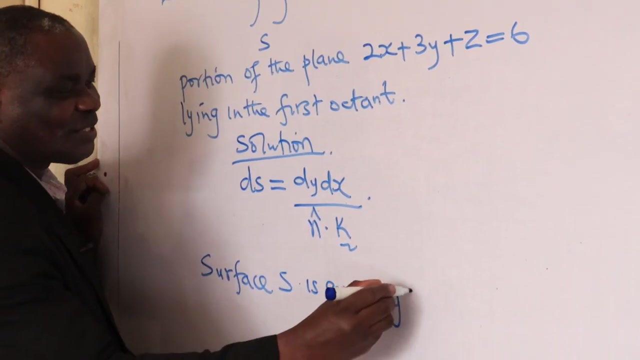 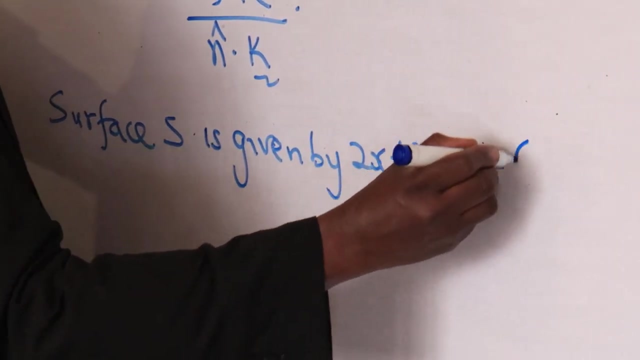 To change into In Now our surface, Now our, Now Our Surface S. Equation Of the is given by, is given by: 2x plus 3y plus z minus 6 is equal to 0.. 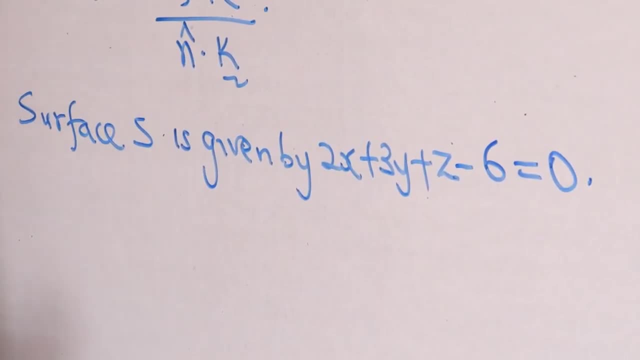 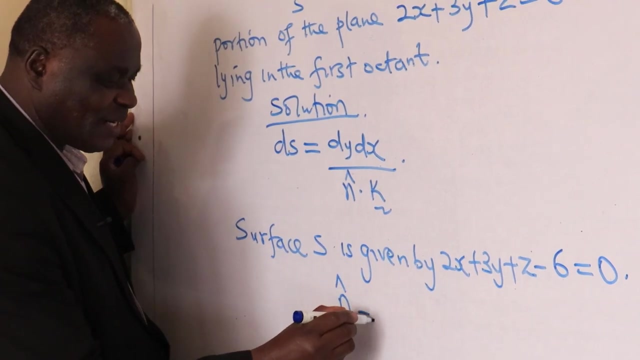 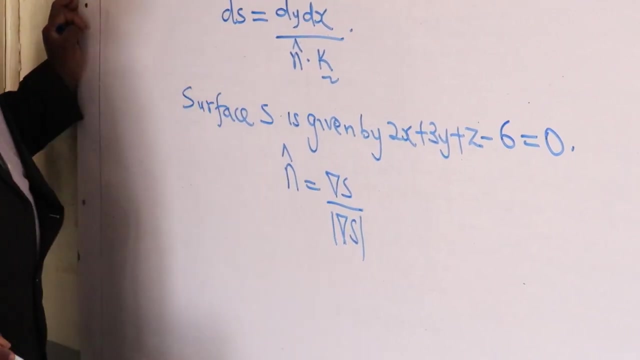 So we are saying now, if that is the equation of the surface, we want to get the normal vector, And the unit normal vector is given by what? Grad s? all over grad s, my magnitude, Grad s. all over grad s, my magnitude, Grad s. 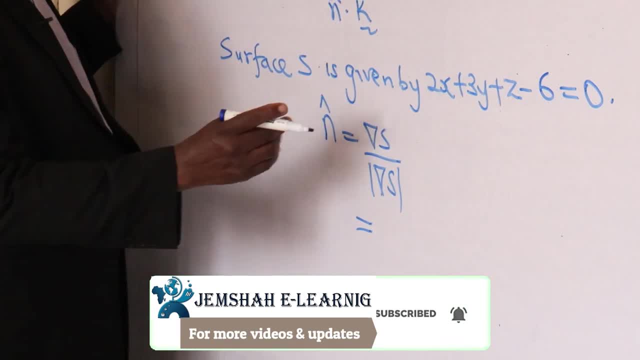 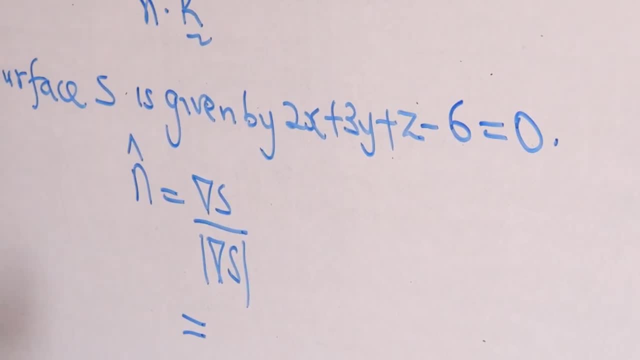 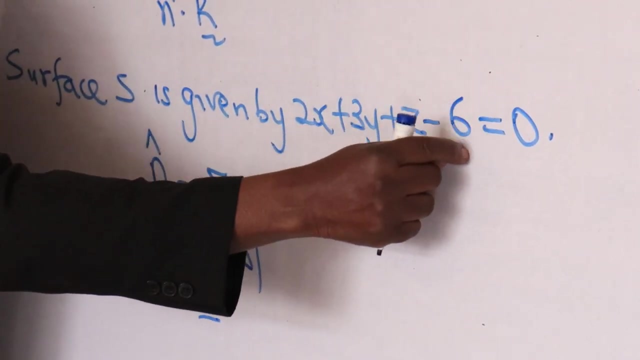 meaning what We are going to do. this is the equation of our surface. so we are going to differentiate that with respect to x. first Give it letter i. So if you differentiate this with respect to x, we get 2.. So we give it what? 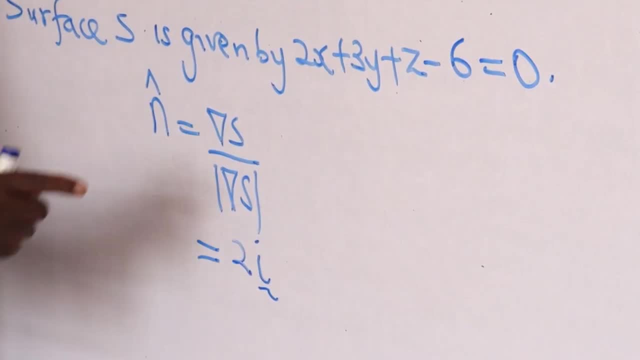 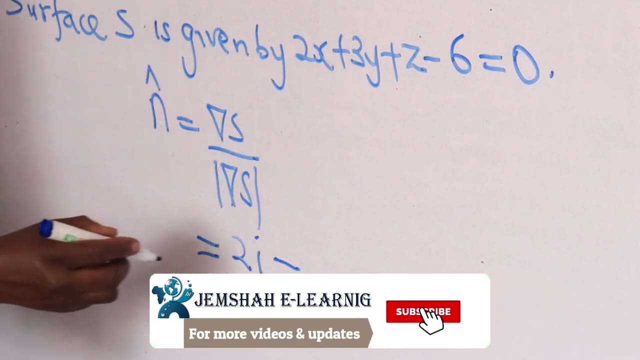 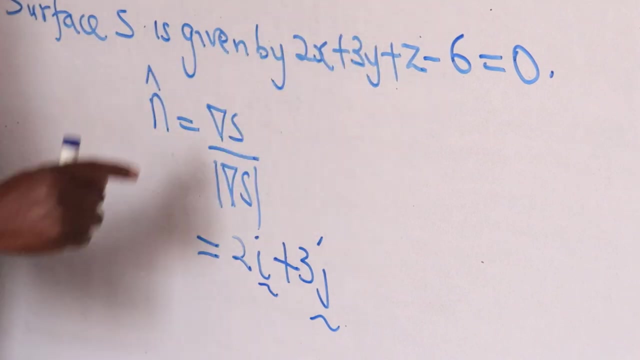 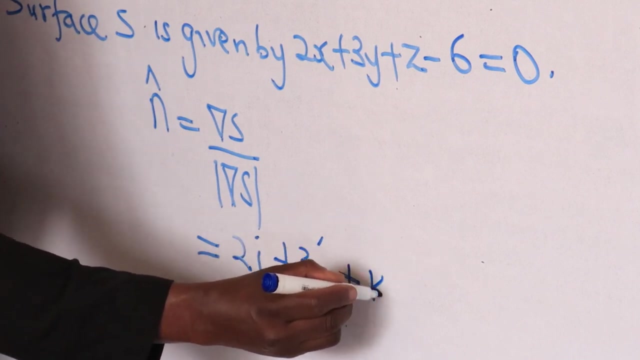 2i. Differentiate the whole of this with respect to y. That is partial derivative. It will be 3. So 3j. Differentiate the whole of this with respect to z. We get 1. So 1 and it's multiplying k. 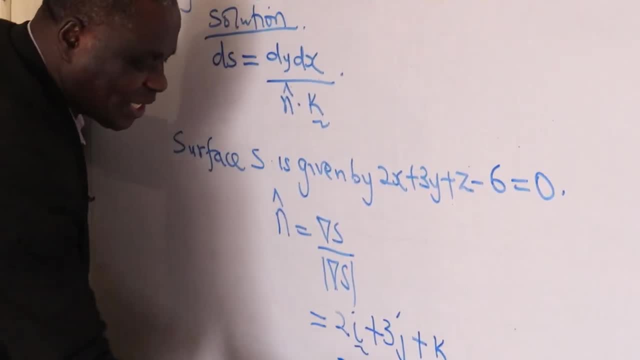 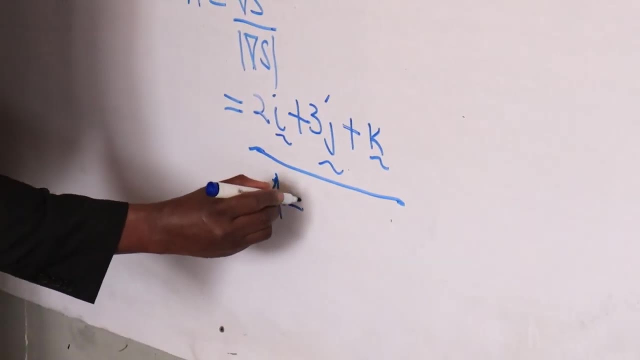 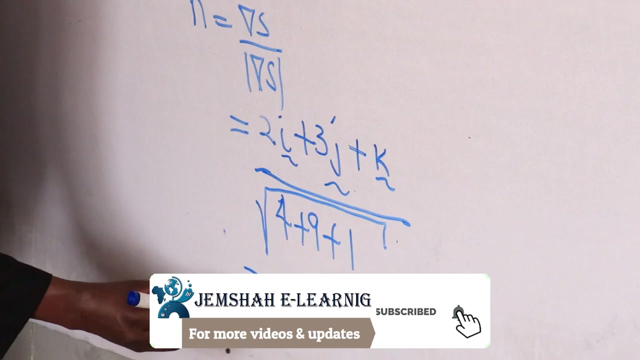 k. So that is our grad s. Now we divide by its magnitude. What is the magnitude? It will be 4 plus 9 plus 1 with a square root, with a square root, So it will be equal to 1 all over root 14. 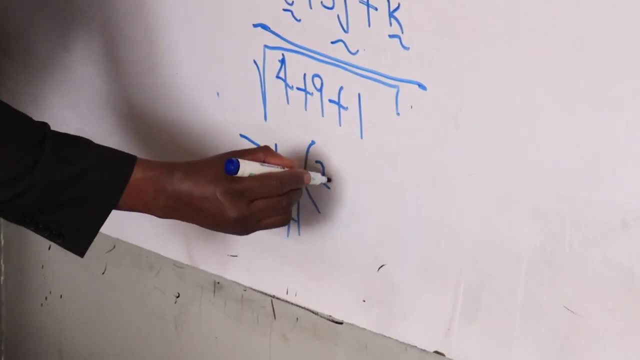 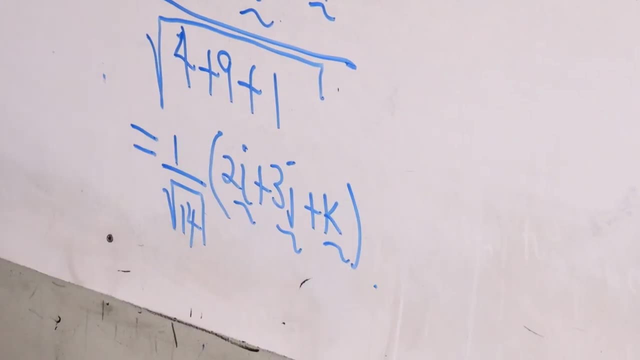 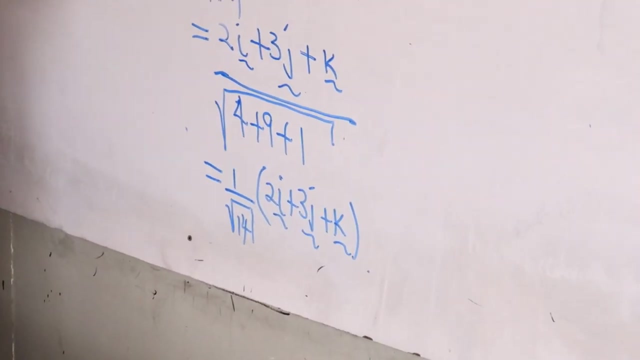 into 2i plus 3j plus k plus k, The actual number of degrees of a square root of 1.. So we have to look at the integral of k to find the integral of n, And what we study is that k is the integral. 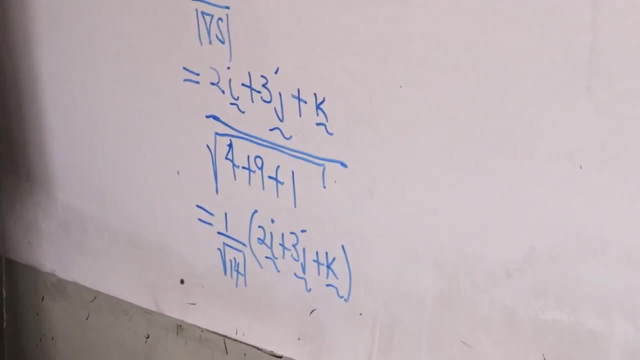 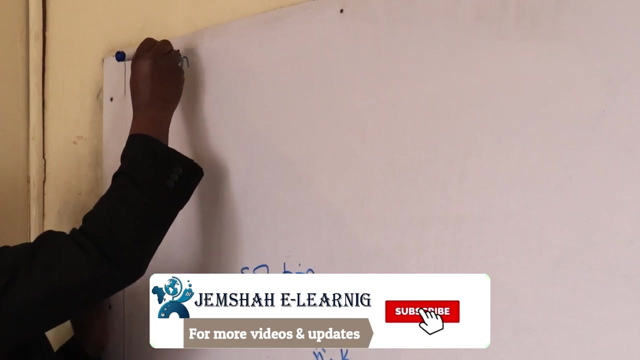 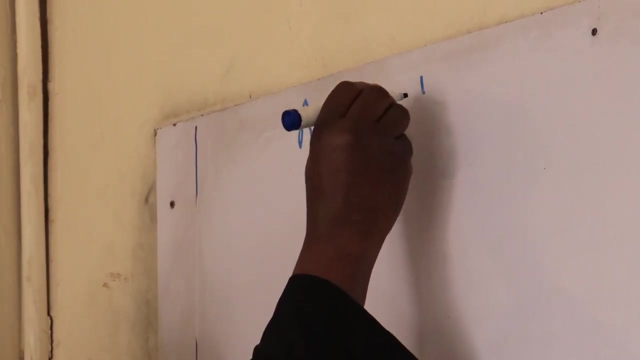 of n. So we can see that k is equal to, k is equal to 1 all over root 14.. And we know that k is equal to k plus k. So now we put k and we get k plus 2i plus 1. 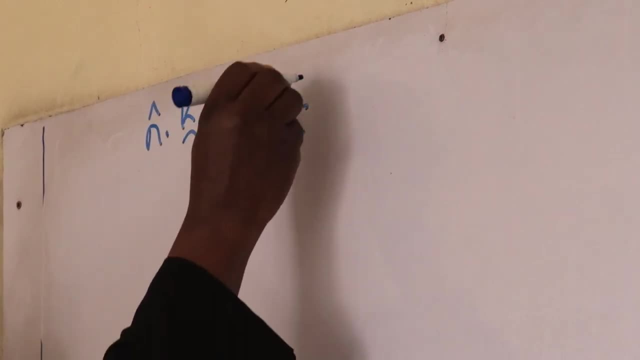 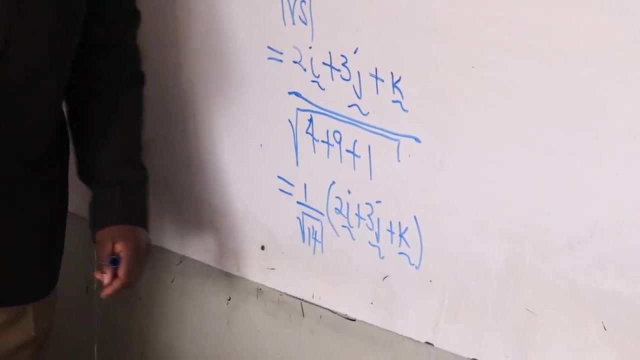 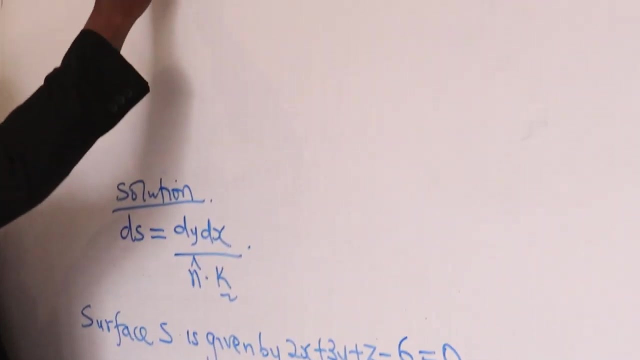 and we get 1.. So now we have nk. Now, when we dot n with k, what is in front of k here is 1.. So it is 1 times this 1 of k, which is just what: 1.. 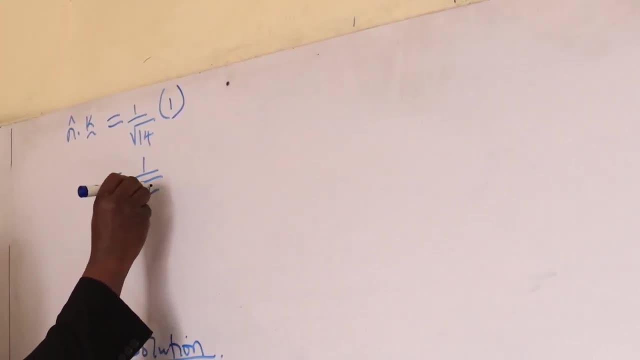 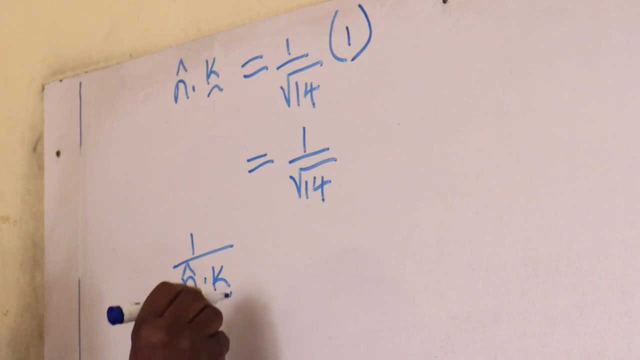 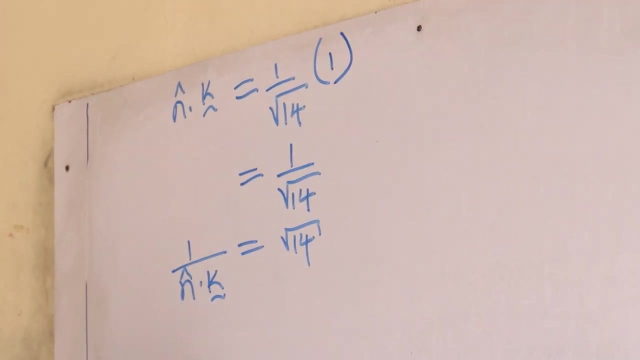 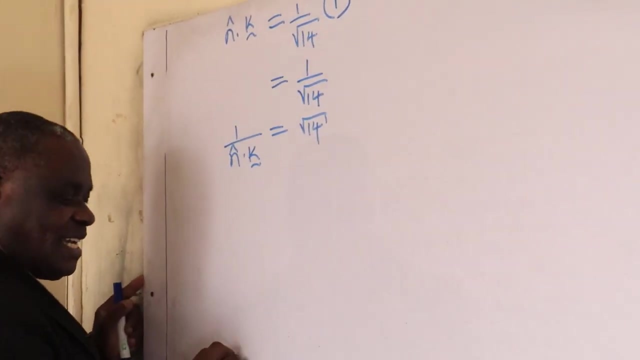 So n dot k is 1 all over root what? 14.. So 1 all over n dot k will simply be equal to root 14. 14. Therefore, we can now be able to write the surface integral. Now our surface. we are going to project it on an xy plane. 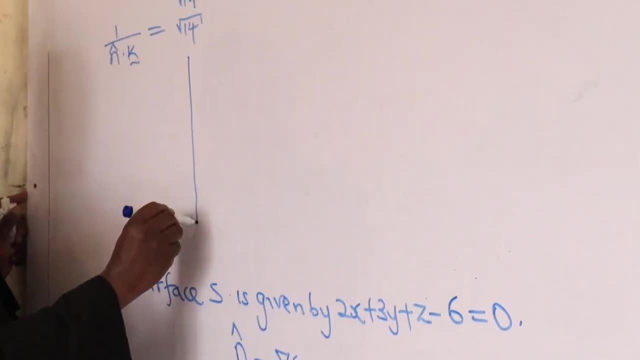 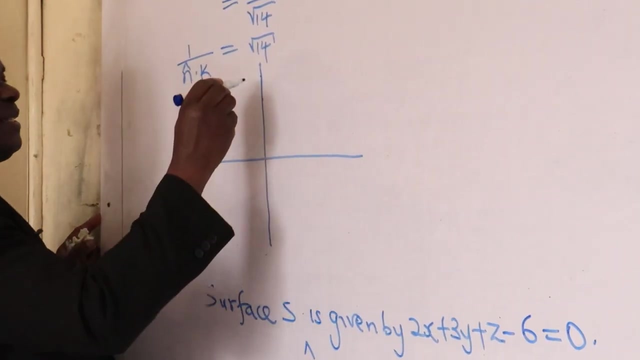 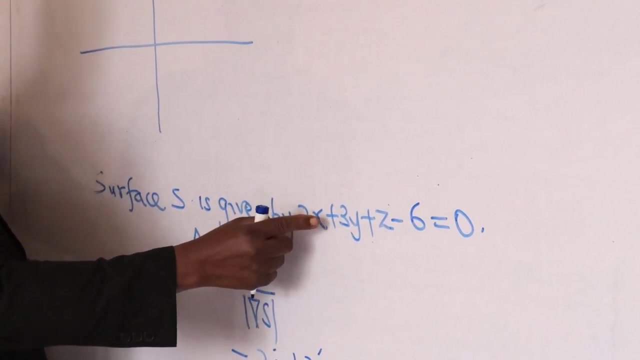 When it is projected on an xy plane, it will create a surface like this: On an xy plane, z is normally equal to 0. So we see, We say, when z is normally 0,, so this one, when x is 0, y will be equal to 2.. 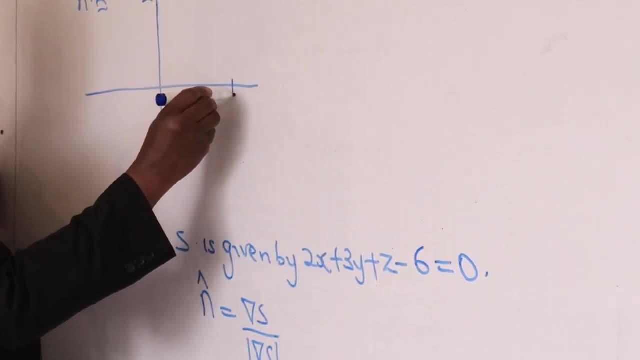 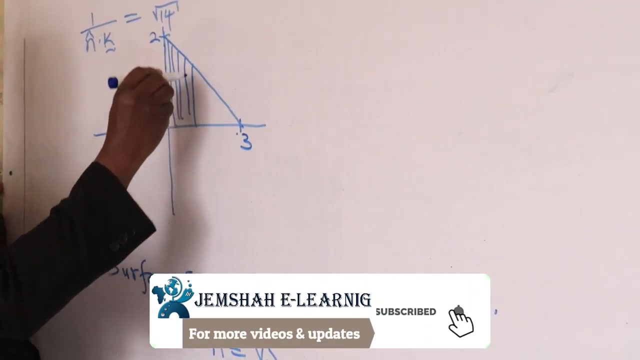 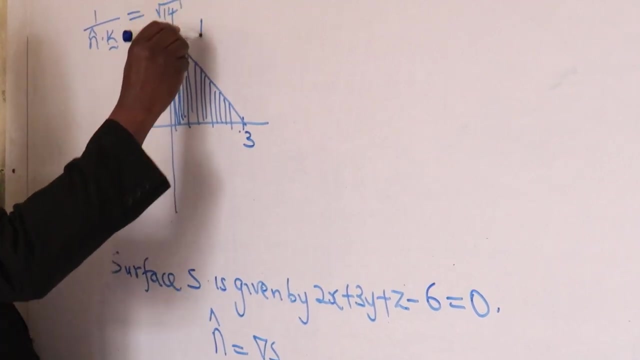 And when y is equal to 0,, x will be equal to 3.. So this is the line, So this is the region, So this is the region, So this is the region. If this is our region, we do a line, what? 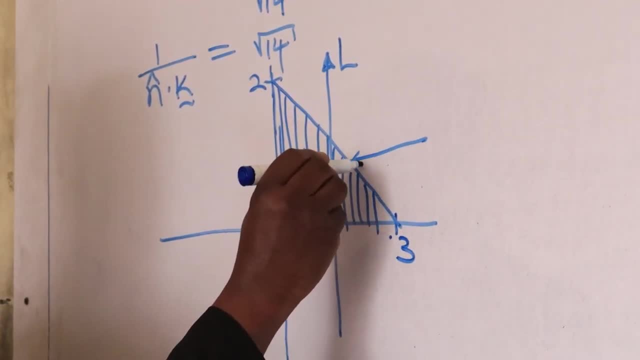 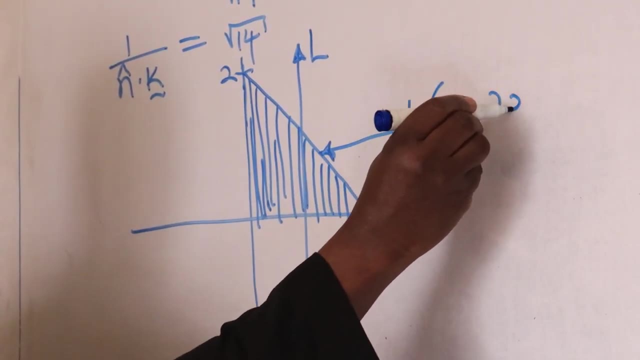 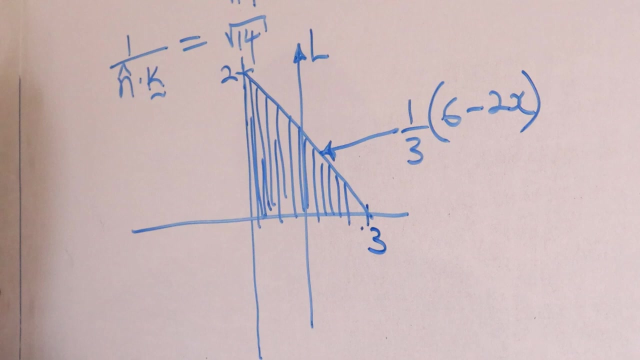 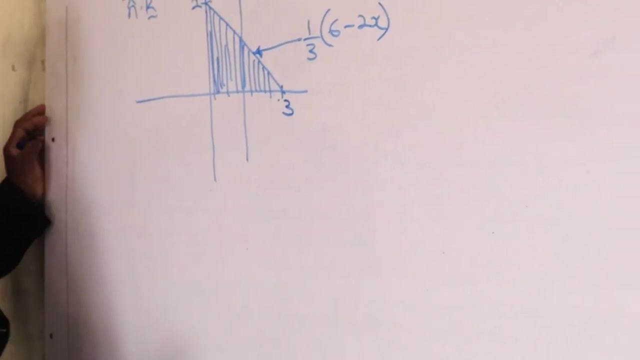 A line m, And the equation of this line is now a third into 6 minus 2x, A third into 6 minus 2x. So from this, from this, we can proceed now. So from this, from this, we can proceed now. 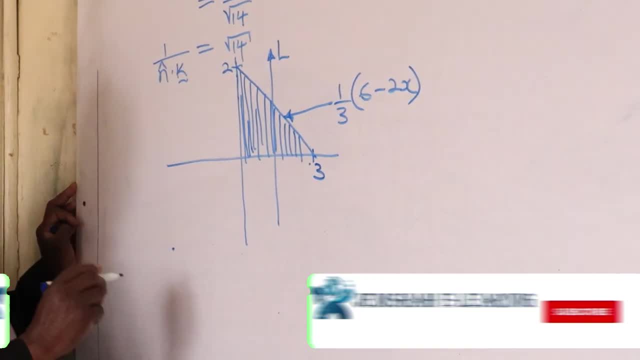 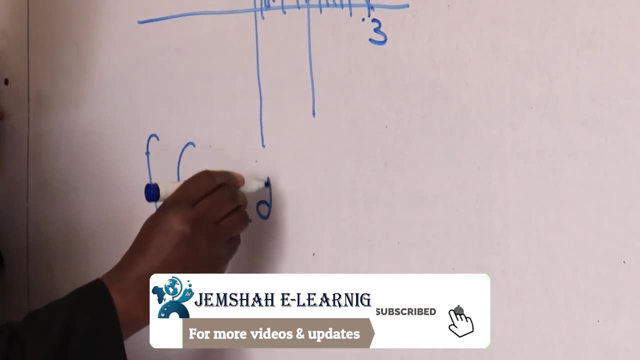 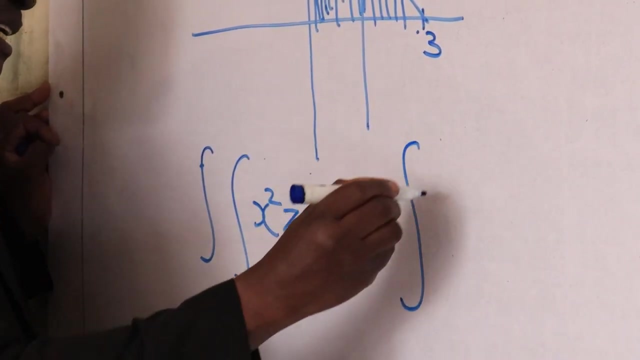 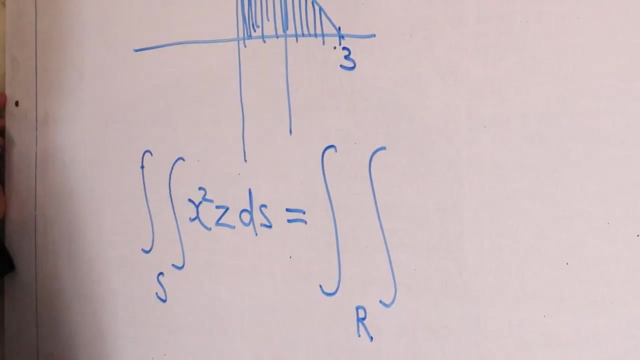 say now, our double surface integral. we are evaluating the integral as x squared z ds. x squared z- ds will be the same as a double integral. we are going to have our region r. this is our region r, where we'll have our limits. we are going to have x squared, then z. 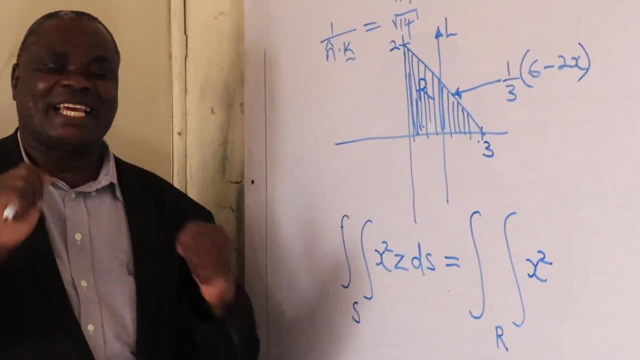 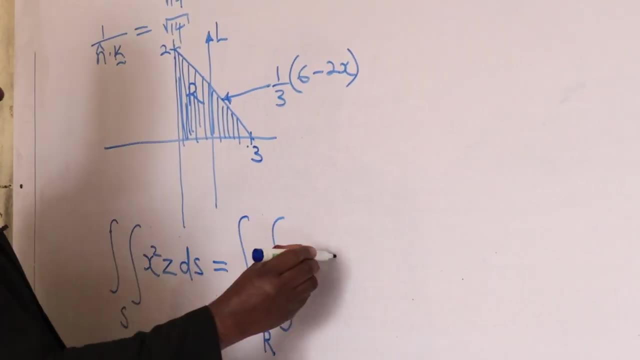 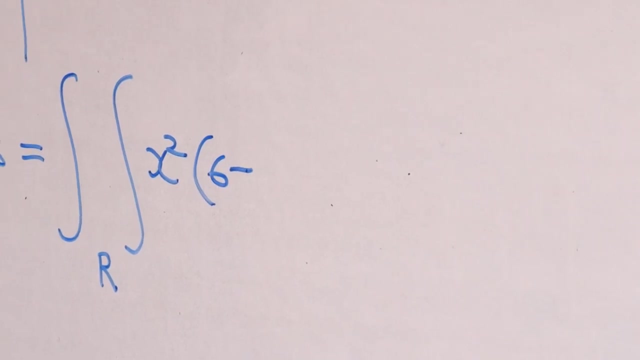 z on that particular surface. how was it related to x and y z? on that particular surface, z was equal to 6 minus z was equal to 6 minus 3y minus 2x. so we replace it where there was z. ds will now be equal to ds will be equal to. 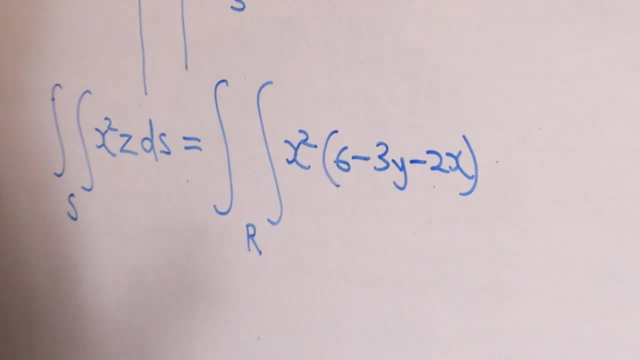 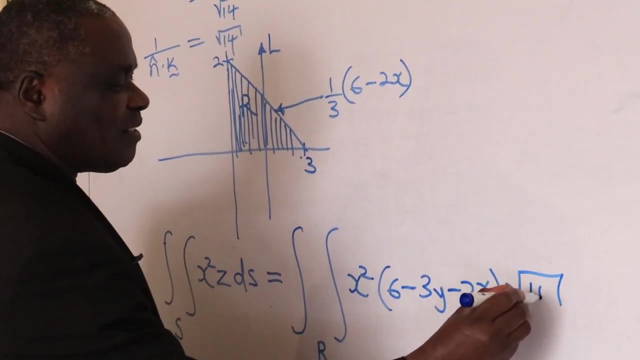 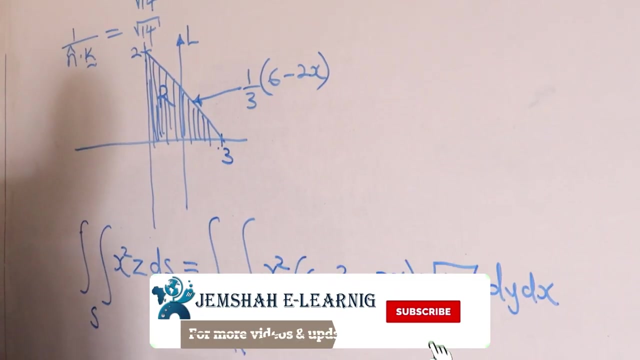 d, y, dx. all over n dot k, n dot 1 all over n dot k is root 14. so we'll be having here root what 14? then dy and dx. now, root 14 is a constant. we take it out. we remain with the double integral. 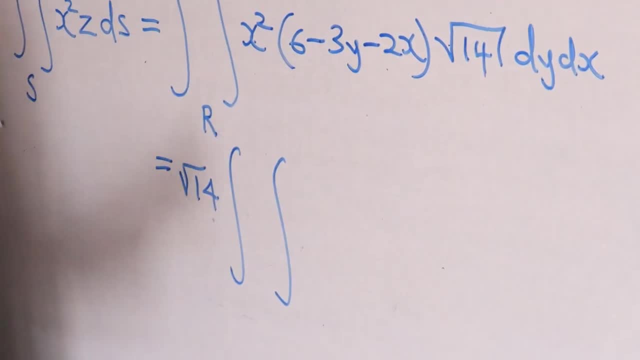 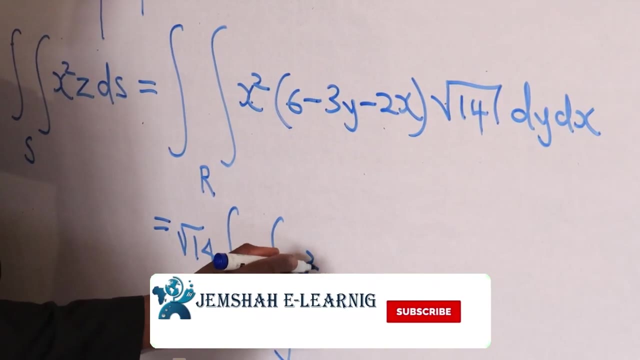 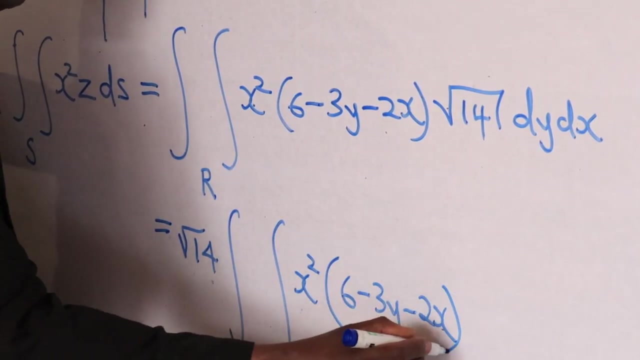 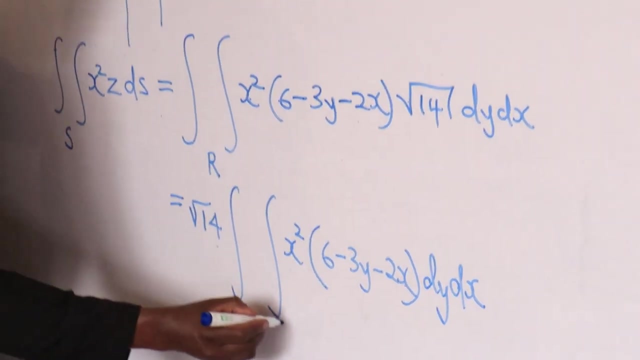 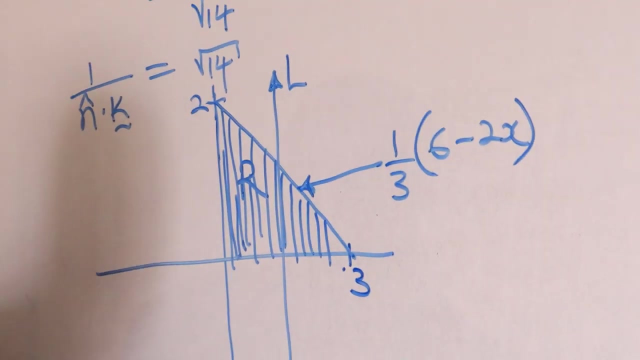 then when we multiply this one out, we can get. now we have a double integral, and we have a double integral. we have x squared into 6 minus 3y minus 2x, then dy, dx, let's insert our limits. as from this region, y will be changing from 0 to a third into 6 minus 2x, and x will be changing from 0 to what? 0 to 3. 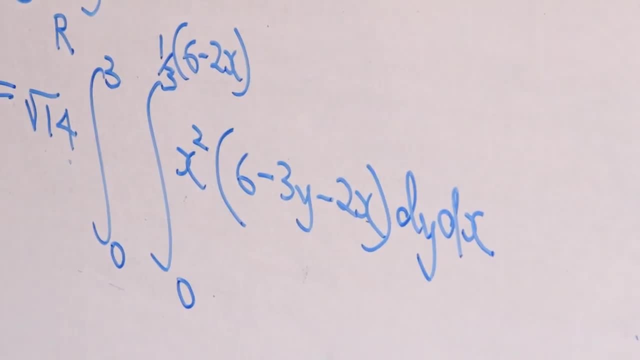 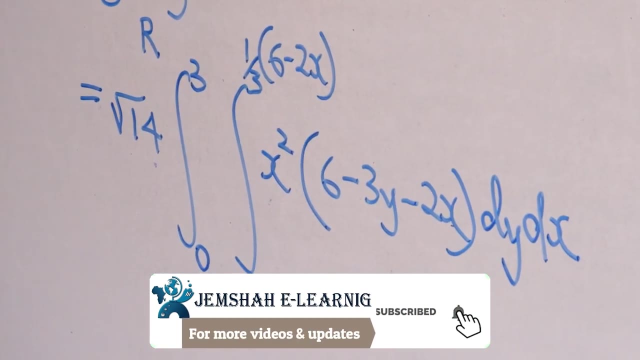 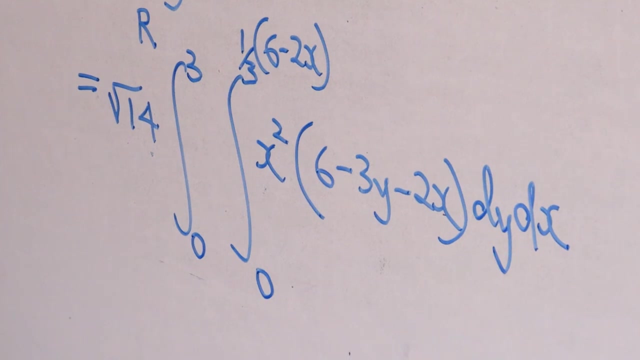 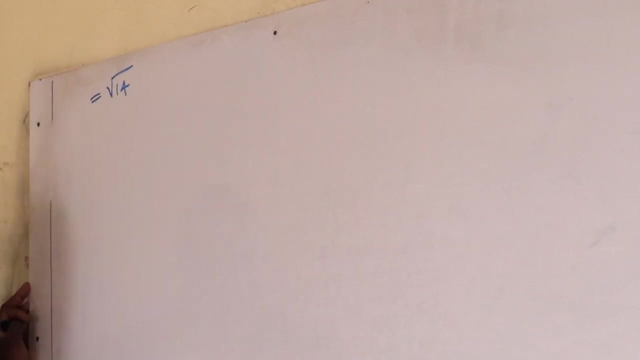 now we should need to poured it in the other side, Ao for this Didr. so this one will be equal to the. so this kin will be equal to root 14, root 14. we are integrating, let N turn off. we are integrating, let N turn off. 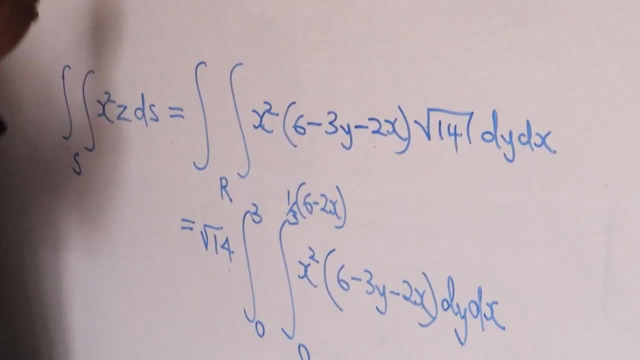 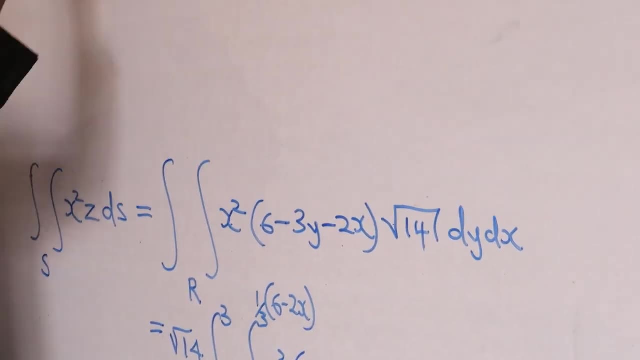 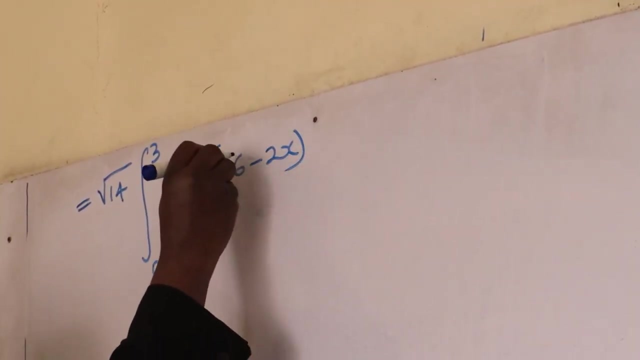 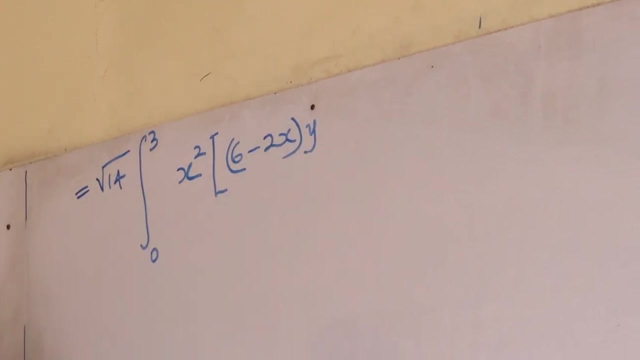 from correct. From 0 to 3, x squared is kept with this constant by that particular time. So we'll be having a scenario in a bracket: 6 minus 2x is also a constant. When integrated, you get what You have, the constant multiplied by y, because we are integrating with respect to y first. 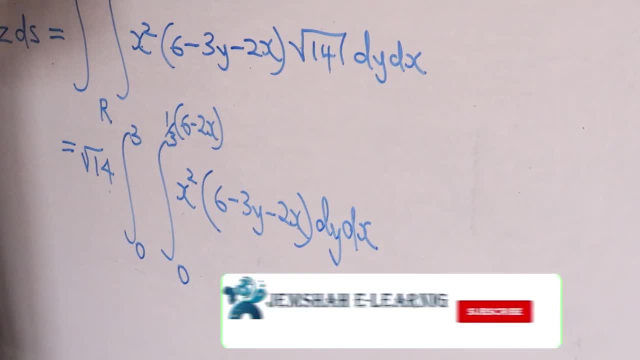 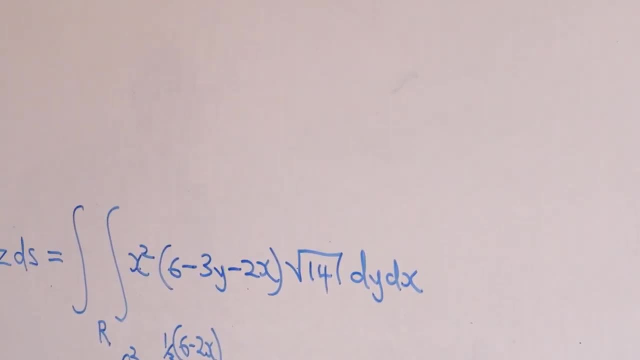 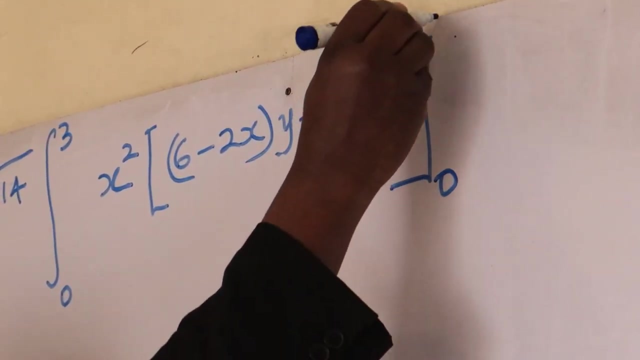 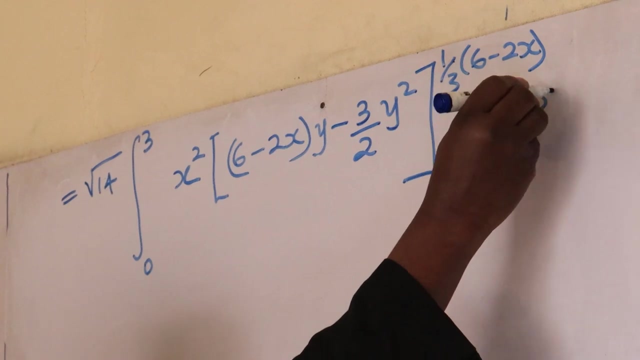 Now minus 3 all over 2, then y squared. minus 3 all over 2, y squared. And now we put our limits from 0 to a third 6 minus 2x. then we remain with the dx. 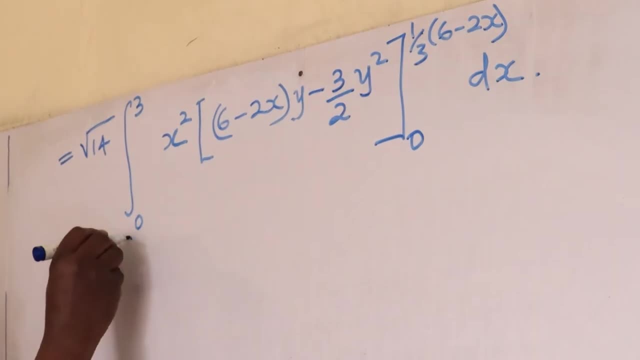 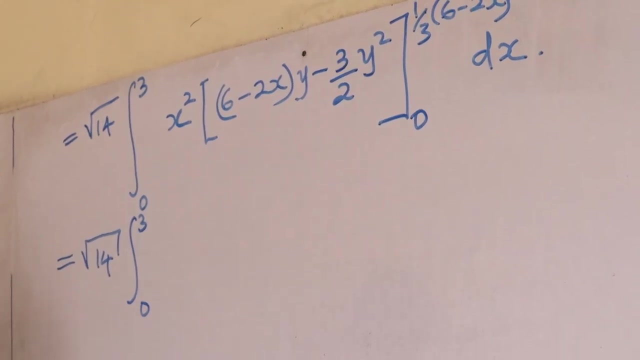 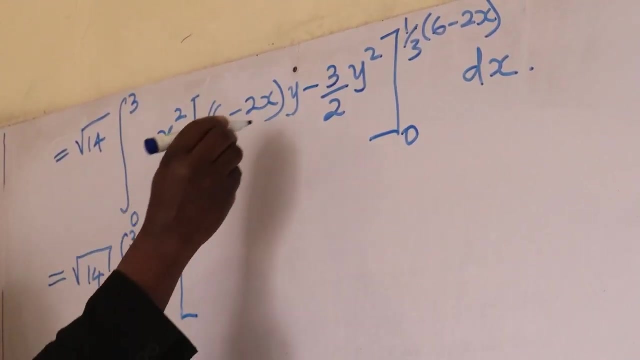 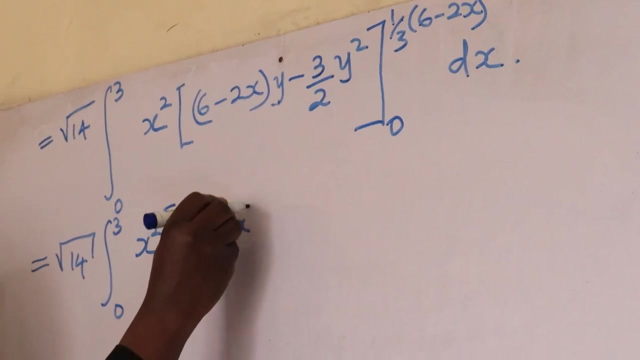 So this will be root 14.. Okay, 0 to 3,, 0 to 3,, 0 to 3.. Now we are substituting for, we are substituting for y, So this one will be a third into 6 minus 2x, which will have been a square, squared minus. 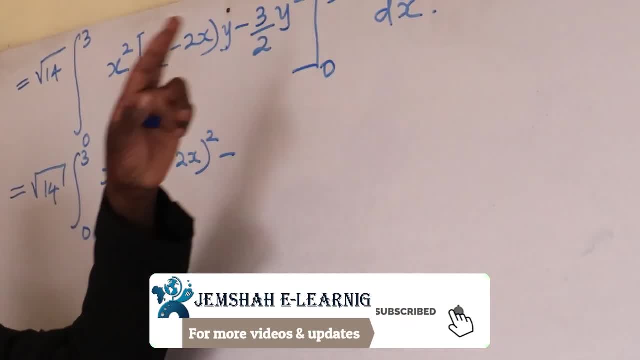 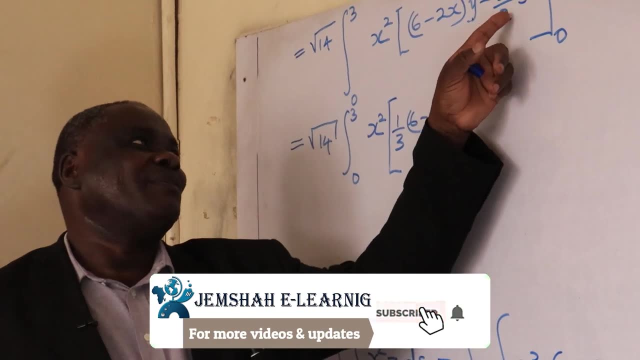 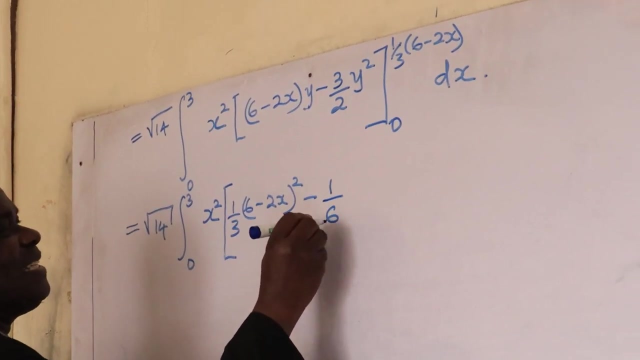 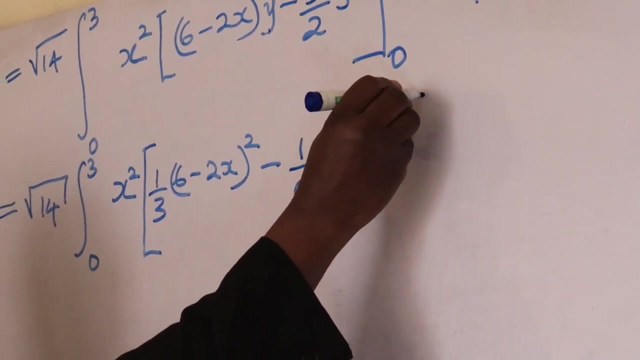 We are inserting this. A third squared will give you 1 all over 9.. 1 all over 9, 2 times 9 is 18,. 3 all over 18 is 1 all over 6,. 1 all over 6, into 6 minus 2x, which will have been a square squared. 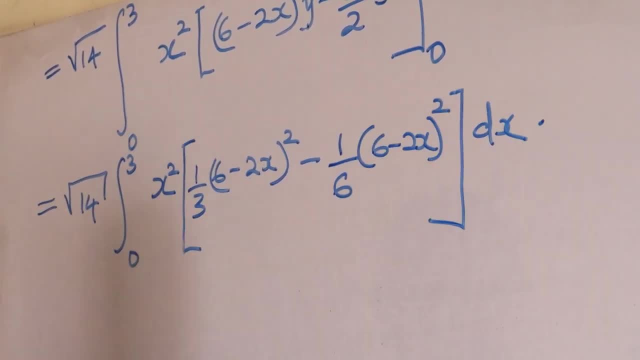 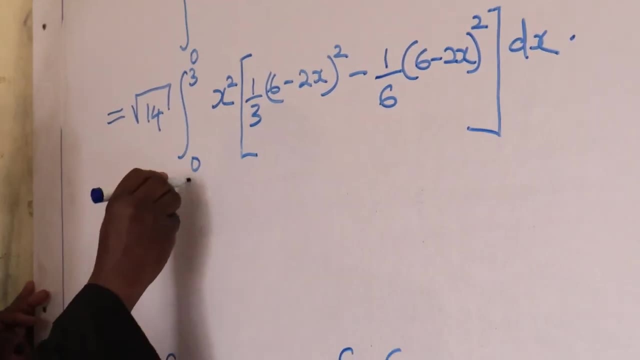 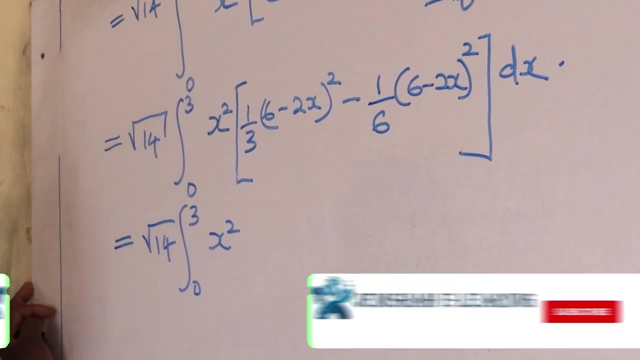 So that is it. Then here we have dx. we have that one as dx, Which gives us root 14, 0 to 3, x squared, A third minus 1 over 6, we get 1 over 6.. 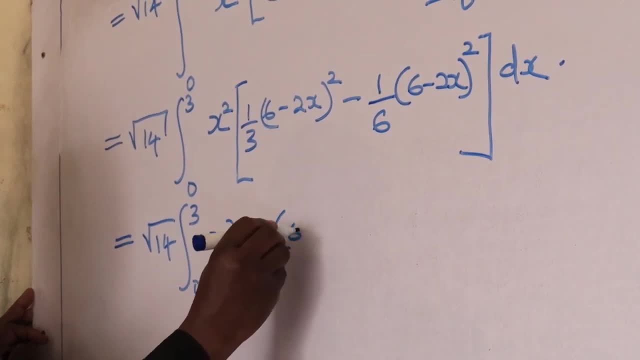 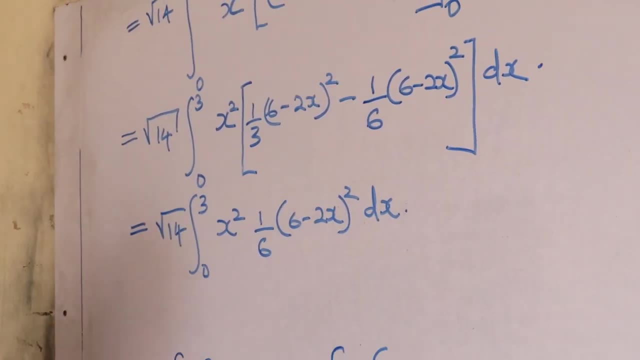 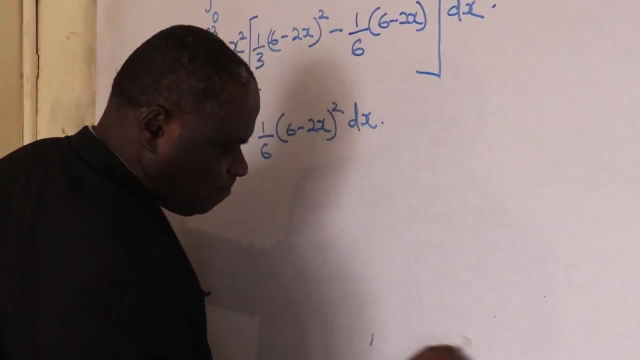 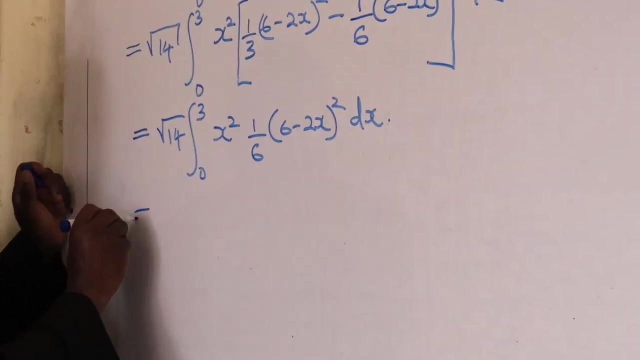 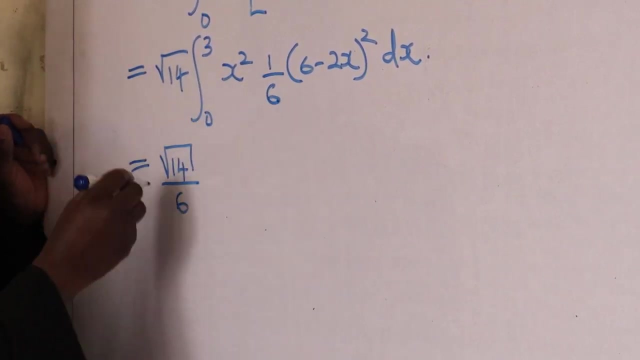 So we'll be having 1 over 6, into 6 minus 2x, which is square squared. Then we have our dx dx. So this will be root 14, all over 6.. We take dx out, we have 0 to 3, we expand this other part, 6 minus 2x, which will bring 36, minus 24x. 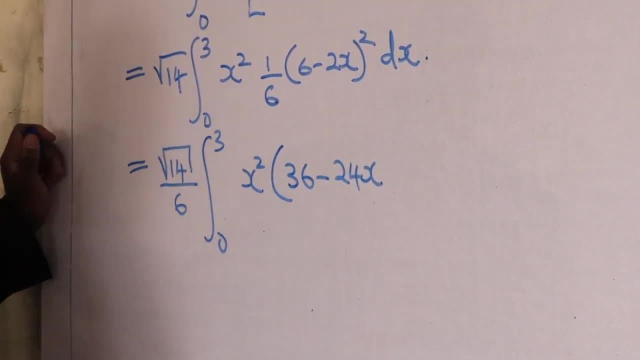 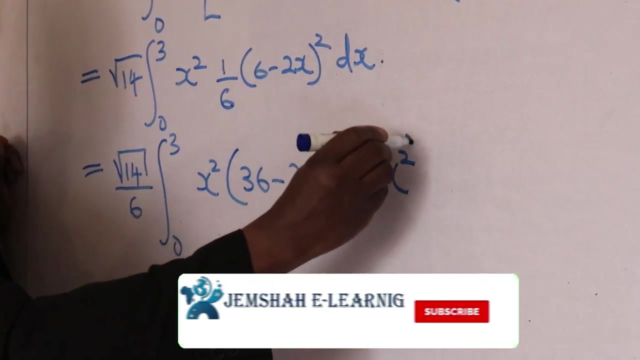 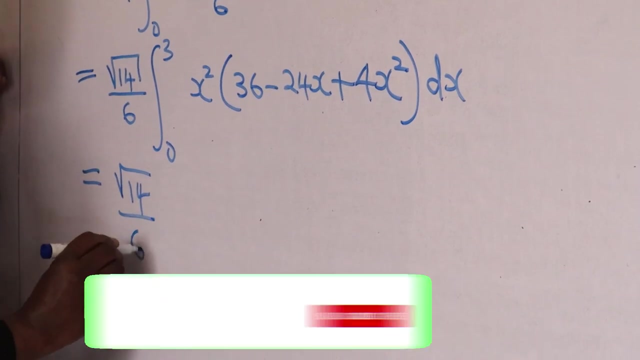 Minus 24x, Minus 24x. Mmhmm, Plus 4x squared, 4x squared. Oh the x. We simplify still Root 14, all over 6. 0 to 3.. 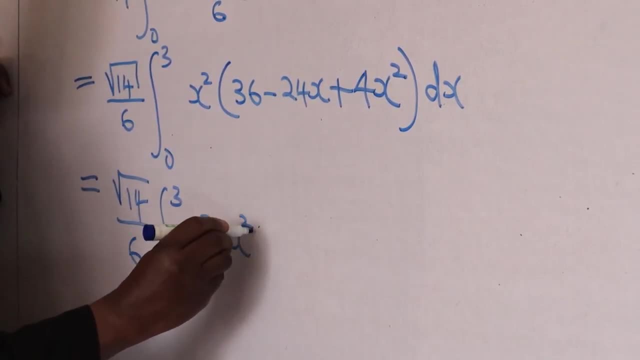 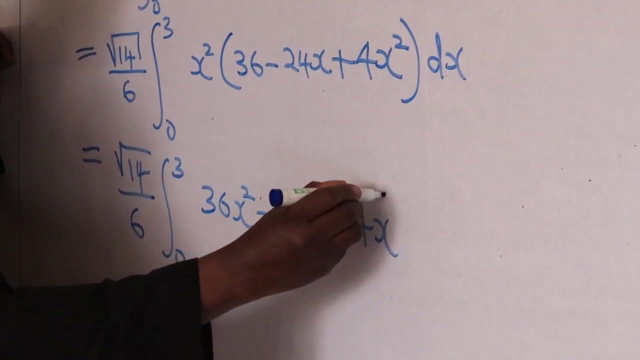 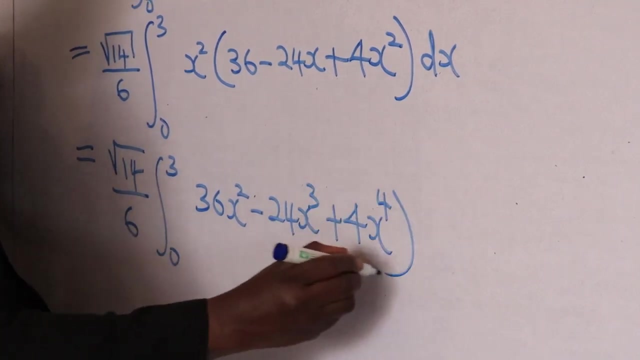 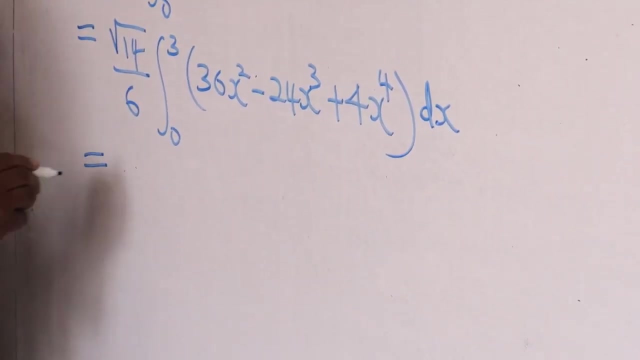 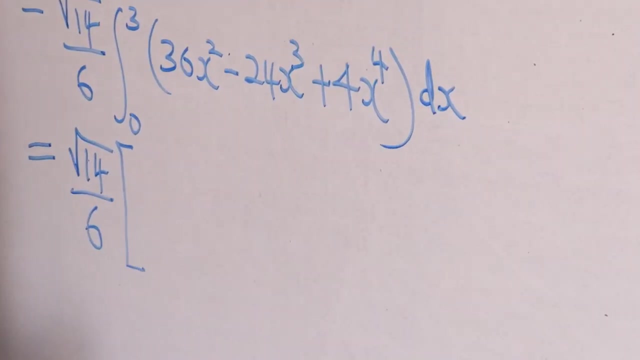 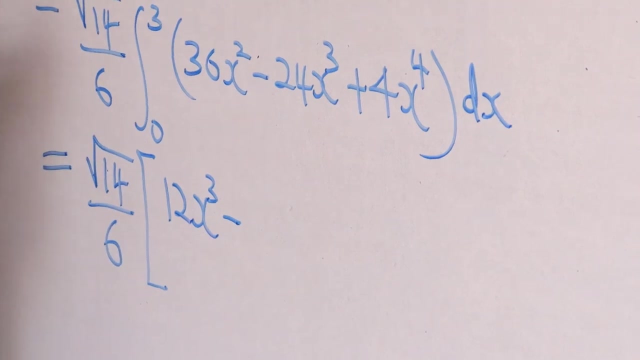 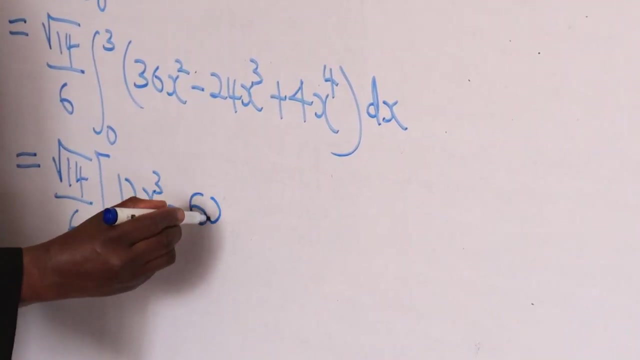 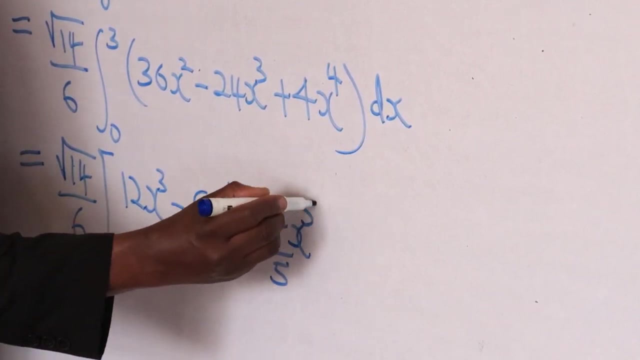 This will be 36x squared Minus 24x cubed, plus 4x power 4.. Now everything integrated with respect to x, This one simplifies to root 14 all over 6.. We are now integrating. we get 12 of x cubed minus 6x power 4, plus 4 all over 5, x power 5.. 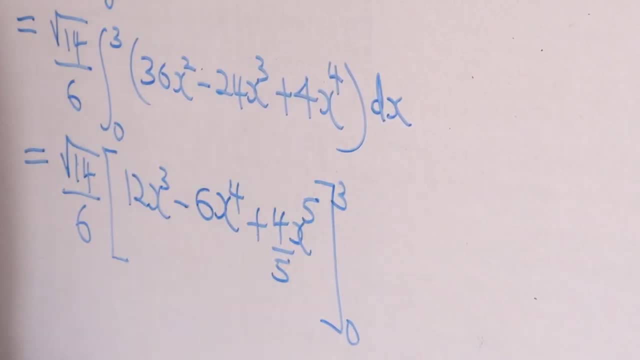 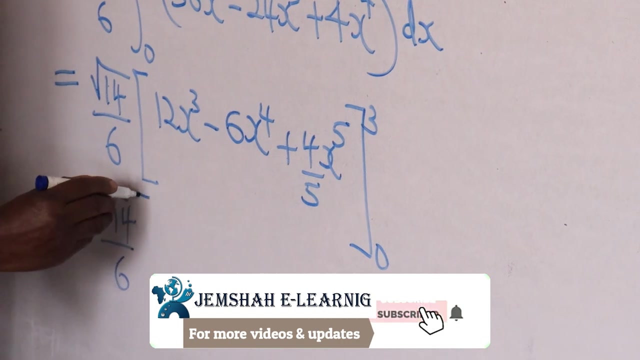 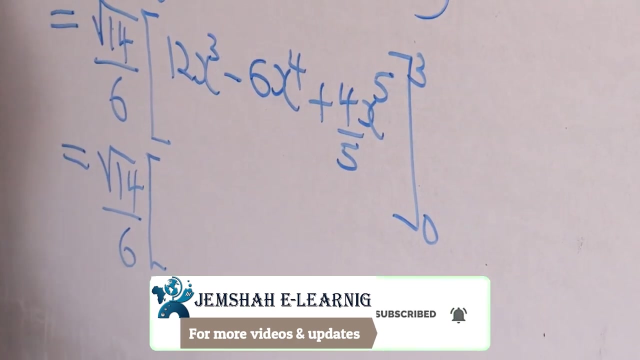 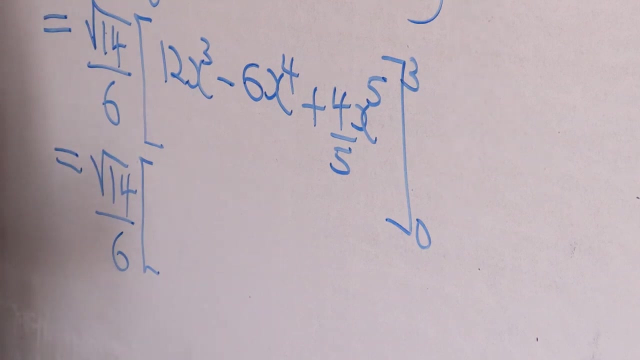 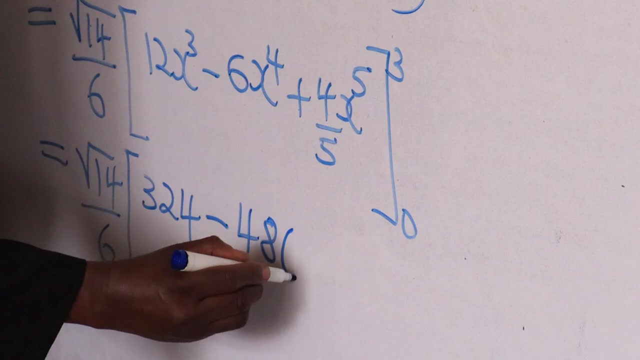 Now we have limits here: 0 to 3.. Which will be equal to root 14 all over 6, into 3 cubed is 27,. 3 cubed is 27, 27 times 12.. 27 times 12 will be 86.. 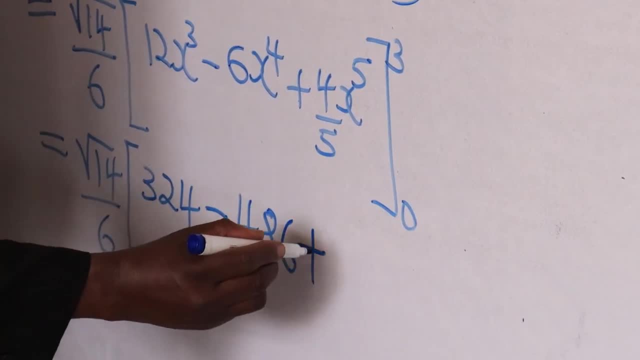 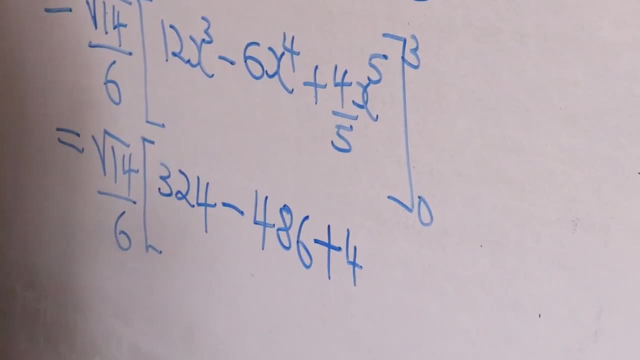 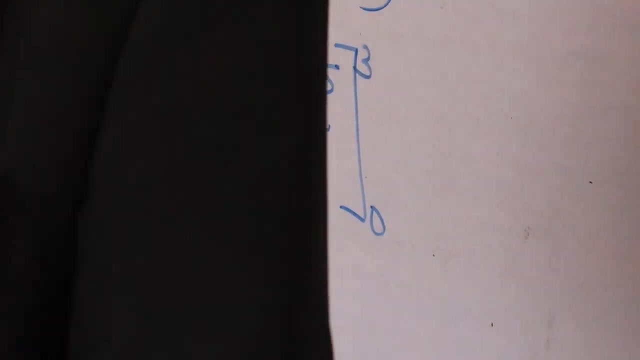 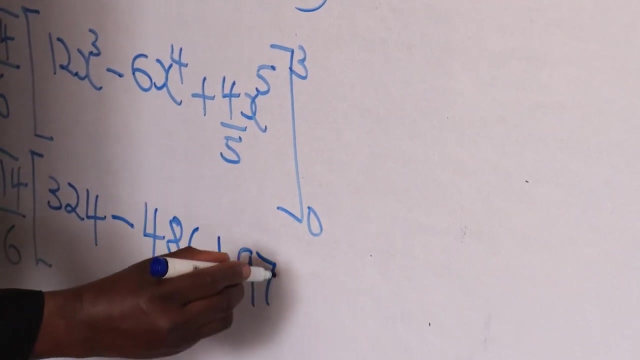 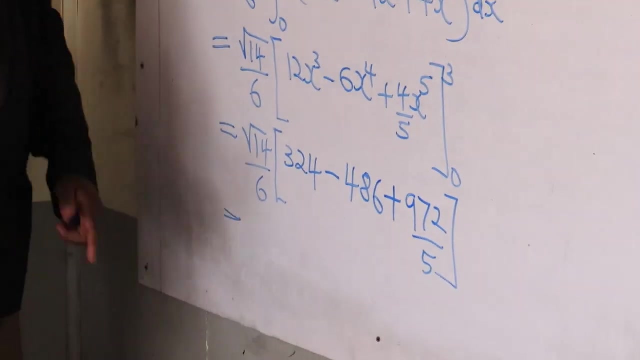 486, plus 3 power 5,, that is 243, 243 times 5, 243 times 4, 972, all over 5.. From there let's do the addition. What do we have inside the bracket? 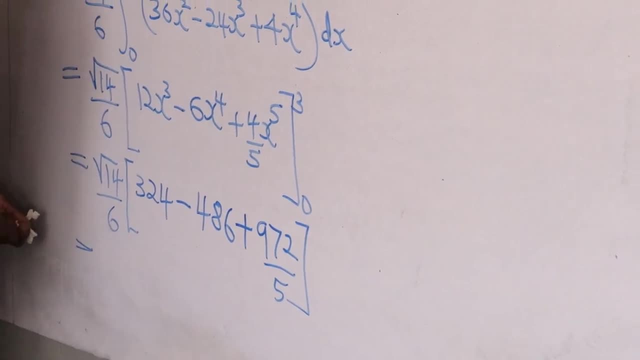 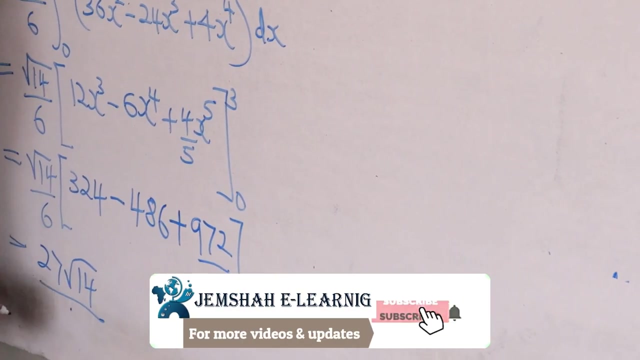 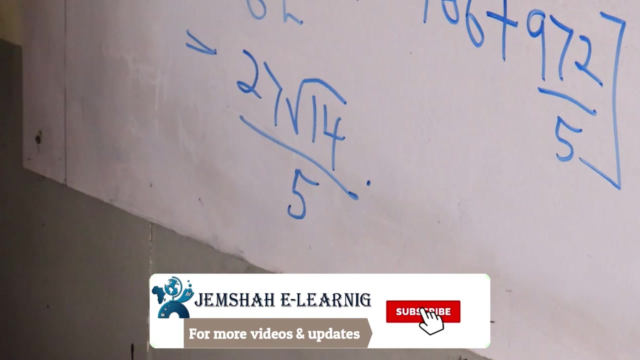 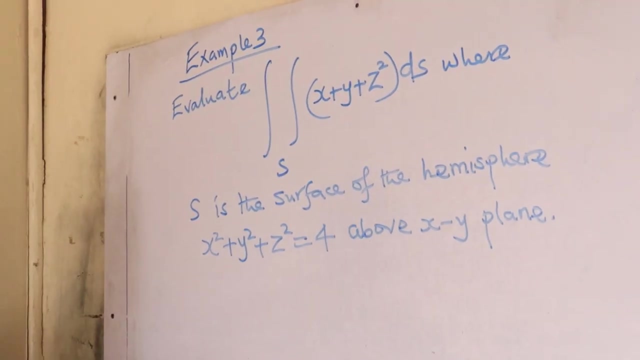 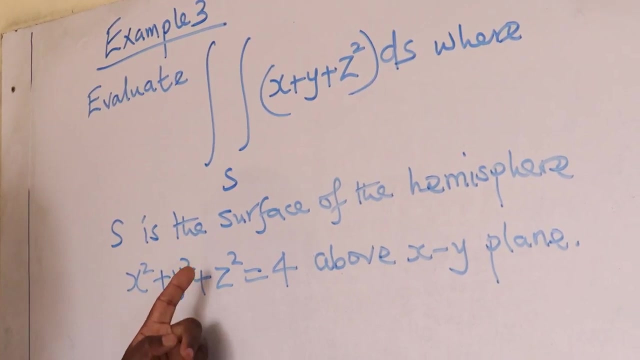 So the final answer here will be 27, root 14, all over 5.. Root 14, all over 5.. That will be the final answer. So in our example 3, we are evaluating a surface integral where this is the surface of the hemisphere: x squared plus y squared plus z squared is equal to 4, above x y plane. 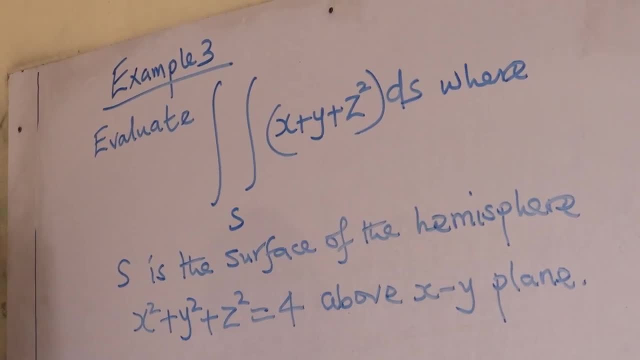 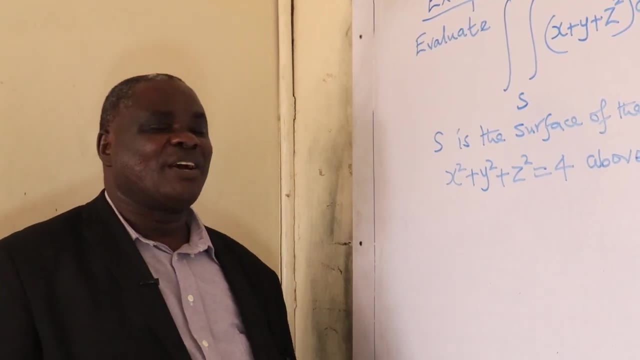 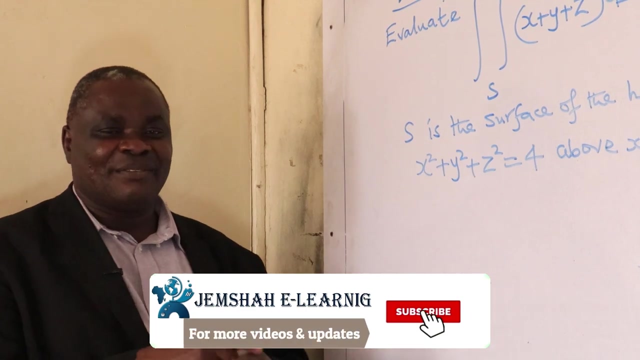 Now, in this particular connection, our ds, because this is a spherical surface- we can convert our ds directly into spherical coordinates. We can do that. We can do that one directly, So we'll not have, there is no need of doing what. 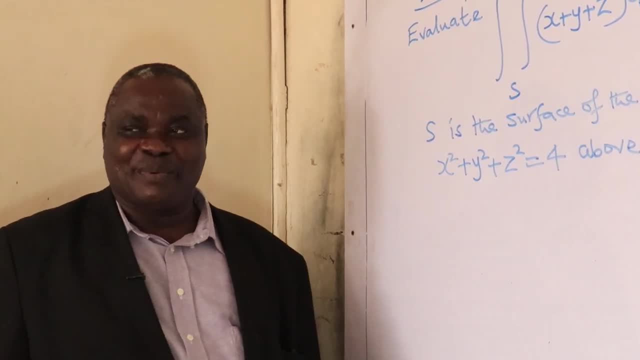 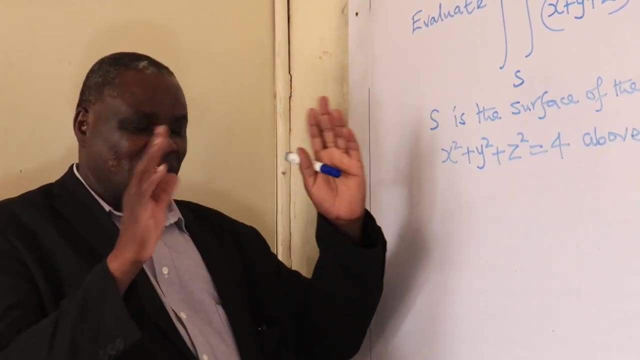 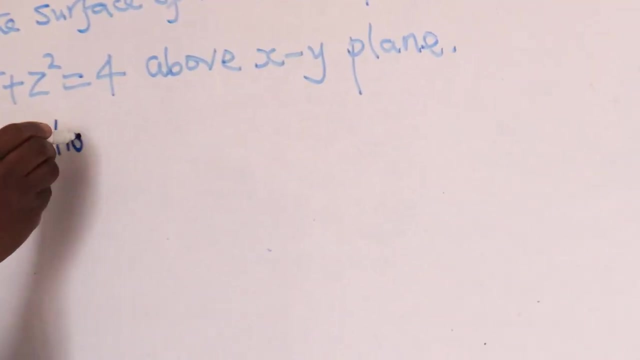 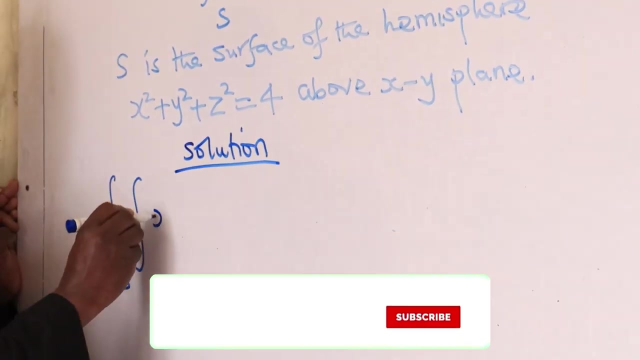 Of projecting our surface onto x, y plane, Because in spherical coordinates ds can be written, And when it is written it will simplify all the operations. So we say in our solution: the integral, integral, integral ds, x plus y plus z squared ds. 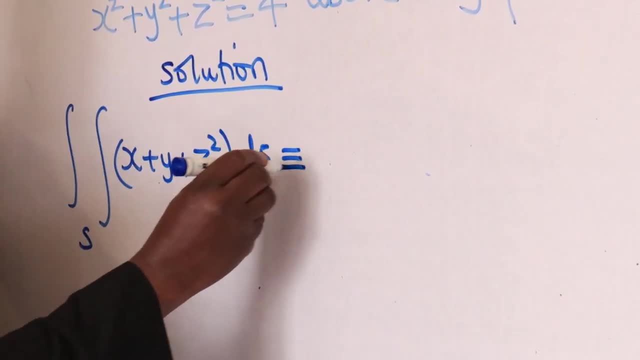 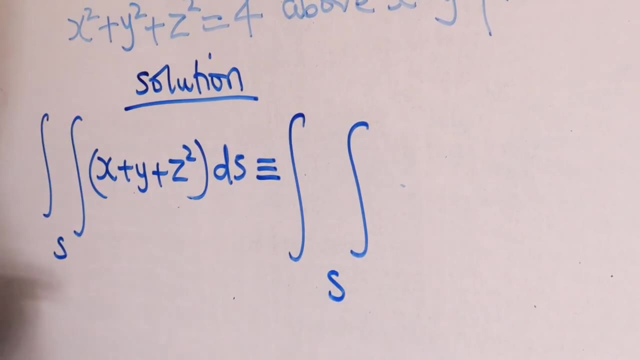 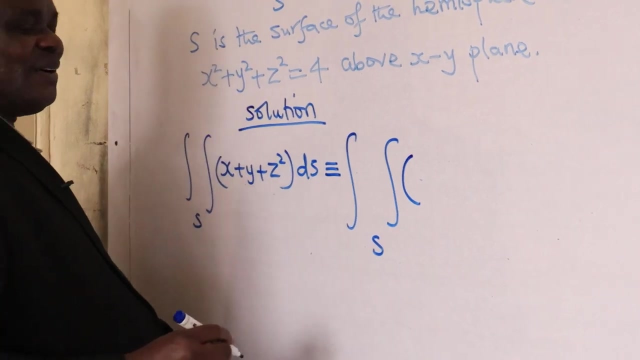 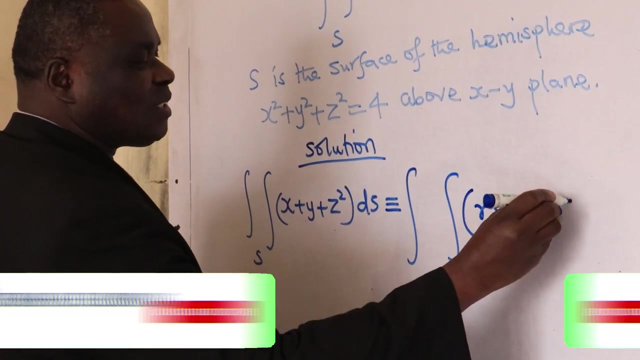 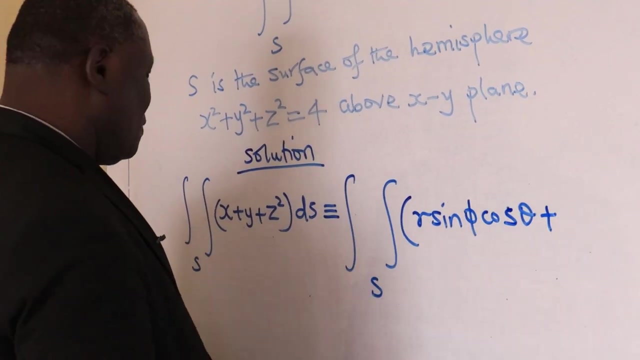 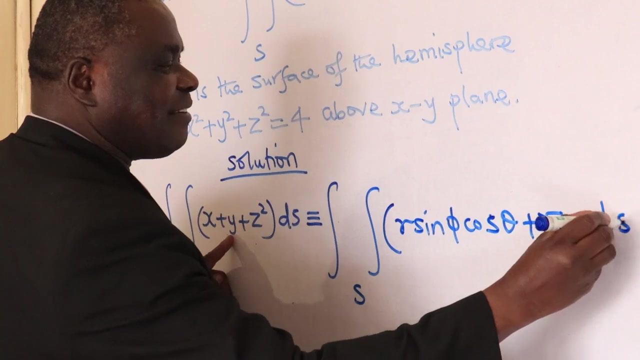 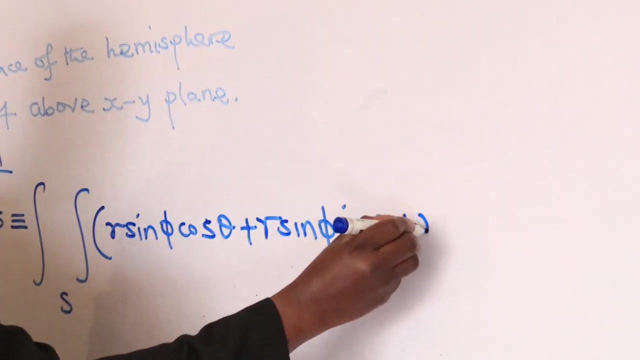 Will be equal to or equivalent to double integral Limits will still come from the surface. Now we put x into spherical coordinates. x in spherical coordinates will be equal to r sine phi cos theta plus y. r sine phi sine theta plus z squared, which we will now read: r, r squared. 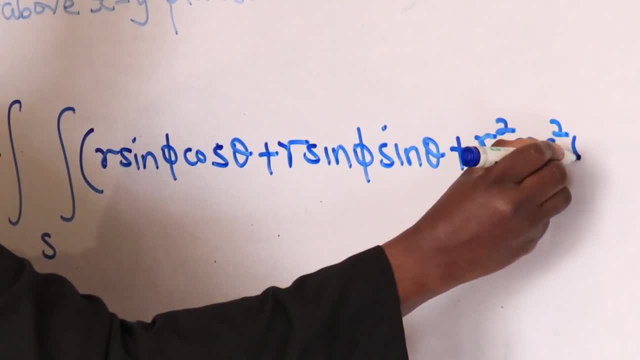 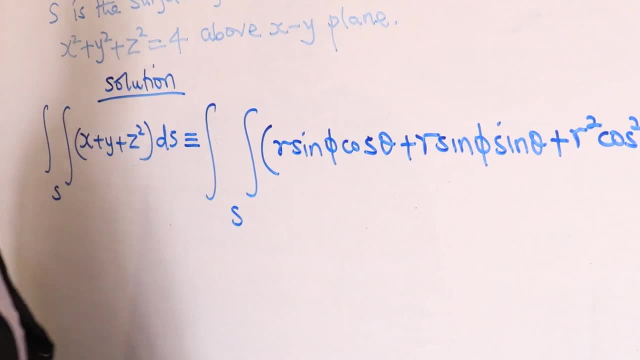 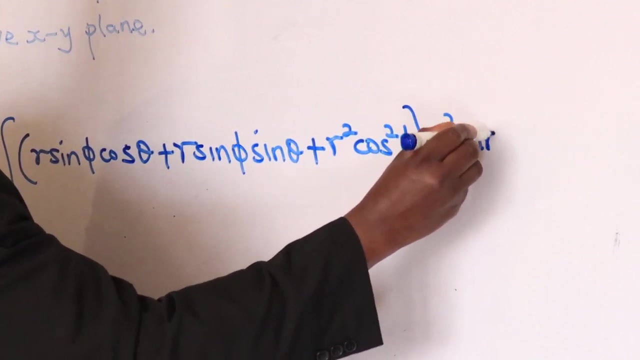 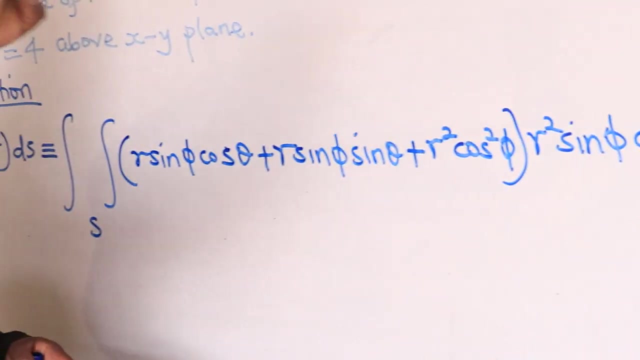 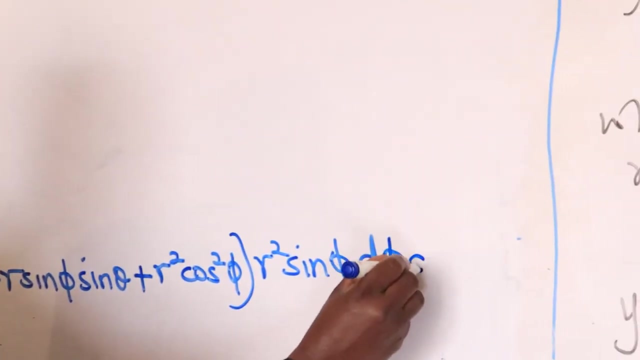 cos squared cos squared phi, r squared cos squared phi, And our ds now becomes r squared sine phi d. on that surface of the sphere, r is not changing. so what is changing is only what. It's only phi, and then theta. 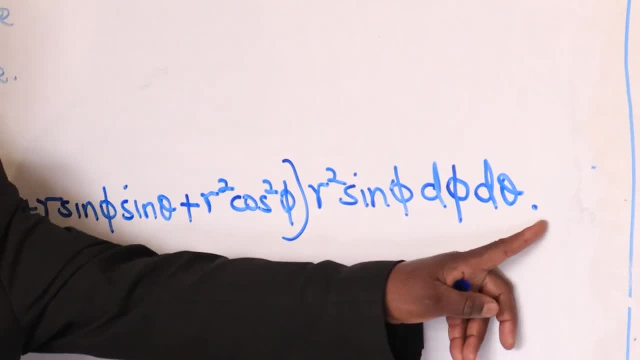 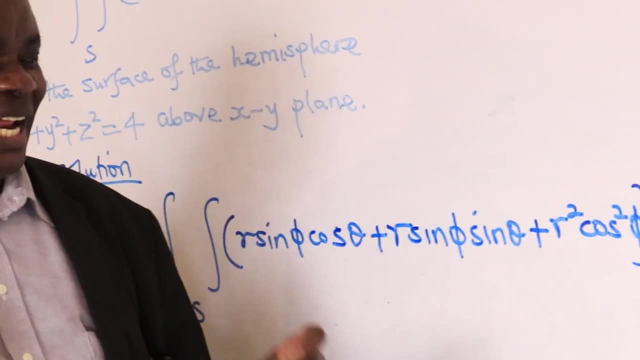 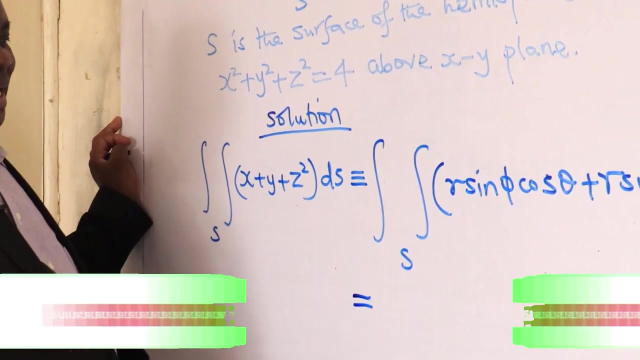 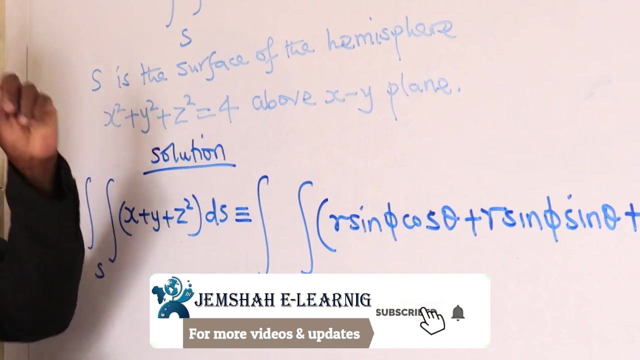 So the whole of this stands in for our ds. This is according to our analysis or analogy on spherical coordinates. So this one but r, since it is constant, and this is a sphere of radius 2.. Whatever we are having here, It's a sphere of radius 2.. 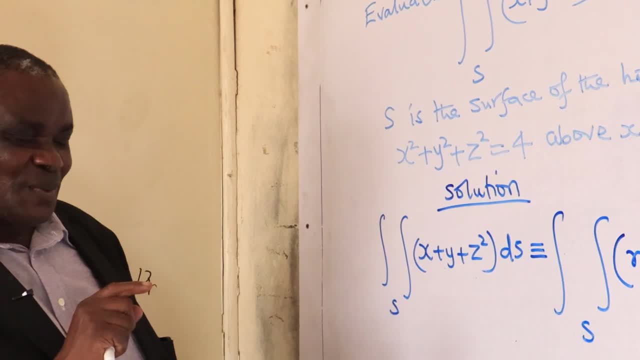 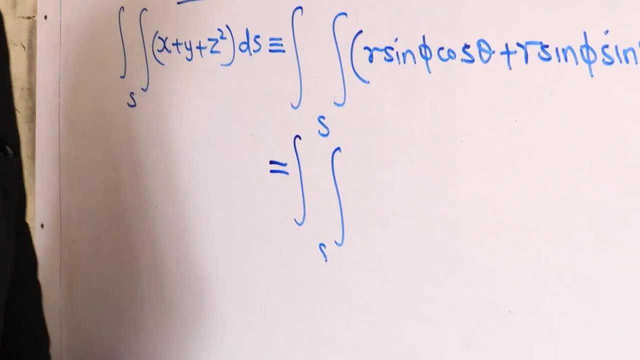 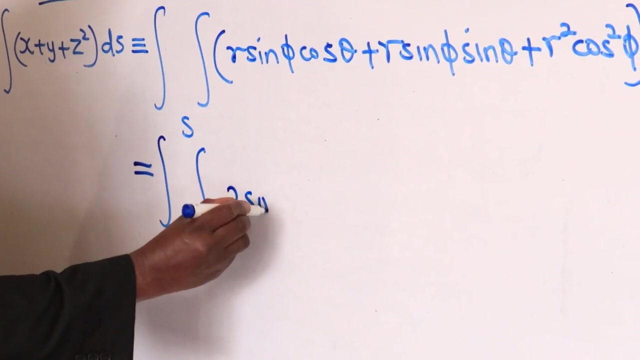 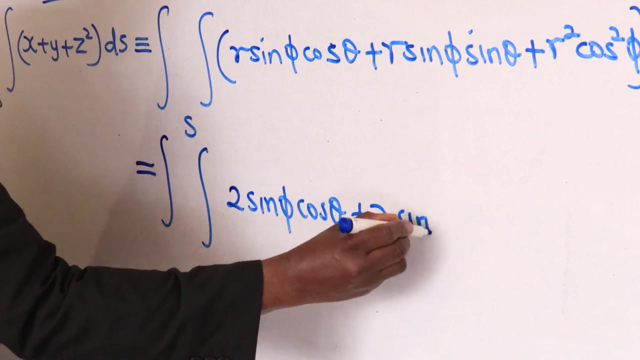 So where there is r, we are going to insert 2.. So this will be a double integral, still on surface s, but we are going to input now our limits. This is r, r is 2, 2 sine phi cos theta plus 2 sine phi sine theta. 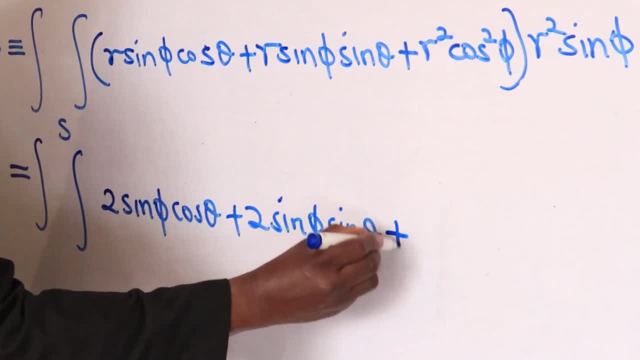 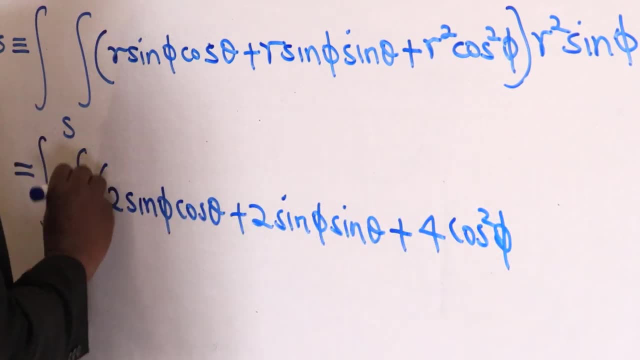 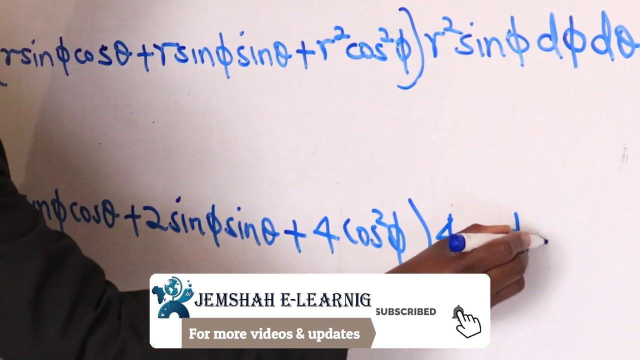 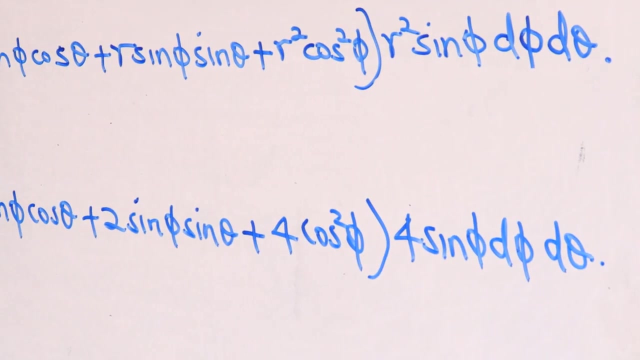 So r is 2, 2 sine phi cos theta plus 2. sine phi sine theta Plus 4, cos squared phi Everything multiply 4, sine phi d phi d theta. Now r phi is changing from 0 to pi over 2.. 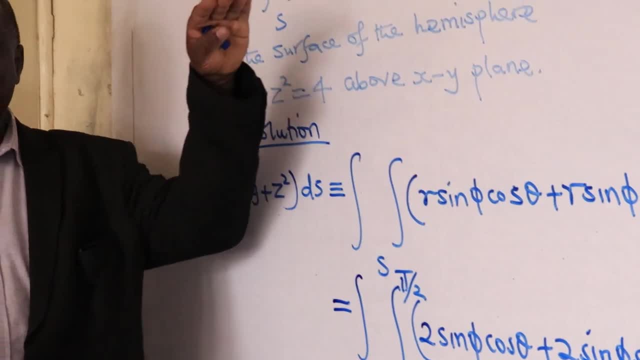 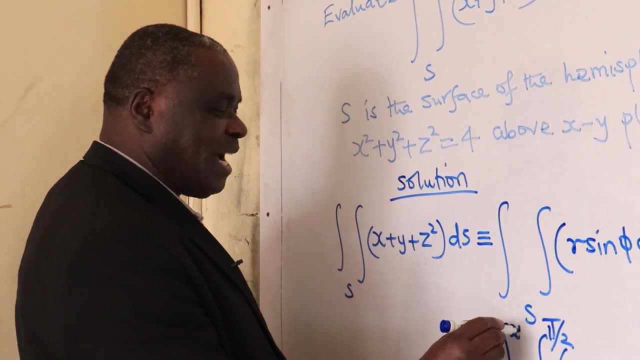 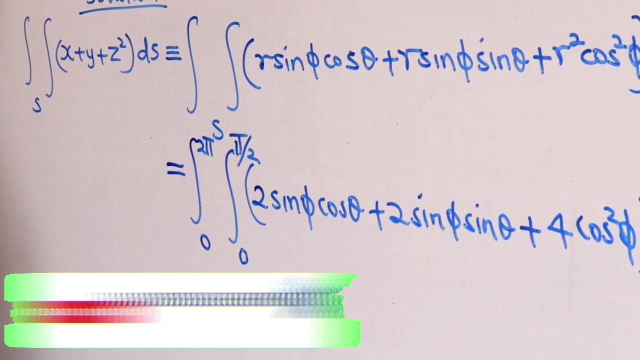 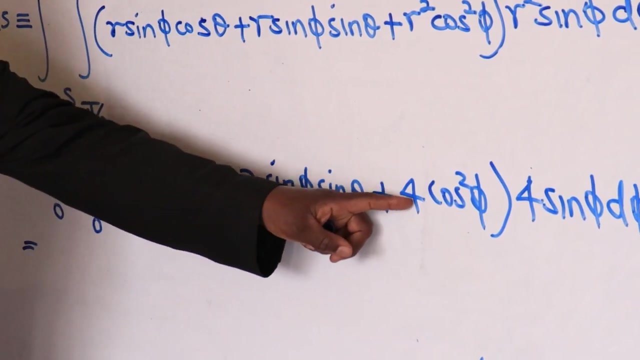 Since this is what A hemisphere above x, y plane And our theta will be changing from 0 to 2 pi, 2 pi, 0 to 2 pi. So from this we can see there is something common. 2 is common in each and every part inside here. 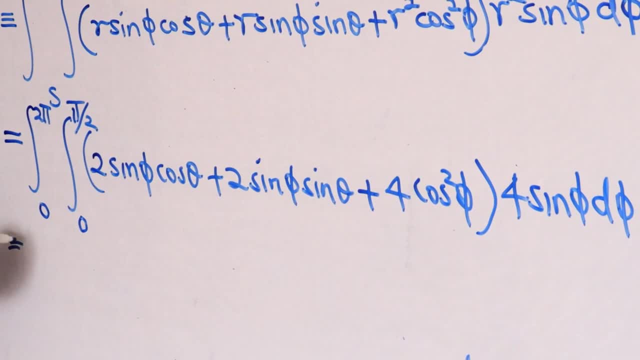 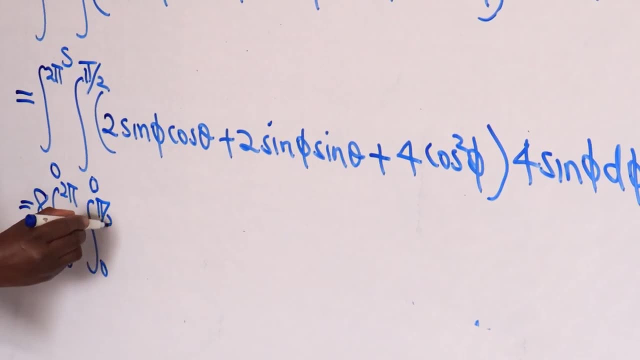 And 4 is multiplying those. So 2 times 4 is 8.. We take it out. We say 0 to 2 pi, 0 to pi all over 2.. What remains now will be: The 4 is already out. 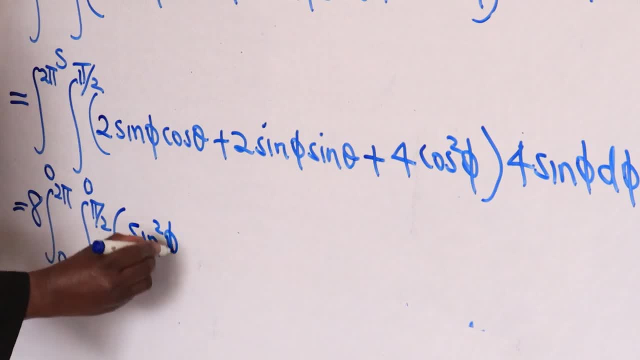 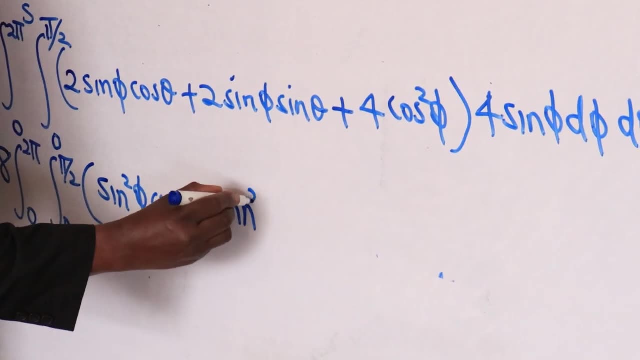 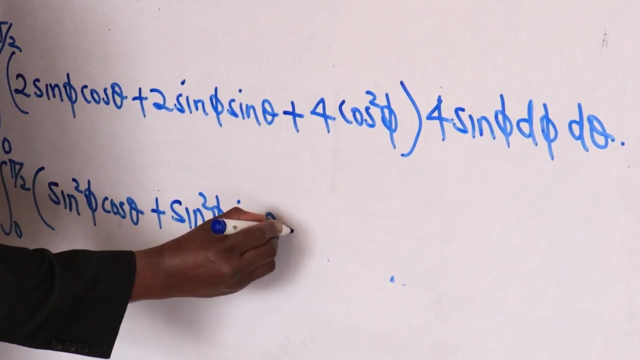 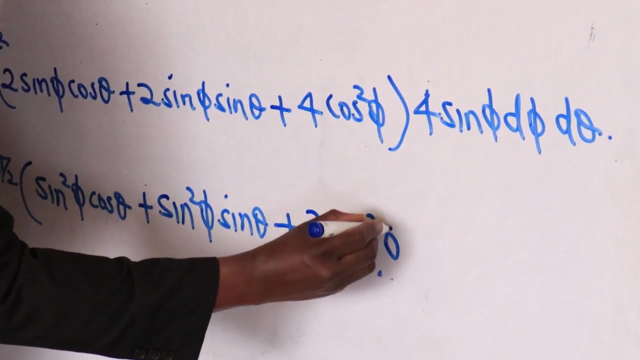 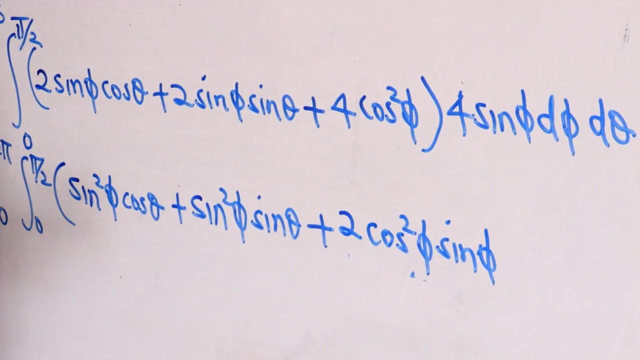 We will be having sine squared phi cos theta Plus, sine squared phi sine theta Cos theta Plus. there is a 2 that has remained here, 2 cos squared phi sine phi, Cos squared phi sine phi. Then we have here d phi. 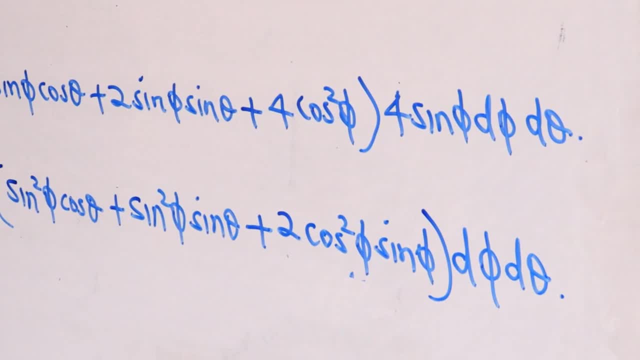 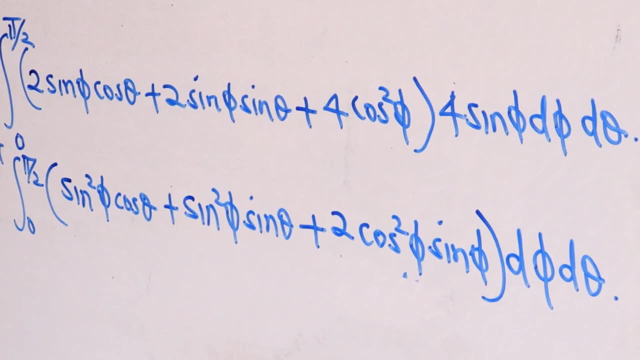 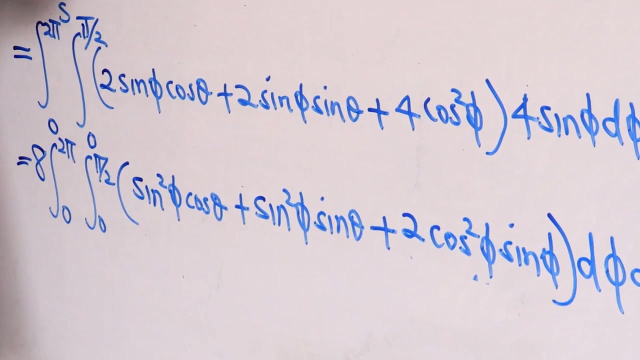 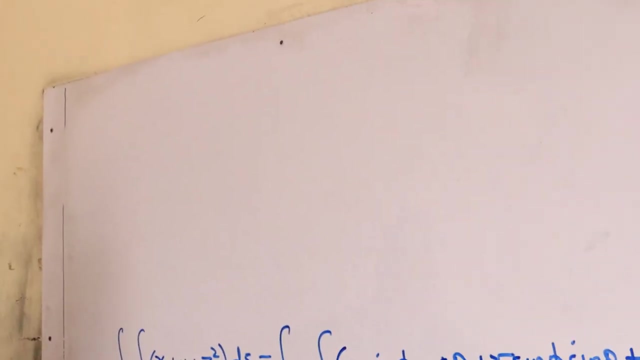 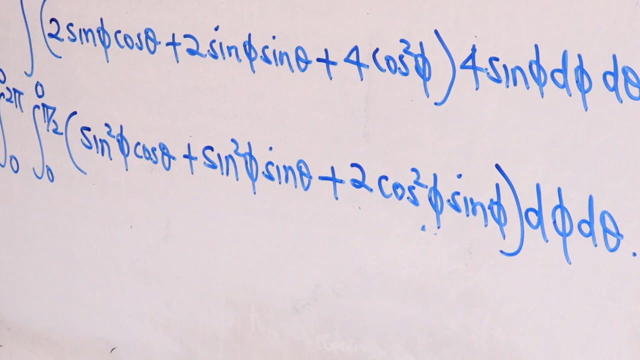 d theta, d theta. We have there d phi d theta. So we proceed with our evaluation. Proceed with our evaluation. Now we are integrating with respect to phi first. So this one will be equal to 8.. The integral is 0 to 2 pi. 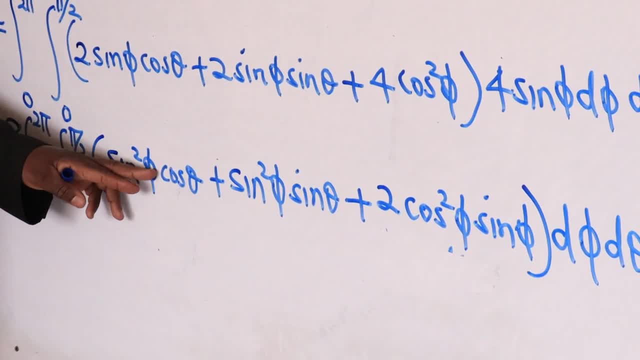 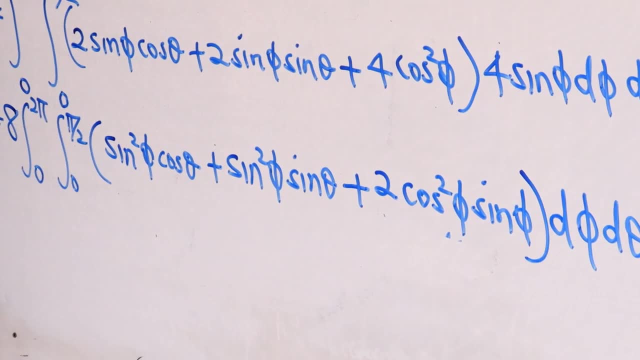 When you integrate sine squared phi With respect to from 0 to pi all over 2.. We can use the Wally's formula. We can use the Wally's formula, Or we can just put it in general, If this one is integrated. 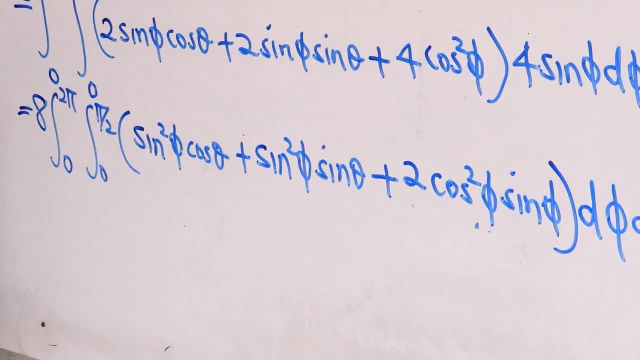 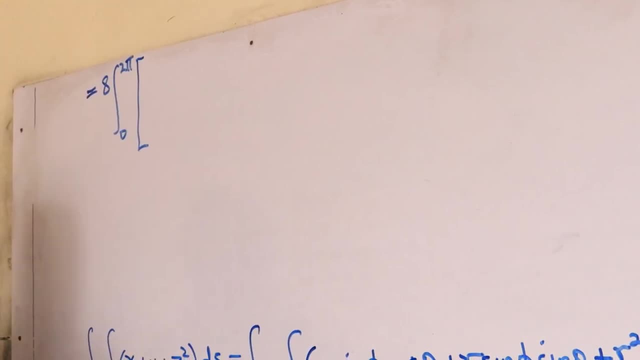 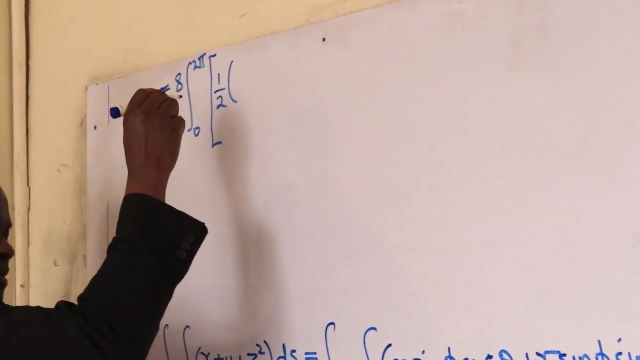 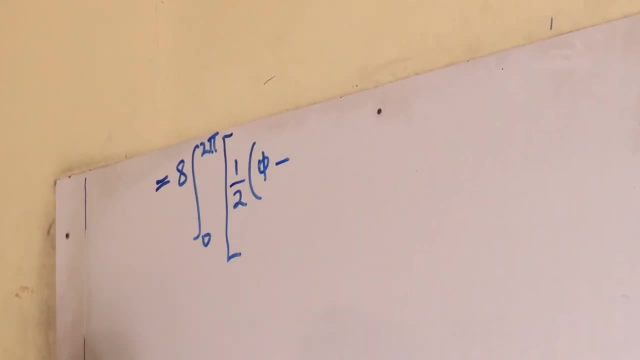 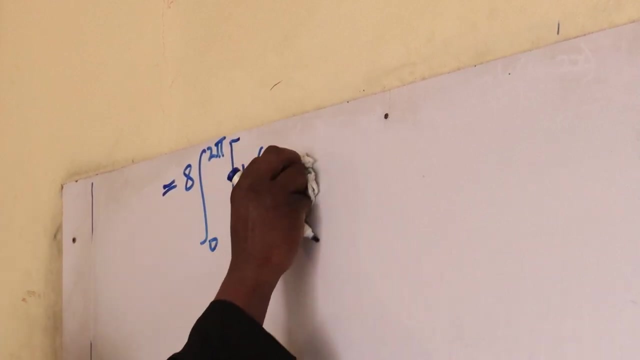 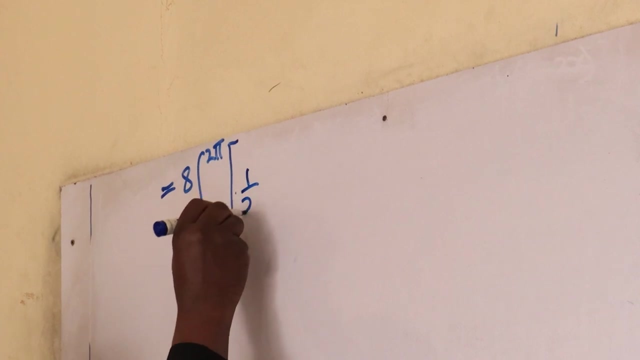 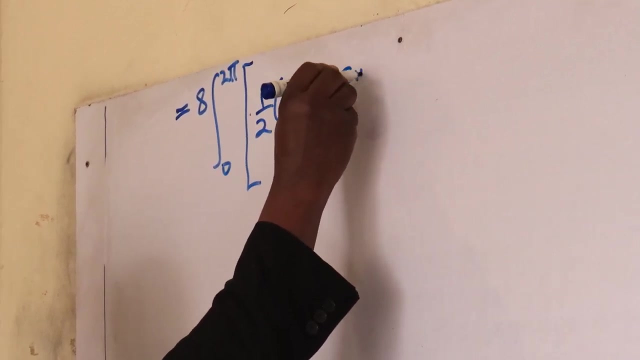 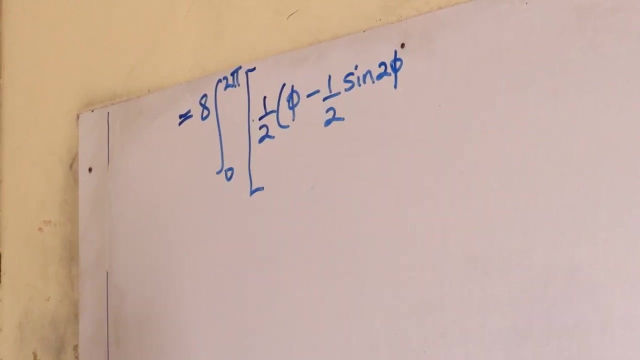 Half into 5.. Minus Minus, We have a half into phi We have a half into phi Minus a half sine Minus a half sine Sine 2 phi Sine 2 phi Minus a half sine two phi. 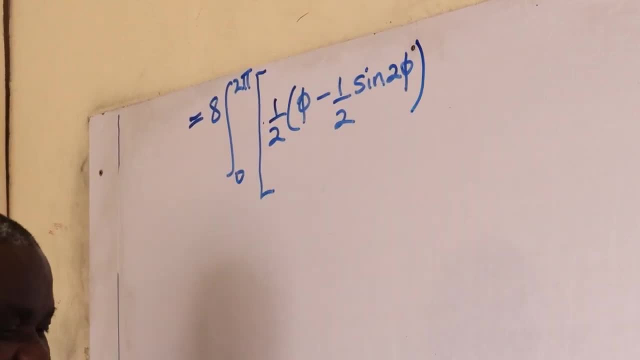 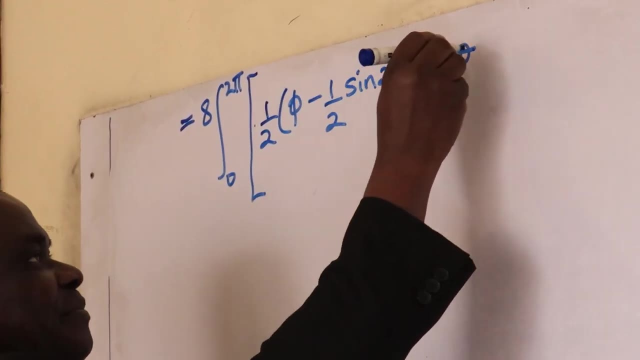 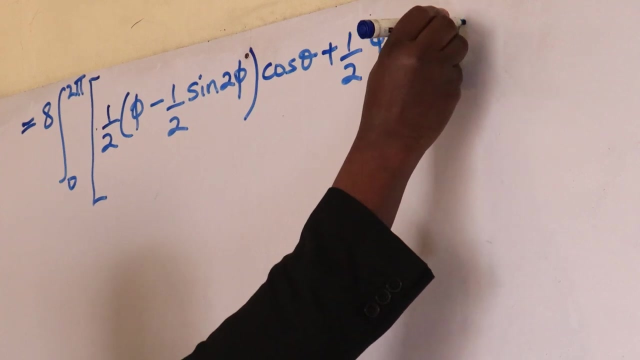 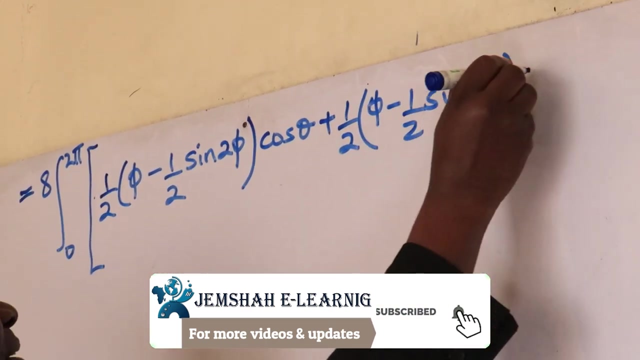 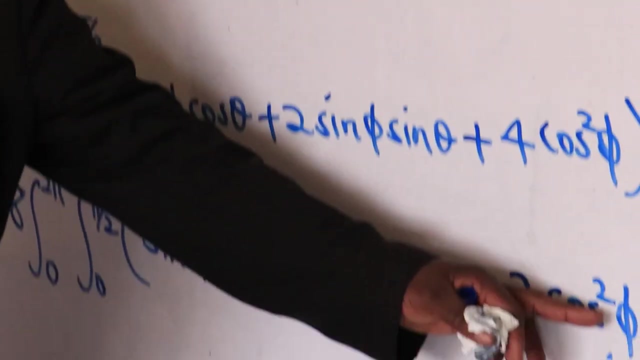 2 phi. Now, the whole of this is multiplying cos theta, plus another half n to phi, minus a half, sine 2, 2 phi. That is when you integrate sine squared, And this one is multiplying sine theta. Now, when we integrate this, since sine phi is when you integrate a cos, when 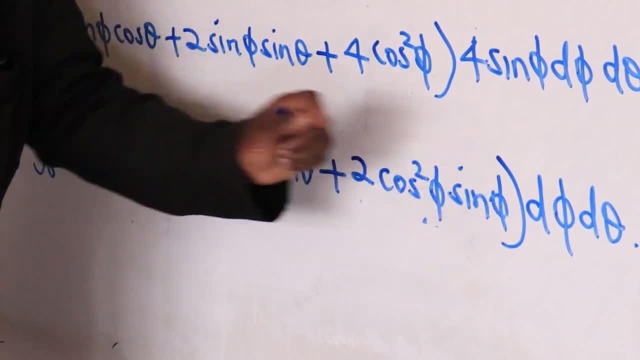 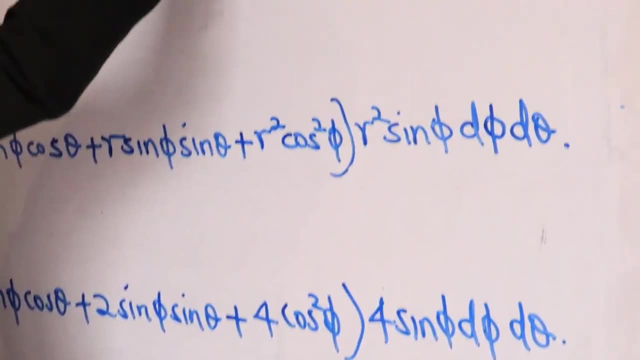 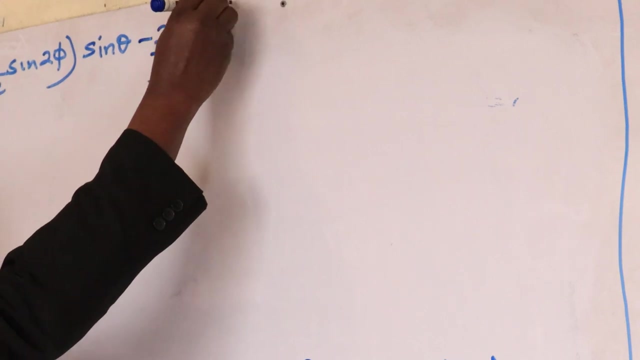 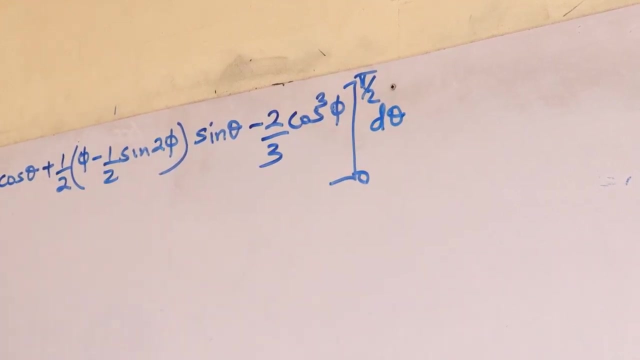 you differentiate a cos phi, you get a negative sine phi. So this one, the answer will be: minus 2 all over 3, 2 all over 3, cos cubed phi. And then we put the our limits from 0 to what Pi all over 2.. Then we remain with the d d theta which 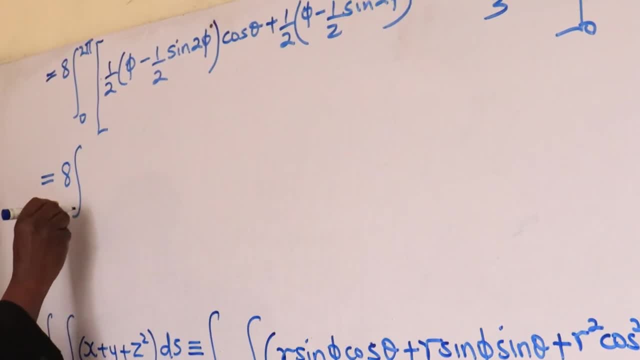 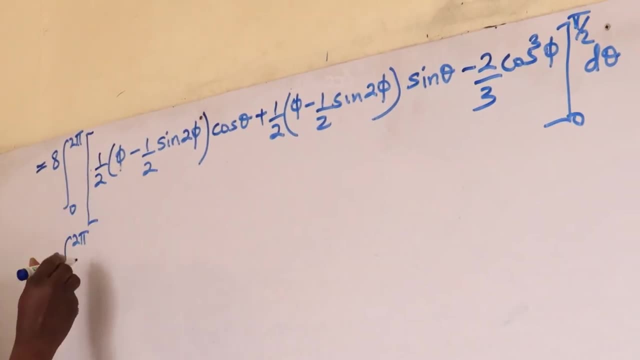 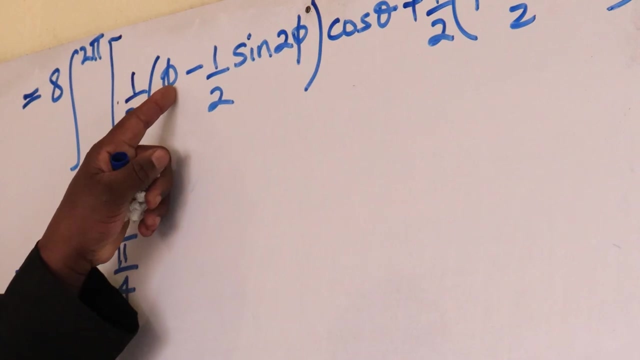 will be equal to 8, the integral from 0 to 2 pi. We are inserting our limits. When we put pi all over 2 here we will get pi all over 4, pi all over 4.. Pi all over 2 times. 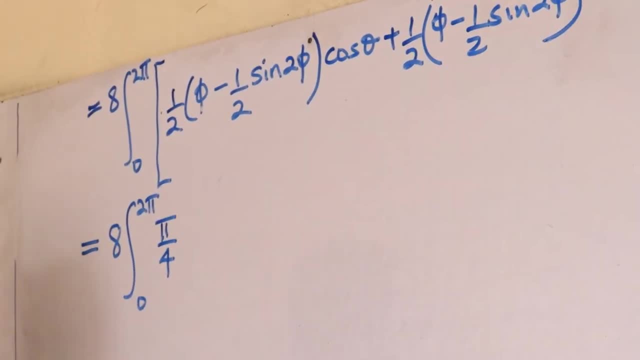 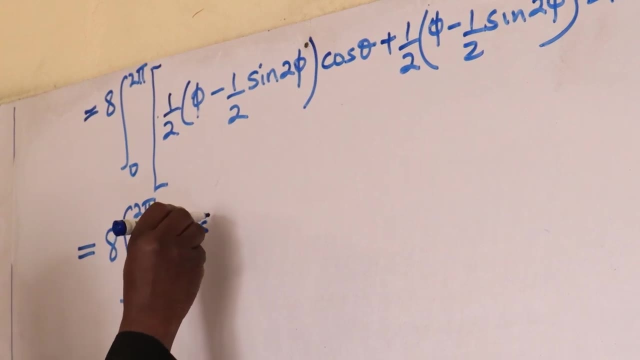 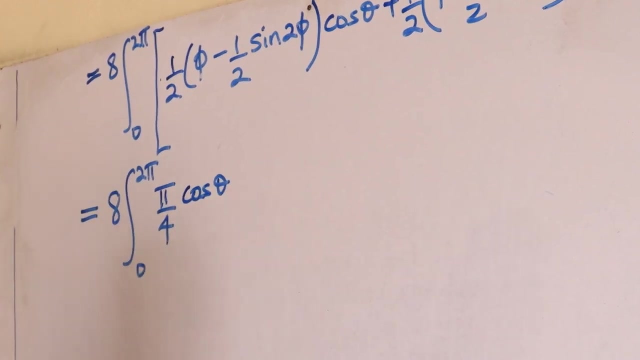 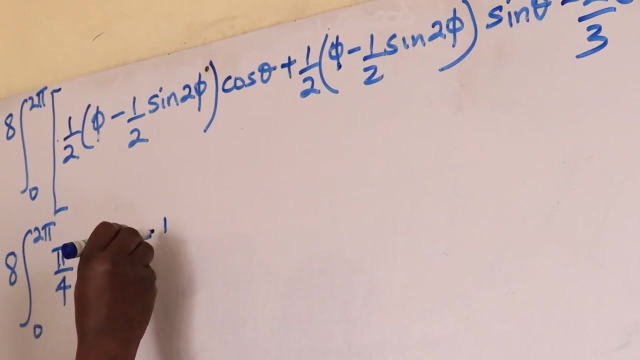 a half will be pi all over 4.. Now if you put pi all over 2 here, that one will be 0. So we'll just be remaining with cos theta There A quarter pi multiplying cos theta. Here you insert that pi all over 2. here It will also be plus a quarter pi, but going. 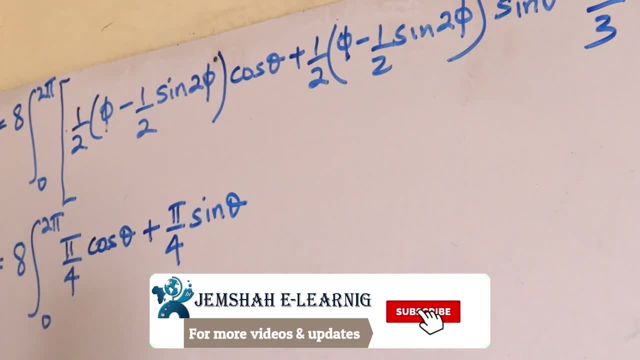 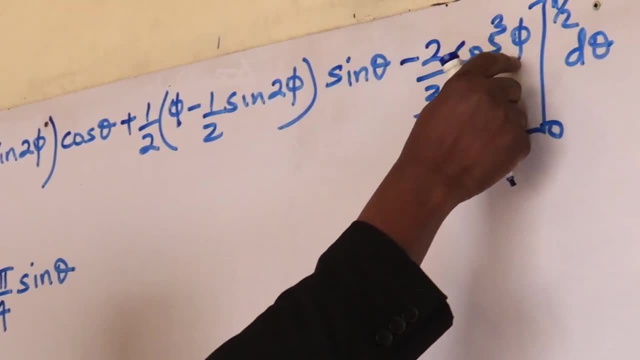 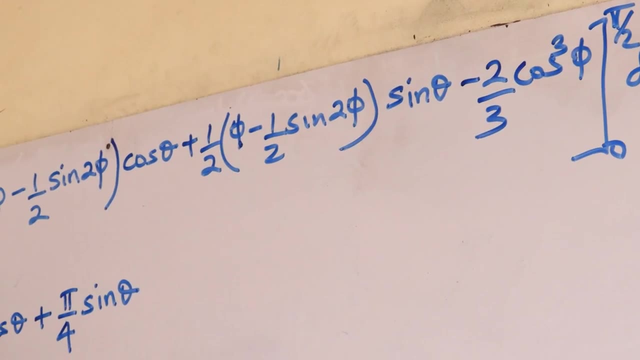 with the sine theta Subtitles by the Amaraorg community, Because the other one will do what. The other one will go to 0. Cos pi all over 2 is known to be 0. So if that one is 0, that is gone. Now we proceed, now We are inputting now. 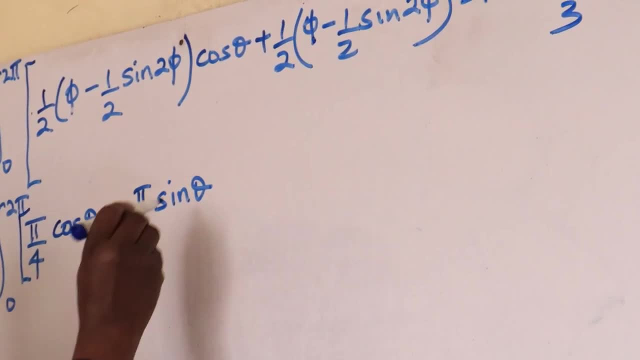 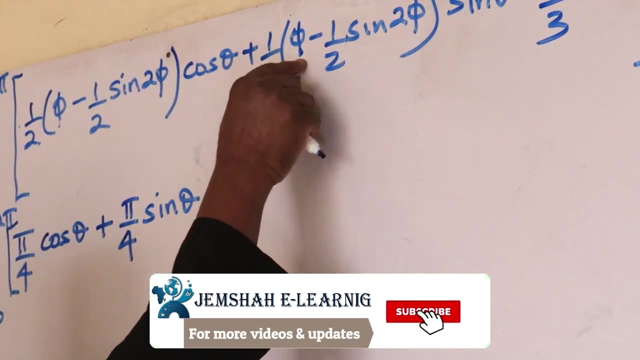 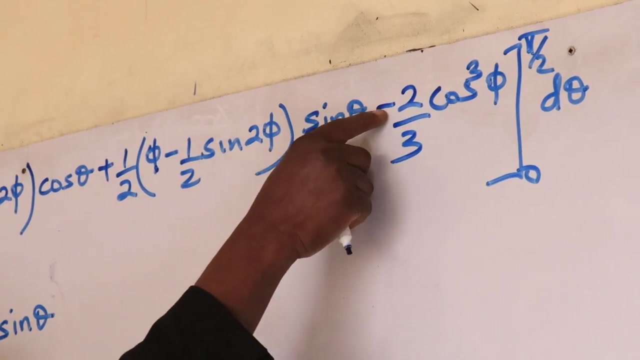 the lower limit, Lower limit, lower limit: When you input 0 here, that will be 0, 0.. So that one is 0, 0, 0.. This one, When you input 0, cos 0, is what 1.. 1. And we are inserting a lower limit, So it will. 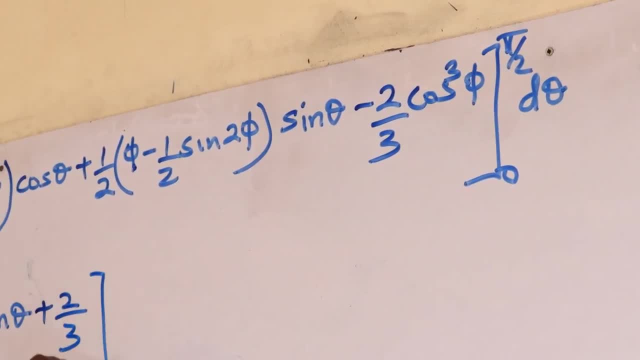 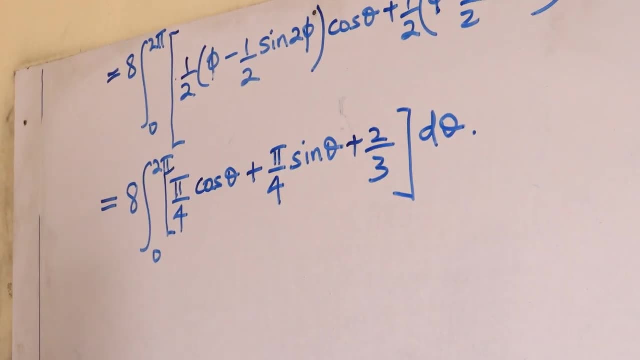 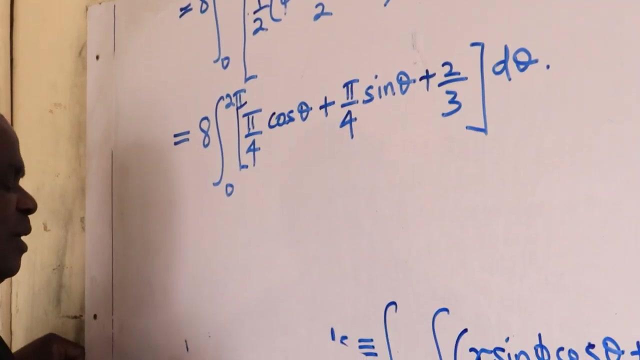 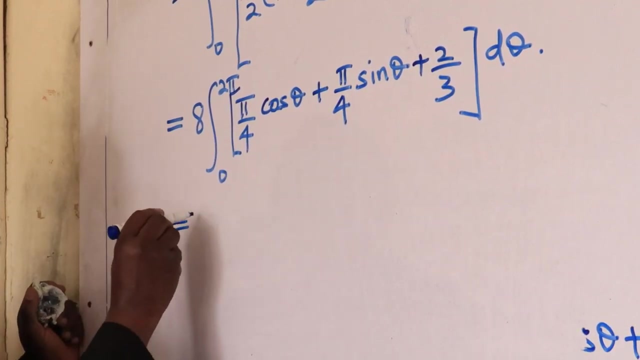 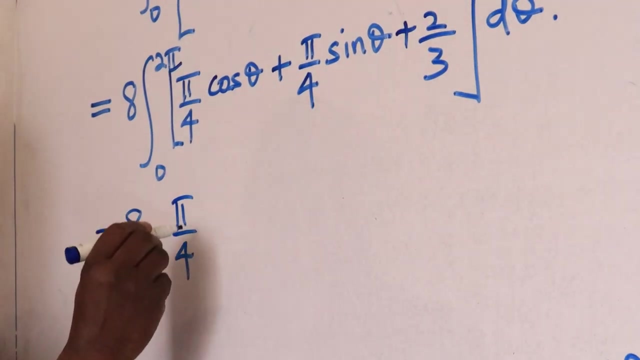 be plus what? 12 over 3.. So this is what we are supposed now to integrate with respect to theta. So from this now we are remaining with only one integral to clear this. So this will be equal to 8.. When we integrate this, we get pi all over 4.. When you integrate cos theta, you 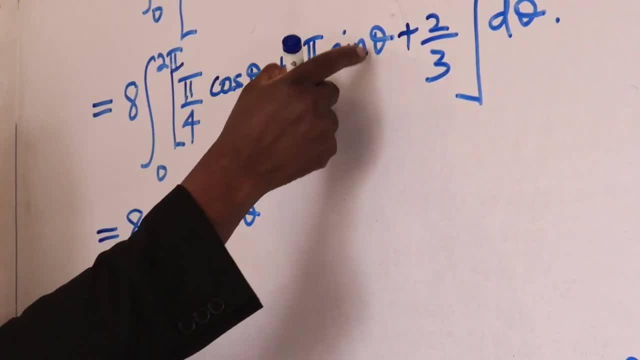 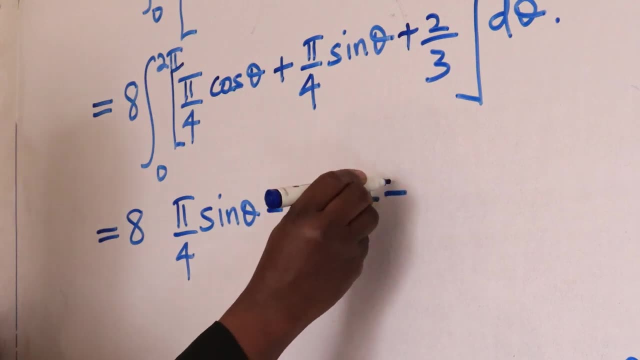 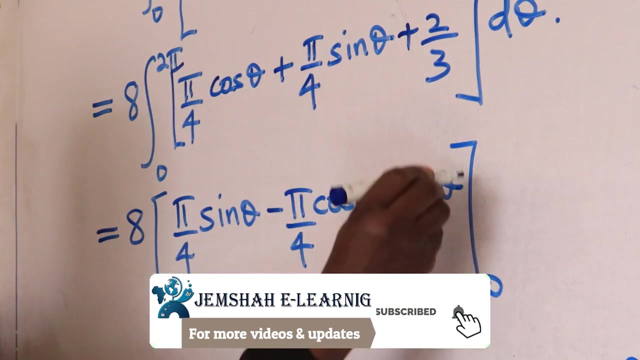 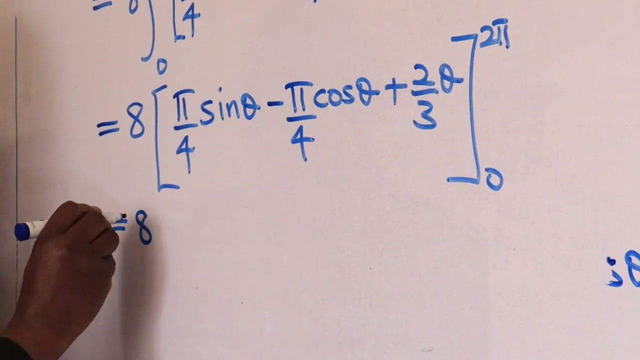 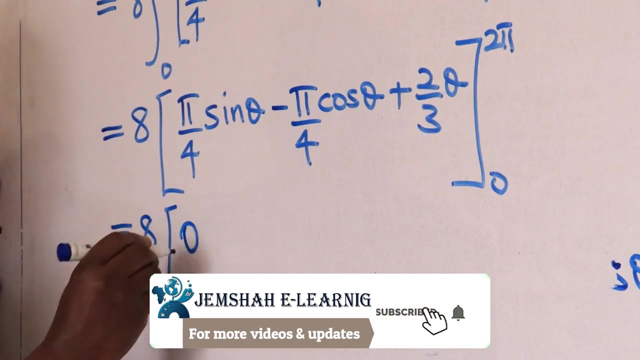 get sine theta. When you integrate sine theta you get minus cos theta, Then plus 2, all over 3 theta, And then we have our limits from 0 to 2 pi. 2 pi, Which will be equal to 8, and pi all over 4. sine 2 pi, That is 0.. Cos 2 pi is 1 minus. 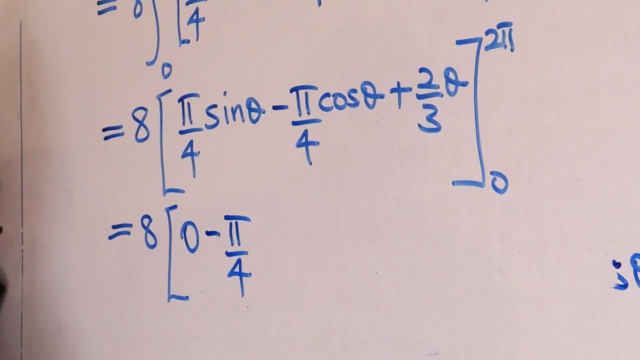 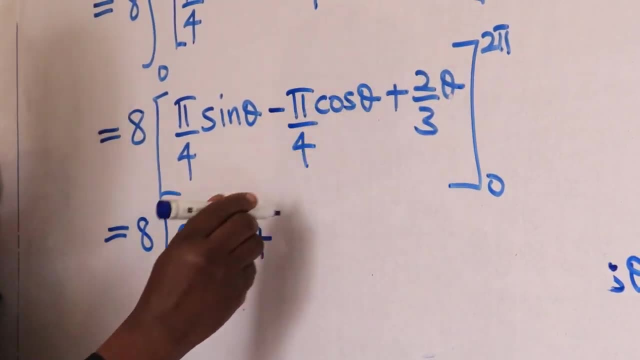 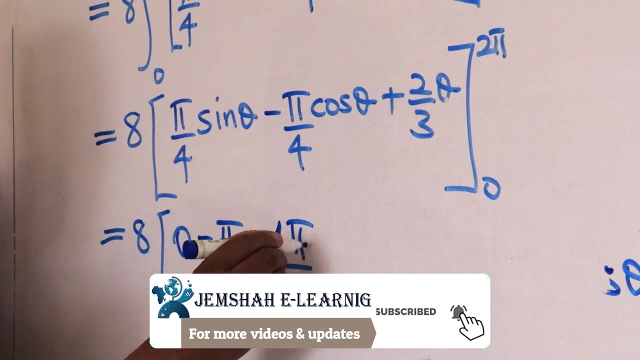 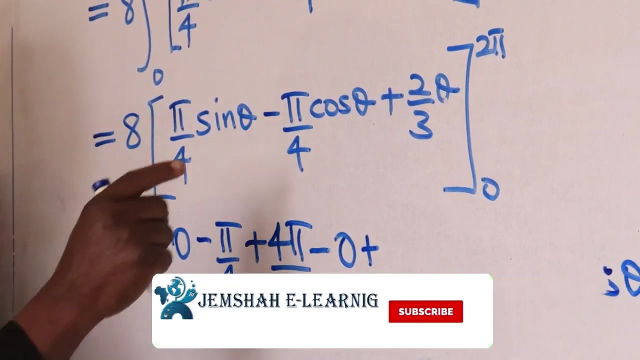 pi all over 4.. Cos 2 pi is 1.. So we say plus. When we put 2 pi here, that will be 4 pi all over 3.. And lower limit: we say minus 0,. sine 0 is 0.. Plus cos 0 is 1.. Cos 0 is 1.. So it will. 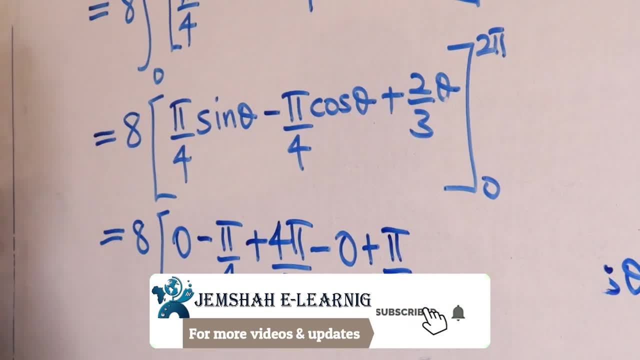 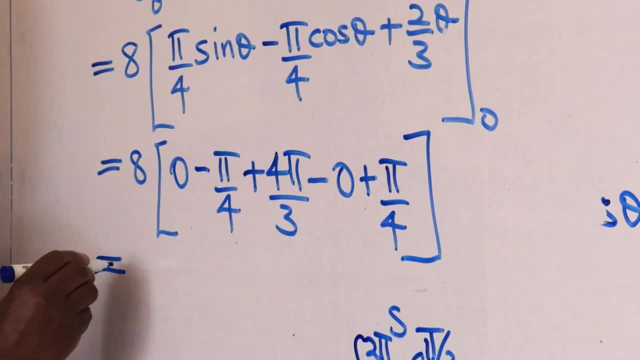 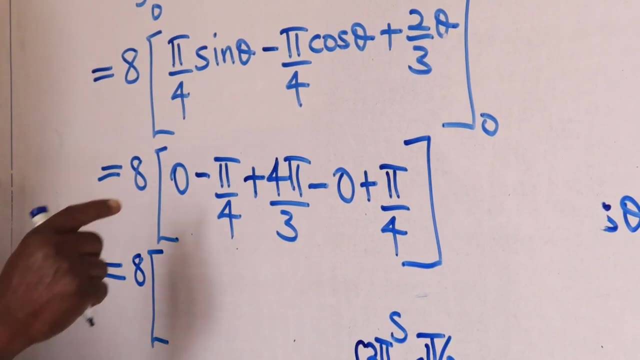 be plus pi all over 4.. And when we put 0 here it will also be 0. So the answer here will be equal to 8 and 2.. 8 and 2.. 8 and 2.. This one and that one there, This one, this will cancel, So it will remain. 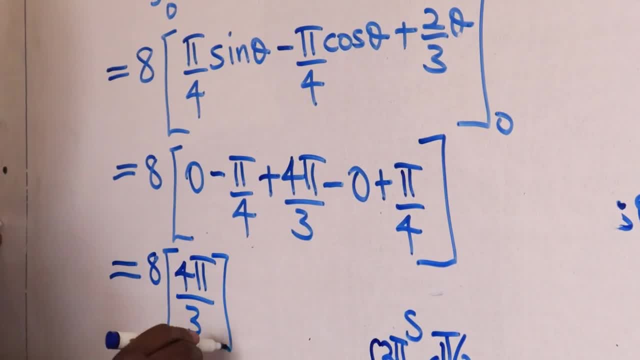 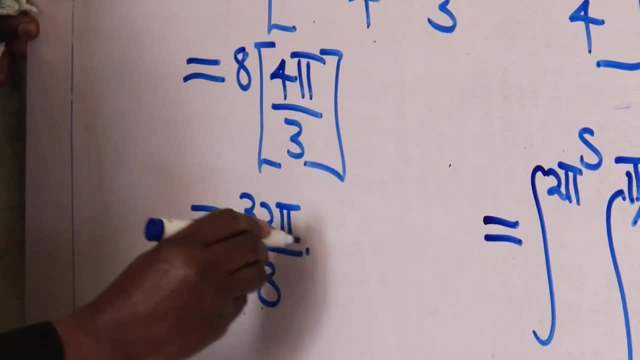 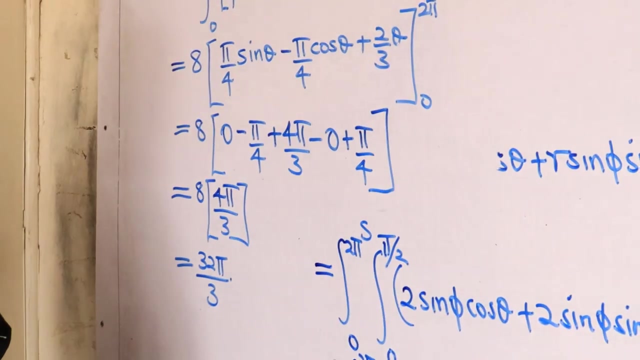 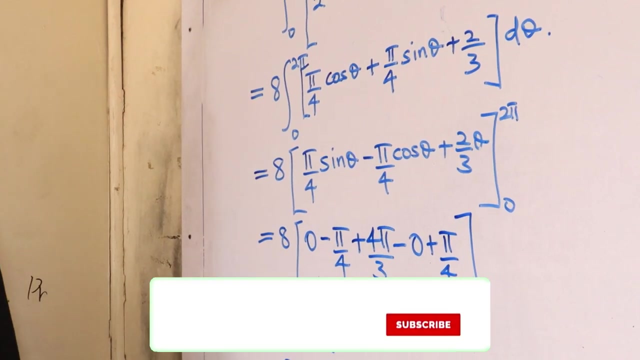 with 4 pi all over what 3.. So the answer to that surface integral will be equal to 32 pi all over 3.. And that's the final evaluation. That's the final evaluation, Lesson number 12. So the future world is, let's where you. 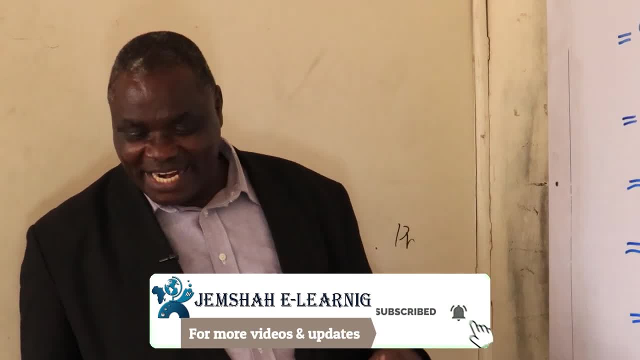 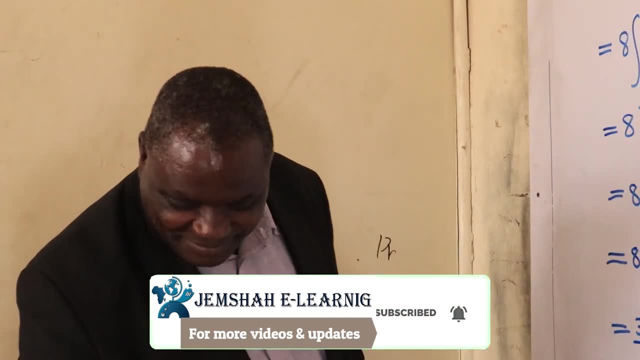 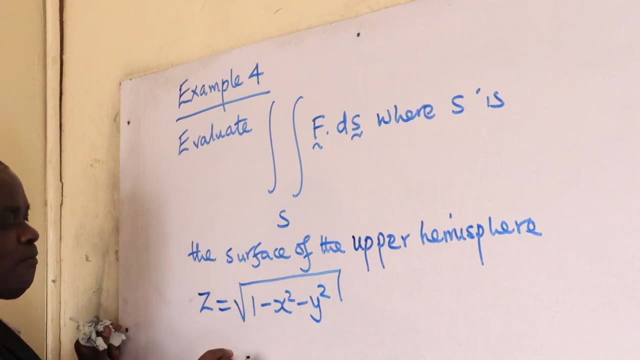 are now 2 pi cold's. Now we go into example four, which will now be a surface integral in the volume vectorial analysis. So this is a surface integral in volume vectors involving vectors 1 pi. Bye-bye, 1 pi. 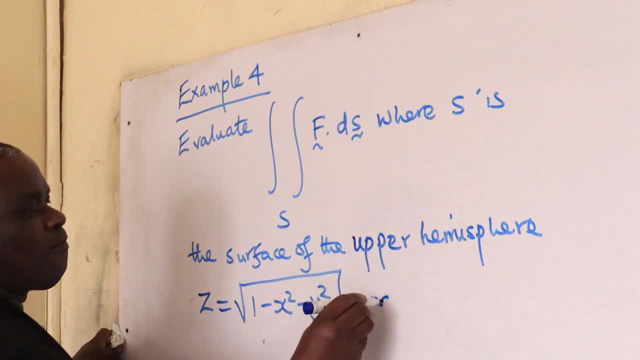 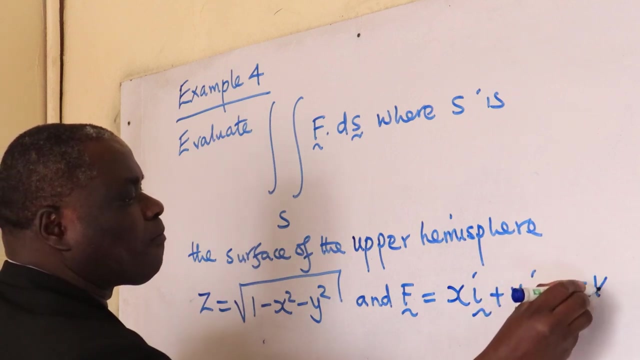 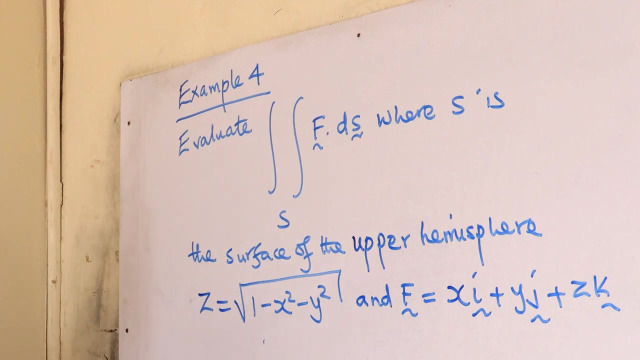 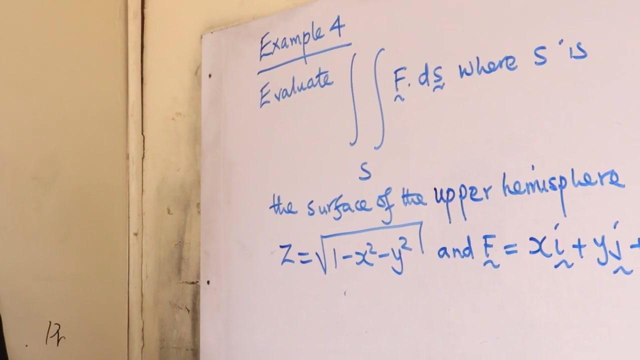 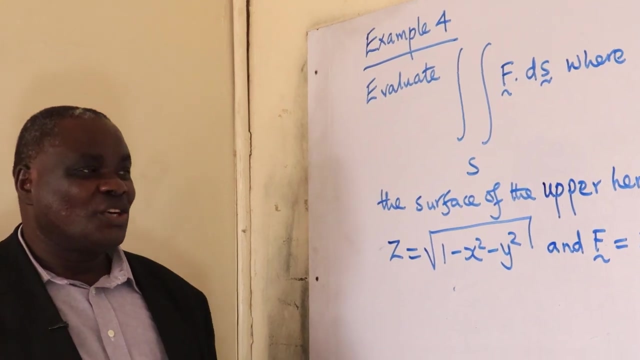 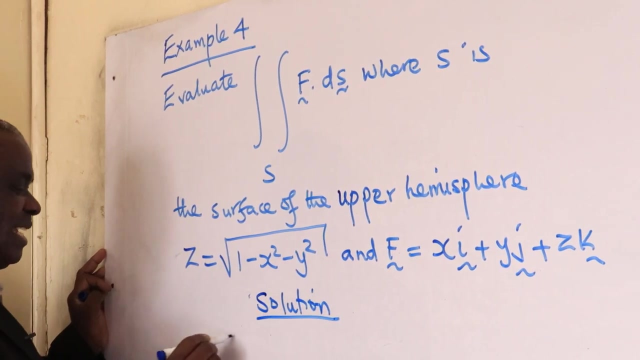 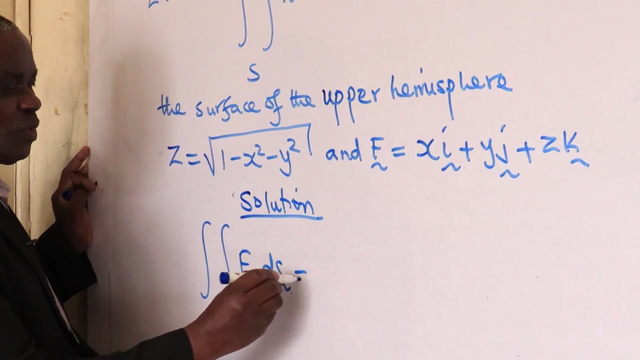 Some. we proceed now. you are now to evaluate f dot ds. this ds is a vectorial s, so in our solution we rewrite that one first. in our solution we say the double integral s, f dot ds vectorial. this one is equal to double integral for the limits from surface s. this will 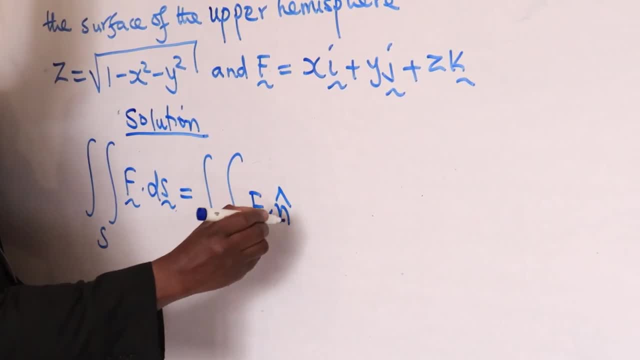 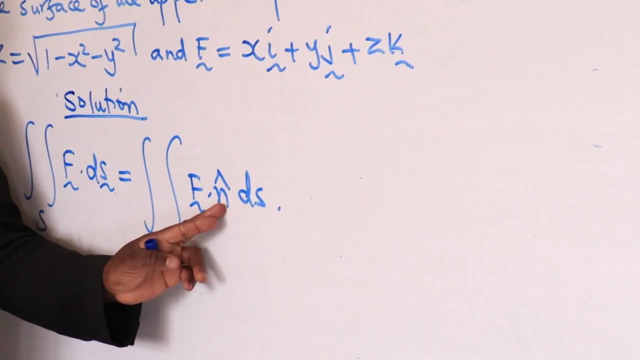 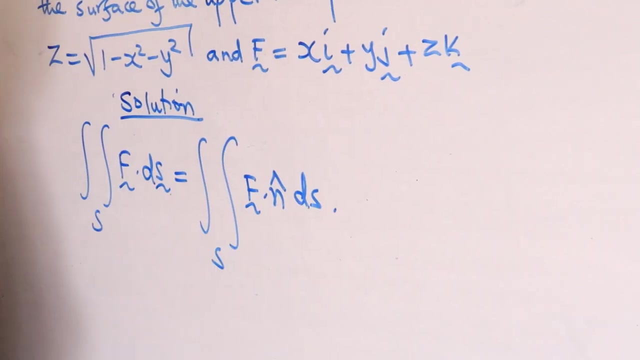 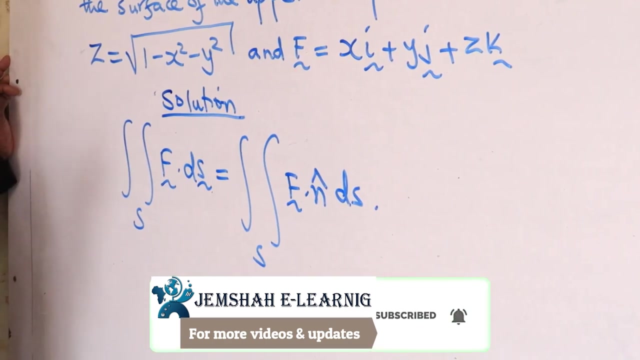 be f dot n multiplying scalar ds. so the vectorial ds is equal to the unit normal vector to that surface, multiplied by the scalar ds, by the scalar ds. now, if that is true, now that n must be a vector normal to the surface, and our surface is. 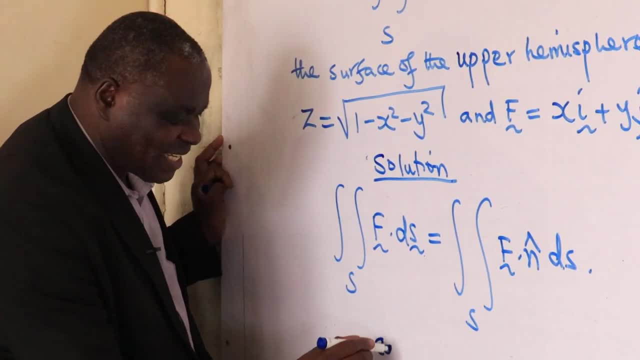 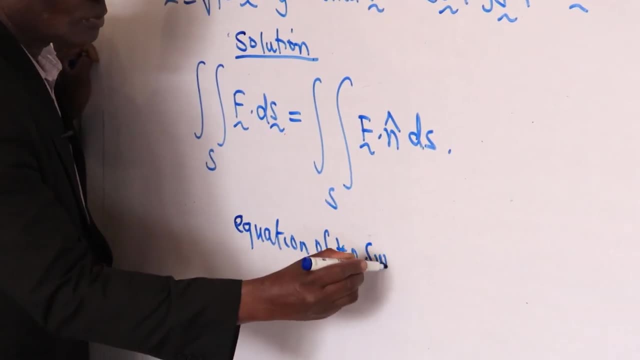 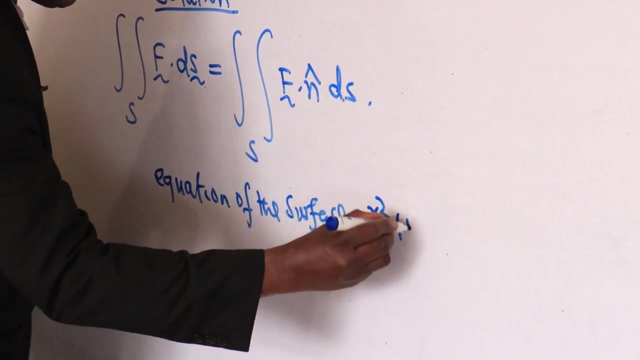 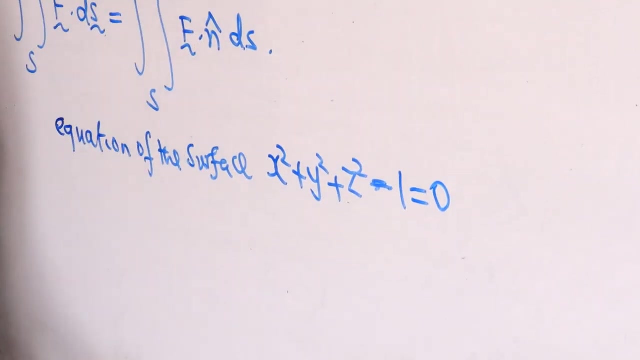 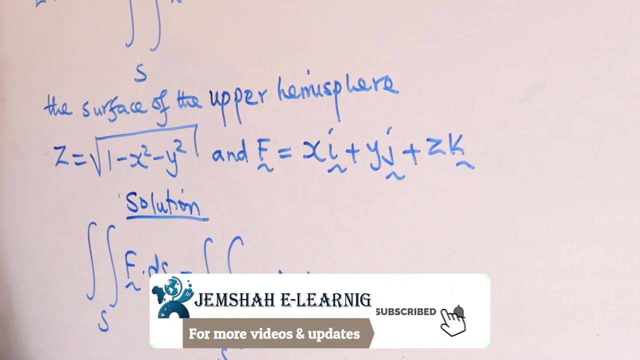 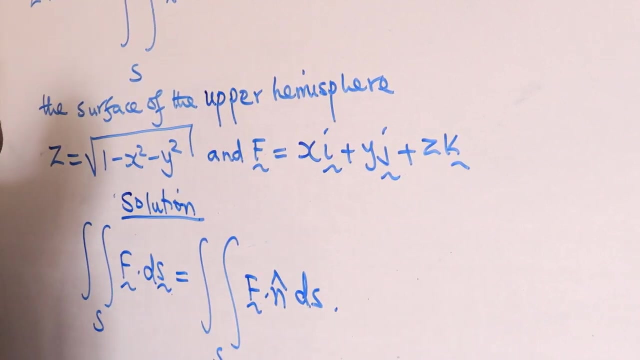 the equation of the surface is given by equation of the surface. equation of the surface is one x squared plus y squared plus z squared is equals to minus. one is equal to zero. if you prepare this, you square both sides and bring all those this side. that's what you're going to have. so we prepare what our n and this unit normal vector. 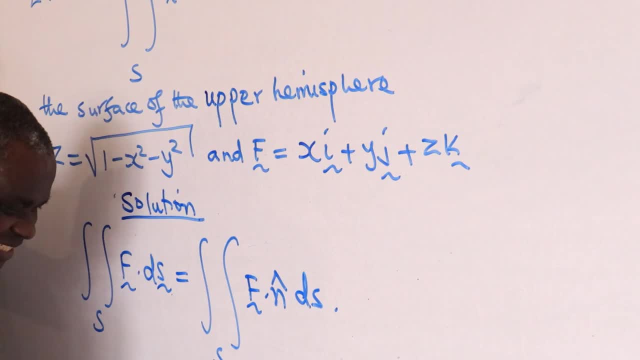 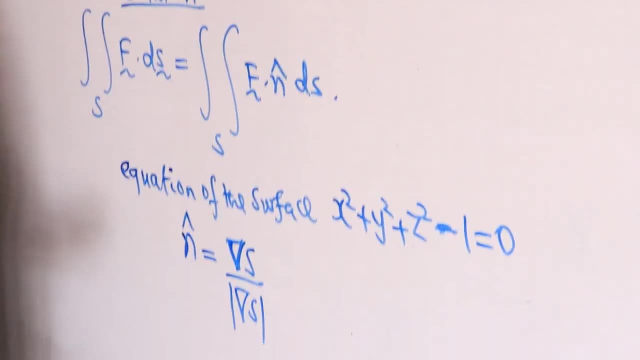 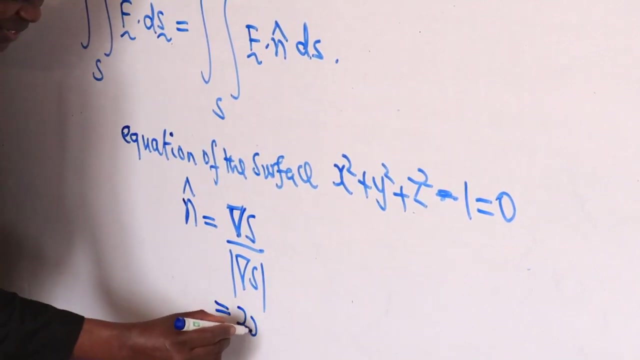 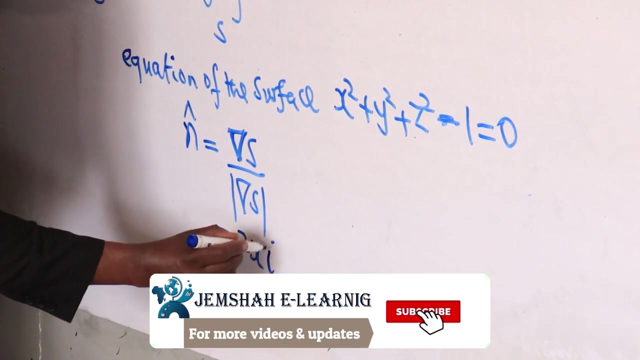 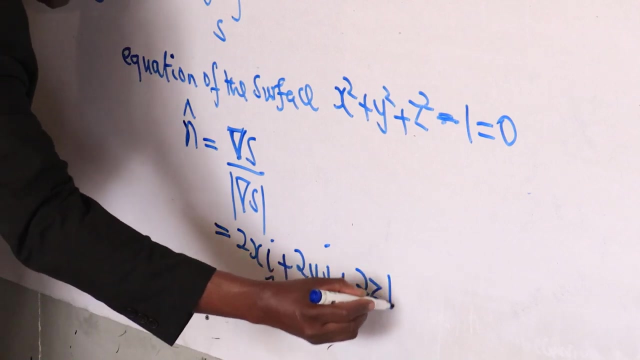 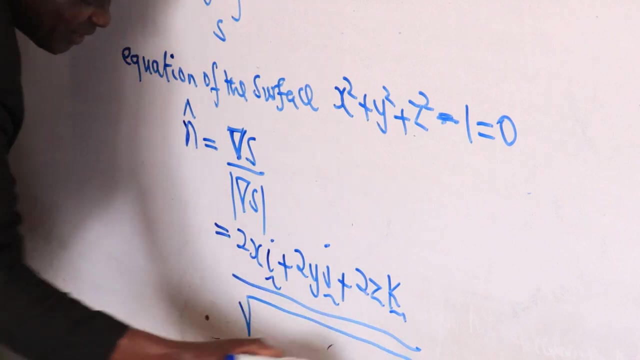 is normally equal to one grad s all over grad s my magnitude, grad s all over grad s, my magnitude, which in our case now will be equal to: when you differentiate this with respect to x, you get two x, two x. now two x goes with the i, i, plus now two y goes with the j, j plus now two z goes with k j, all over the square root of all, over the square root of four x squared plus four y squared, plus four z squared. 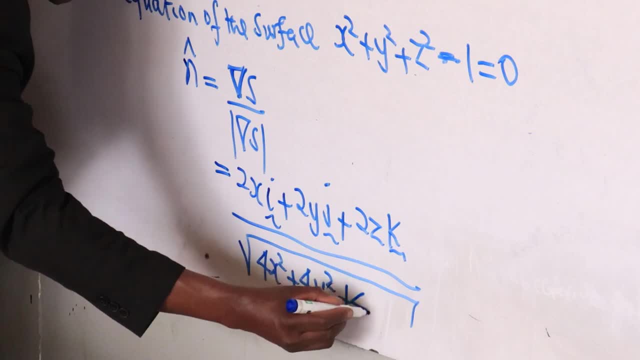 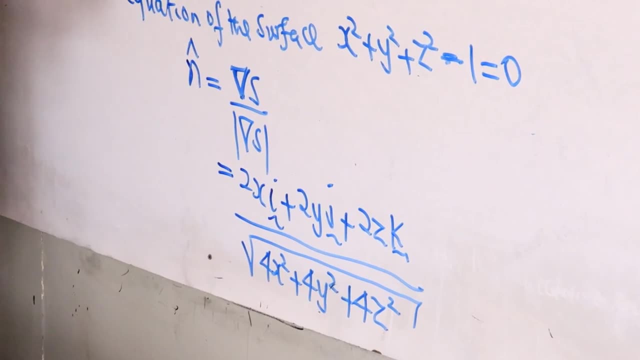 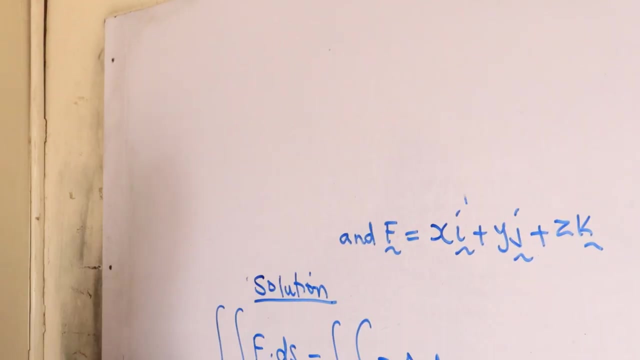 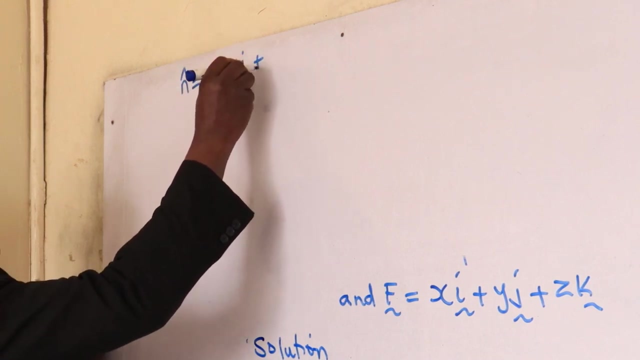 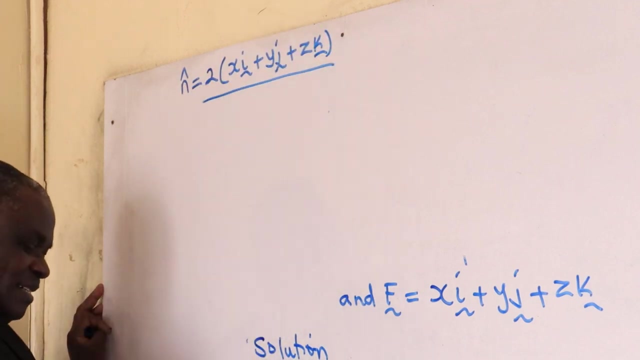 half four, half killed, which simplifies to our end, will be Tutu And will be he called. Tutu is common Right. Two hour Tt will be x, i plus y, j plus z, k, all of them root of 4, root of 4, we know, is also 2, then we have 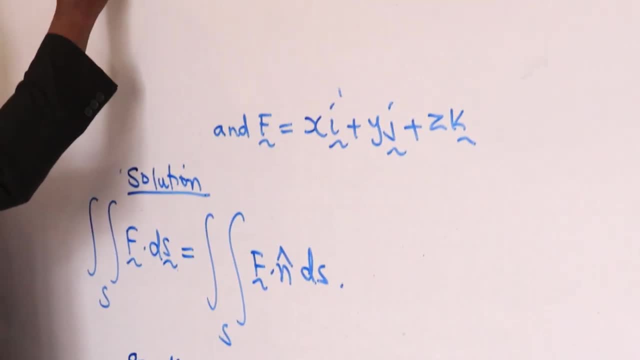 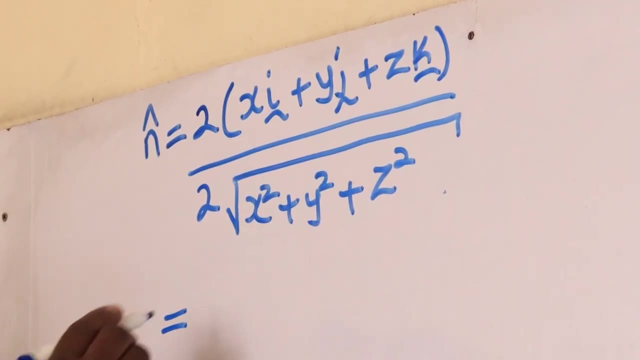 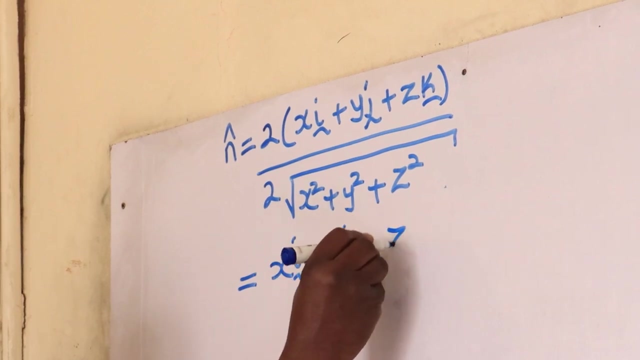 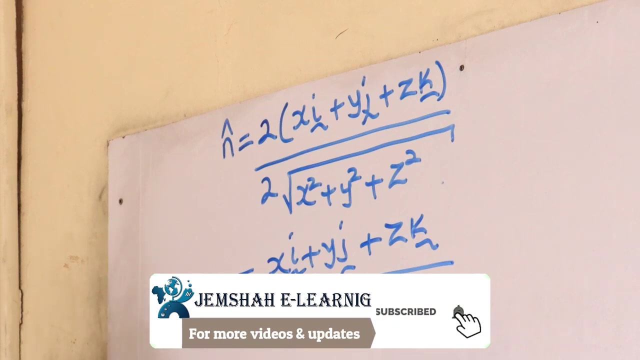 square root here, what is remaining, which is x squared plus y squared plus z squared, What we know very well on that surface, on that surface, on that surface, x squared plus y squared plus z squared is a constant and it is equal to 1.. So we are going to divide. 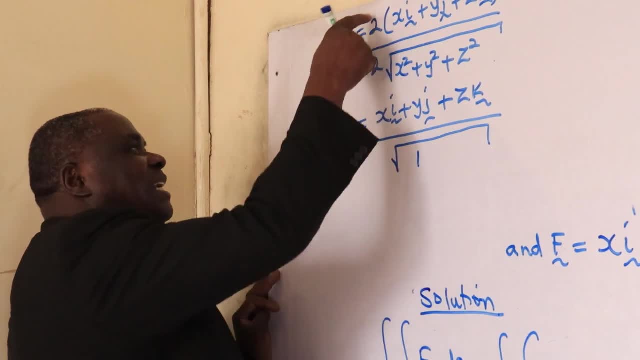 by root of what? 1, since this one has cancelled that. So whatever we have now will just be x, i plus y, j plus z, k, all of them root of 4, root of 4, we know, is also 2, then we have: 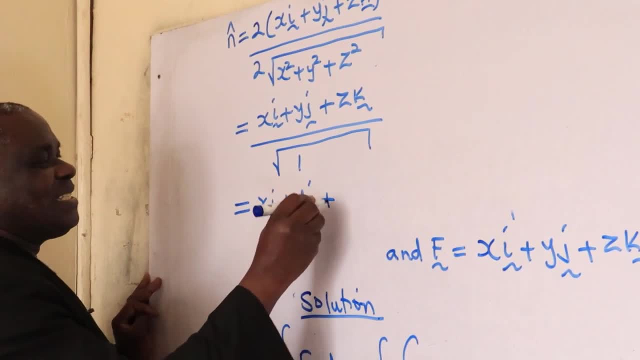 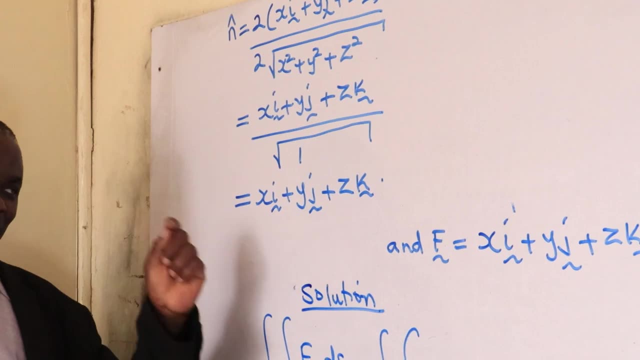 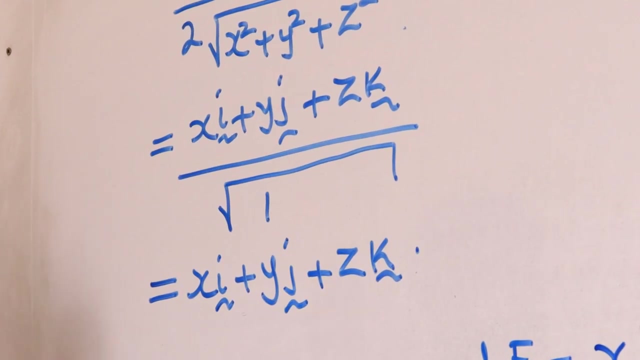 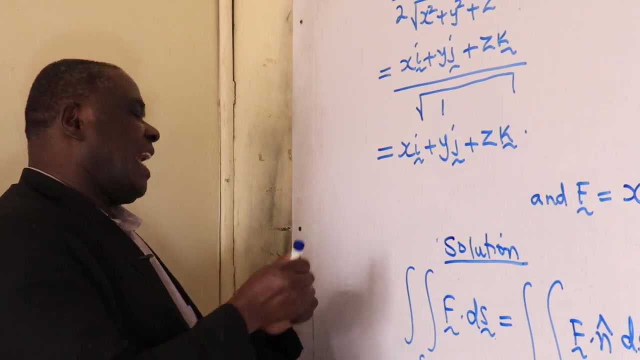 square root x, i plus y, j plus z, k, that is being our world unit normal vector to that particular surface of our world, our hemisphere, and it is an outward normal vector. Now we would like to prepare f dot n, because it is appearing: 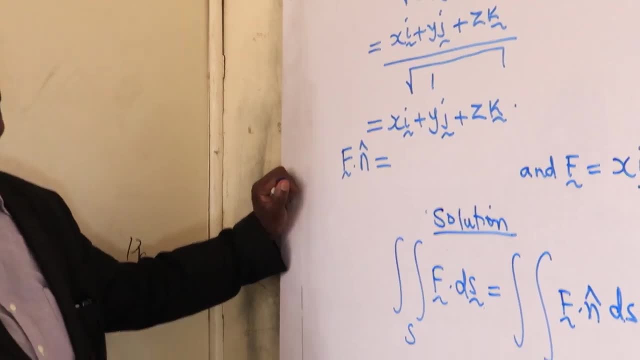 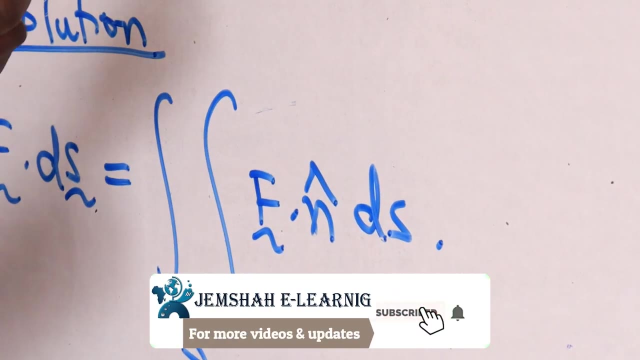 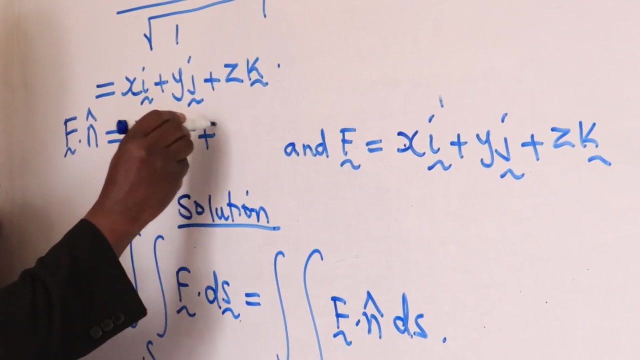 in our analysis, where we have our surface integral F dot n, We are dotting F and a n, So F dot n. this x will multiply that x, so it will be x squared plus y squared plus z squared. That will be our F dot. what Dot n? 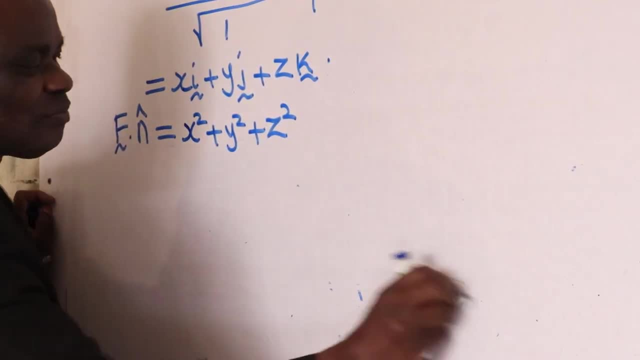 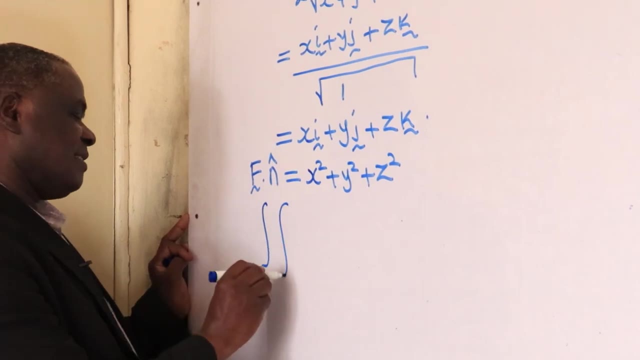 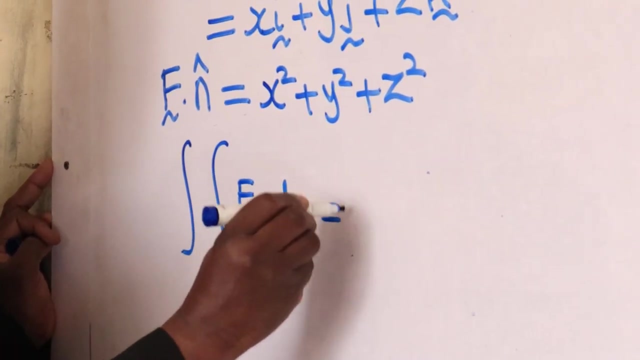 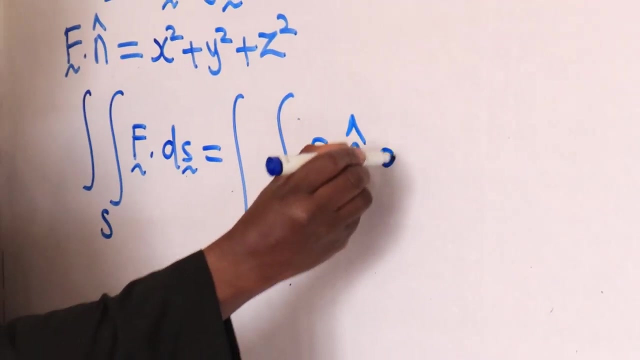 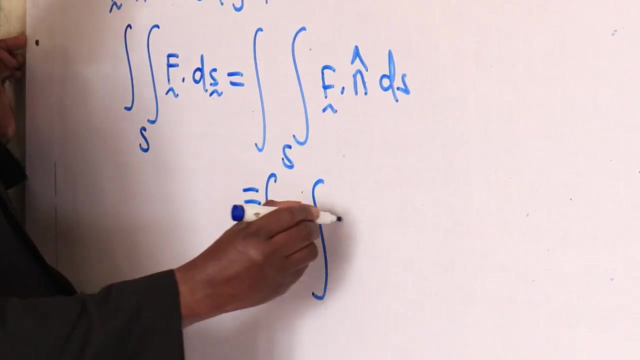 That will be our F dot n. Finally, finally, we now evaluate so this: as F dot ds now, which will be equal to integral, as F dot n ds will be equal to what A double integral F dot n is x squared plus y squared plus z squared. 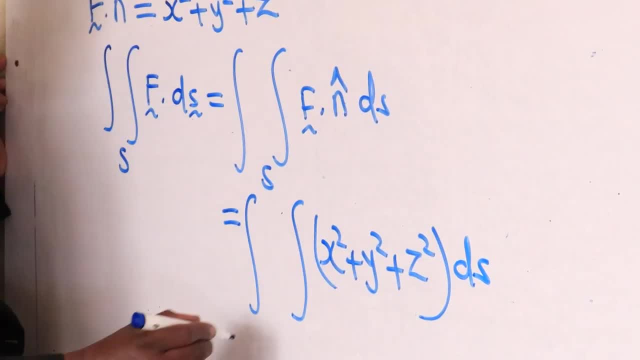 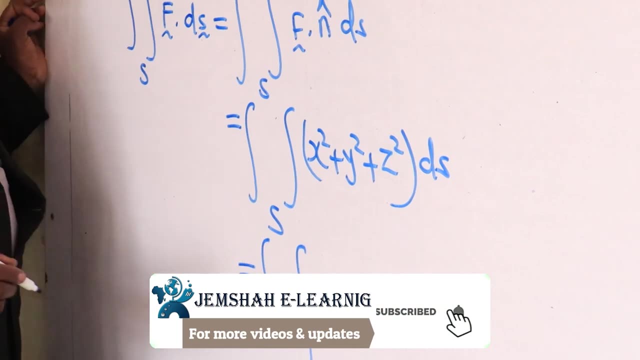 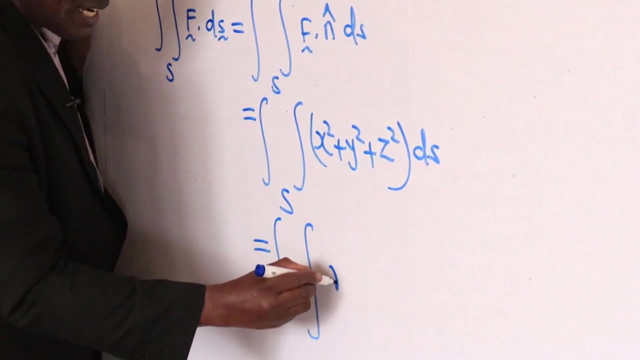 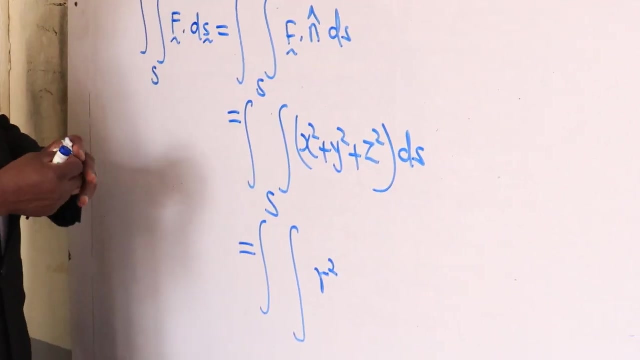 Then we say ds. Then we have here: since we are on a spherical surface, we change everything into spherical coordinates. x squared plus y squared plus z squared in spherical coordinates is equal to r squared. Can I say it is equal to r squared. So 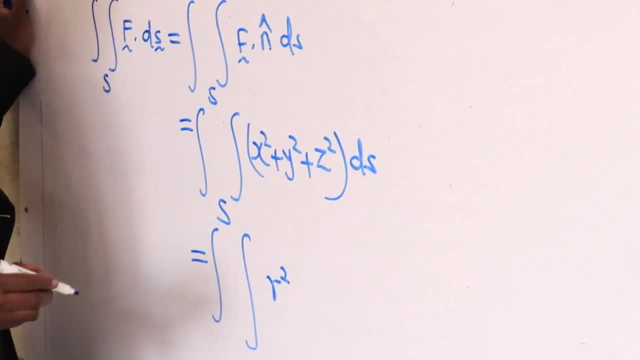 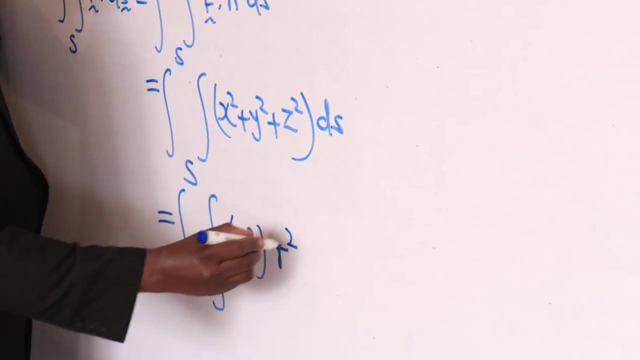 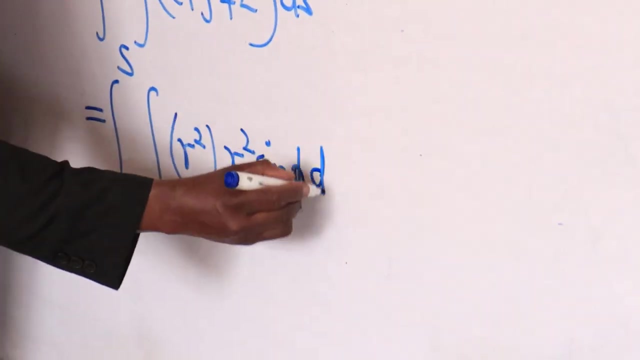 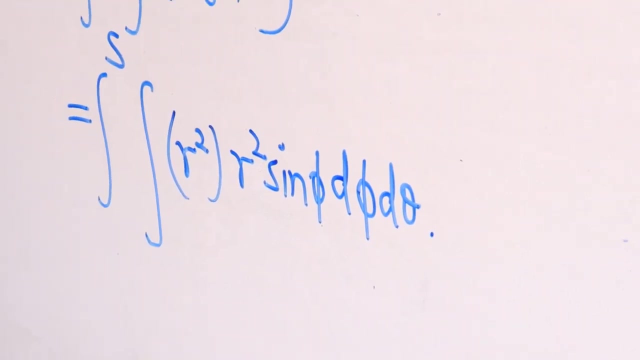 ds now will be equal to ds now will be equal to what r squared sine phi, sine phi d phi, d theta, d theta. Now, on that hemisphere we say phi is changing from zero to pi element. phi is changing from zero to pi element. phi is changing from zero to pi element. 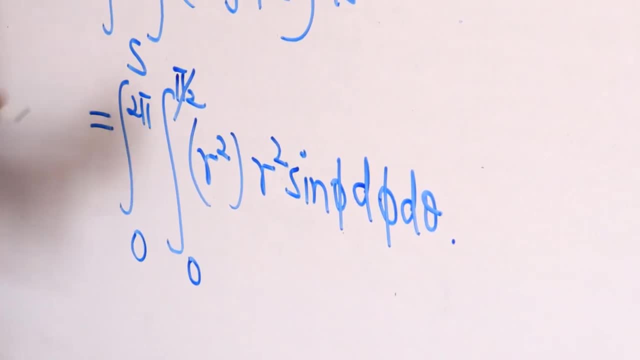 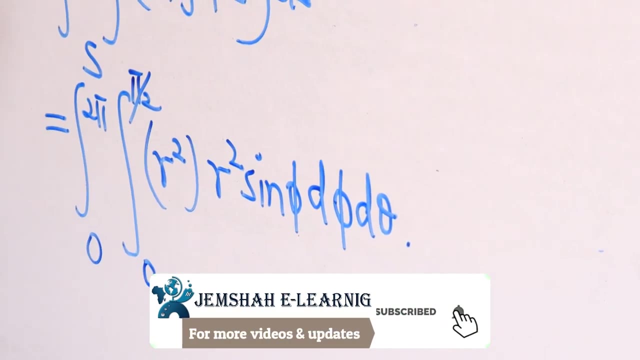 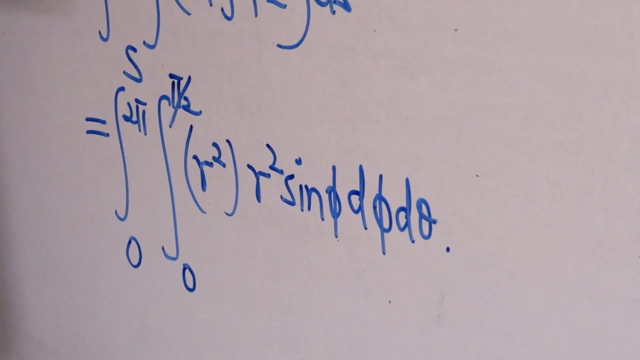 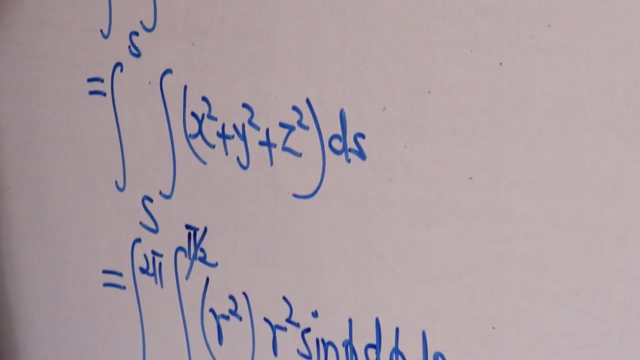 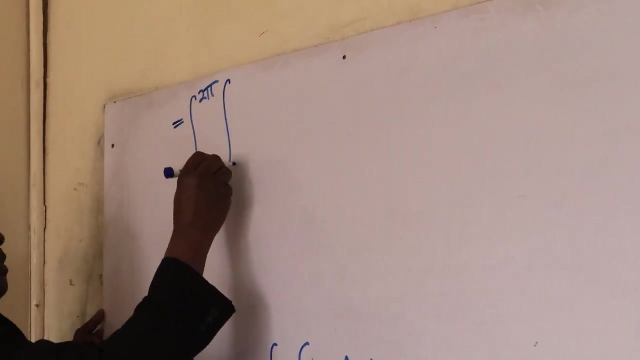 And theta changing from zero to two pi. Two pi, So the r. there is just what A constant Which simplifies to what It simplifies: to zero to two pi. zero to two pi, 0 to pi. all over 2. 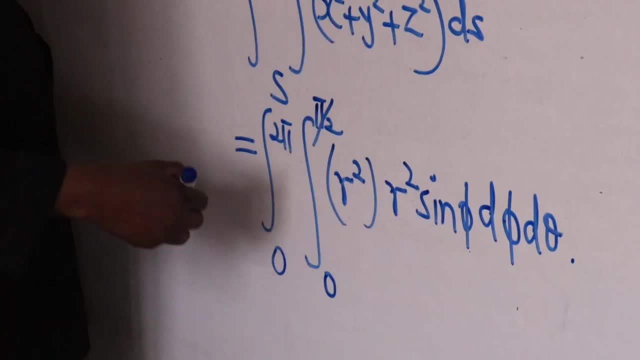 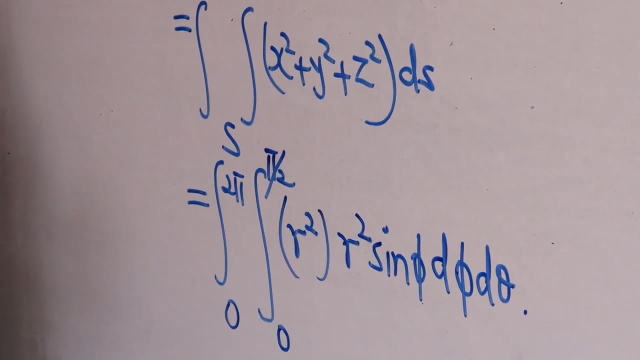 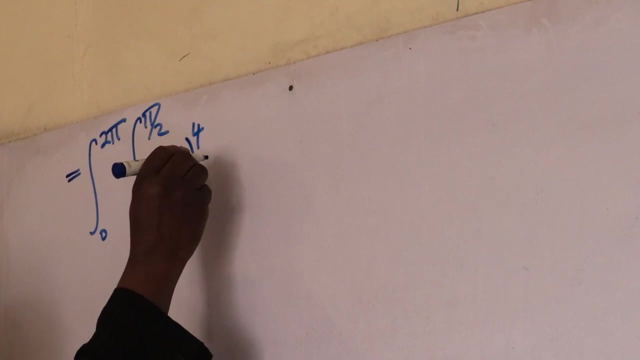 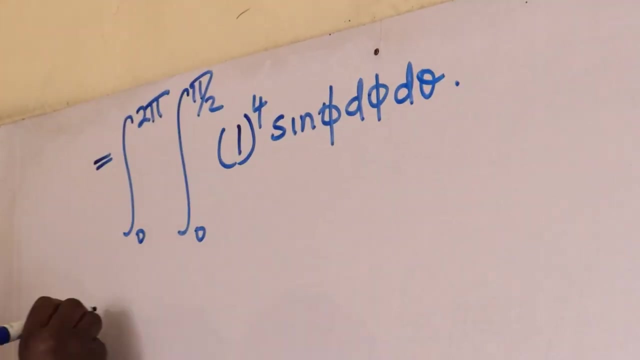 then this one times, that's r power 4, and r was a constant, and in that particular sphere it is a sphere of radius. 1, 1 power 4 is just what: 1 so sine phi d phi d theta, which will be equal to 0 to 2 pi. 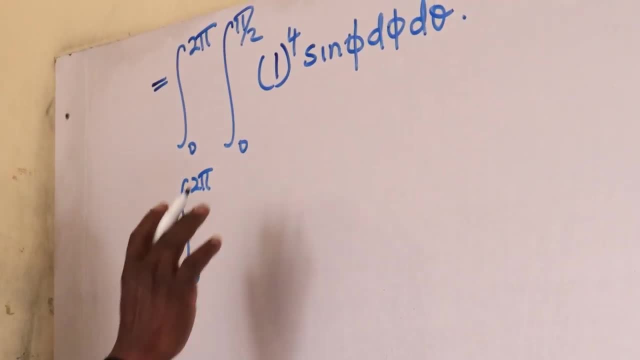 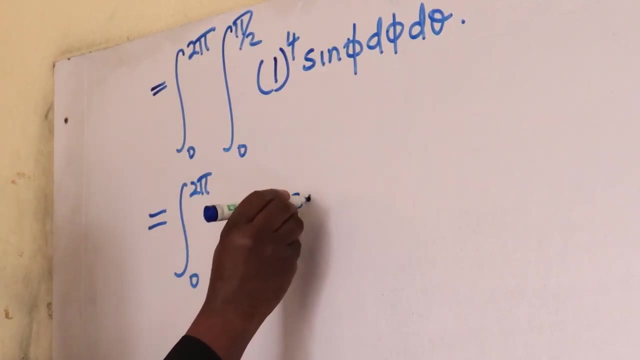 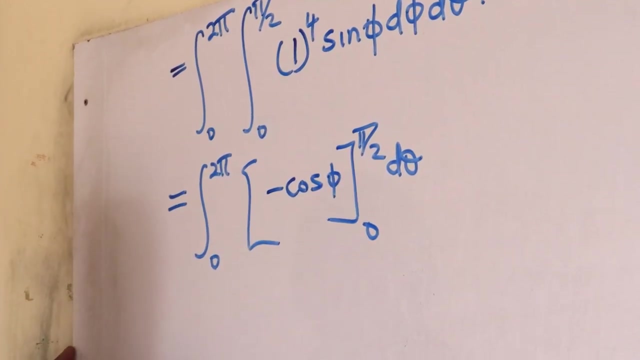 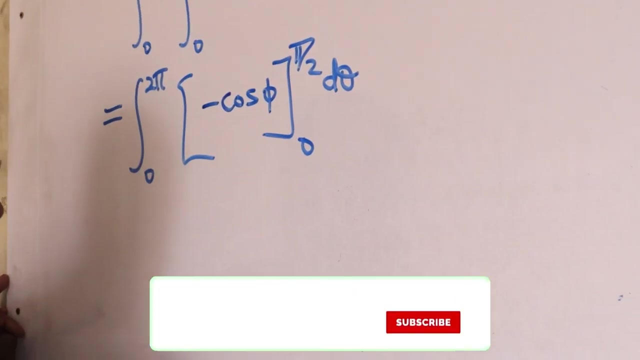 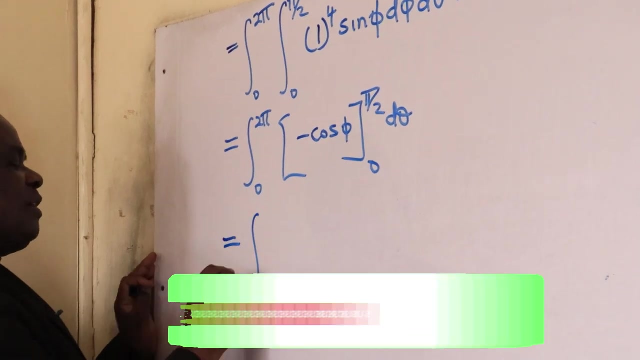 0 to 2 pi. this one will then give us what integral of that we get, minus cos phi we input from 0 to pi, all over 2 d theta d theta, which will be equal to 0 to 2 pi, which will be equal to 0 to 2 pi. 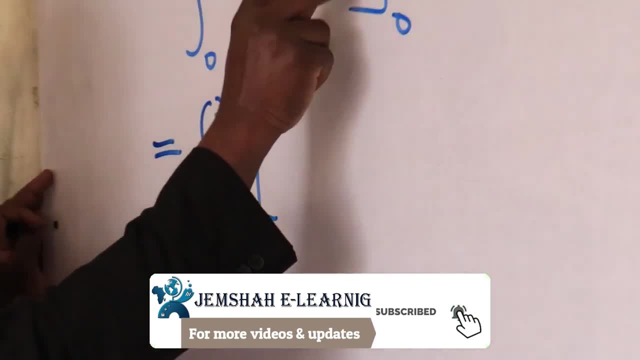 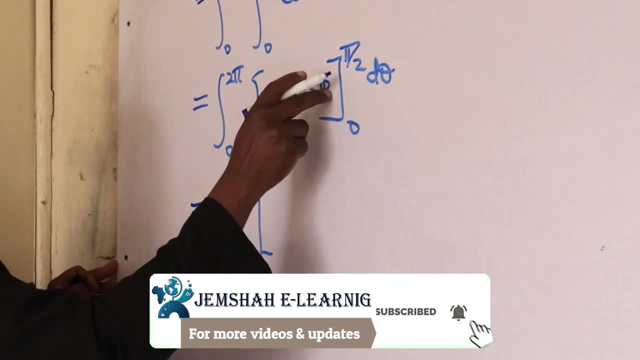 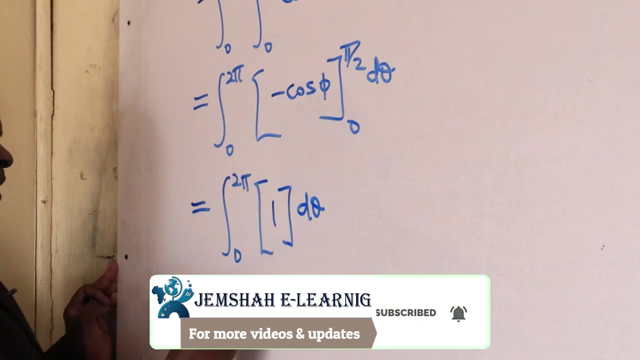 this one. we insert this one. here we get minus cos phi all over 2. cos phi all over 2 is 0, cos 0 is 1. so here is just 1 d theta, which is equal to theta 0 to 2 pi. it just gives us 2 pi, 2 pi. 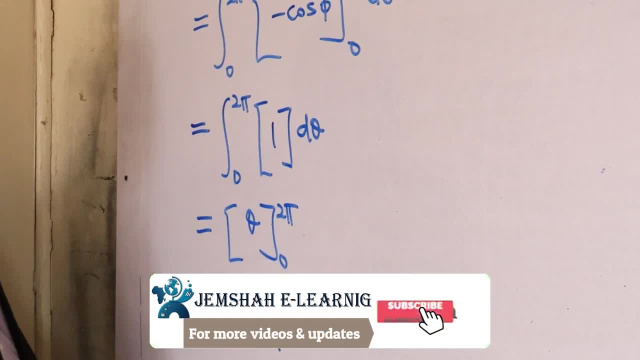 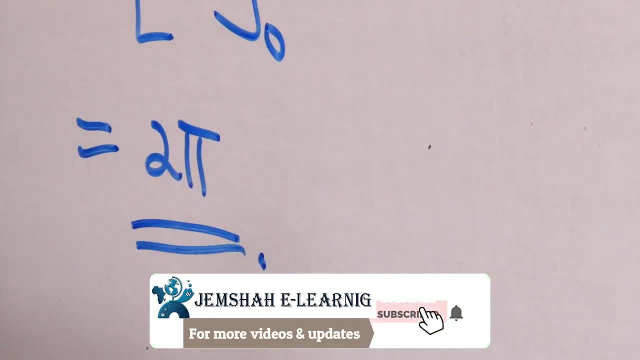 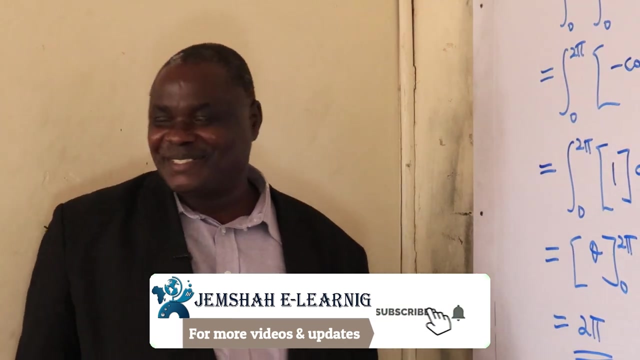 and that's now the end of that working. that's the evaluation of that surface integral. we are going to stop there. our next stop will be the line integrals. so when we meet next time, we will be doing line integrals. we will be doing line integrals.